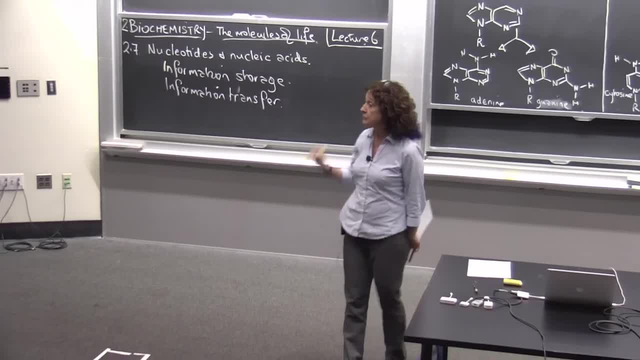 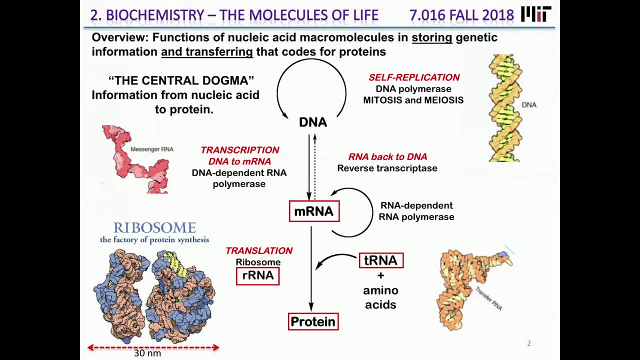 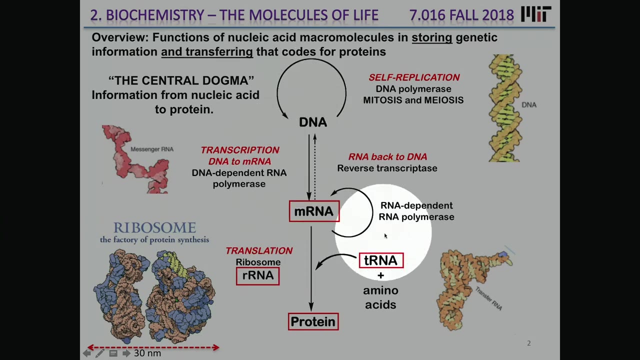 it's a nanosecond scale structure that one can program to do different things, And I think you might enjoy that. So, in this picture of the components and what's known as the central dogma, that is how DNA is converted into messenger RNA which, through the help, 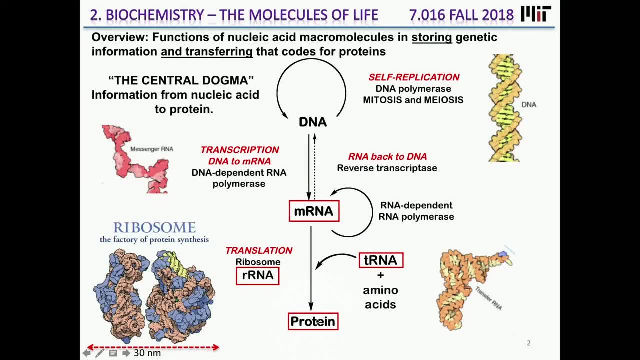 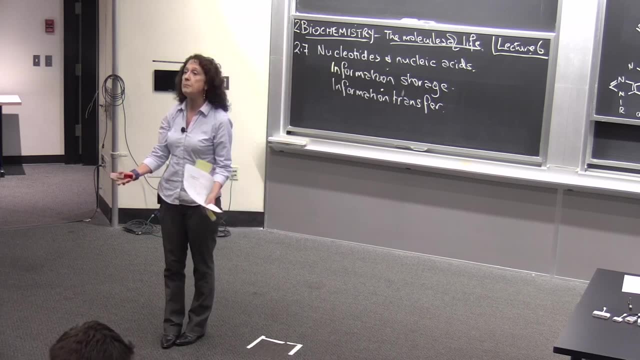 of transfer RNA and ribosomal RNA, we get proteins. The key elements on this slide are RNA, messenger RNA, ribosomal RNA and transfer RNA, And those are all made up of nucleotides being brought together into polymers that are nucleic acids. 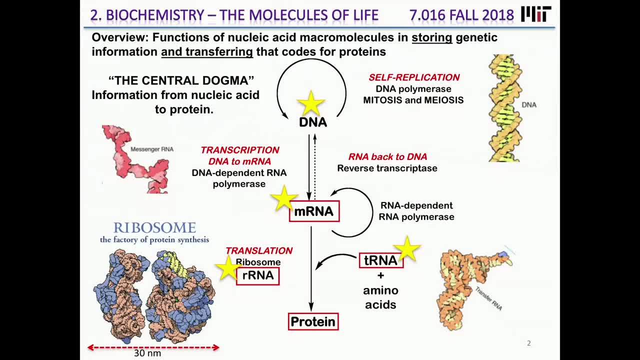 So obviously we really need to crack the structures of these and understand how the structure informs function. Remember, we did that for proteins, We've done that for phospholipids, We thought about it very briefly for carbohydrates. But the thing that I really want to stress, 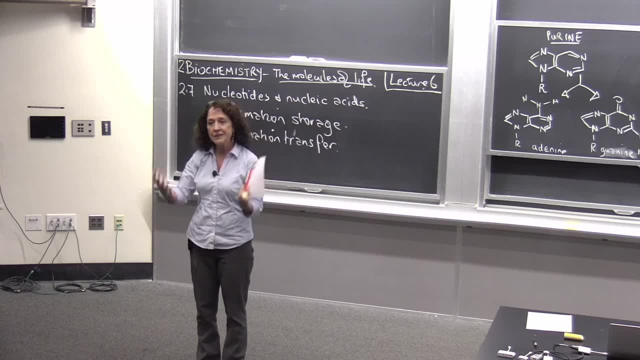 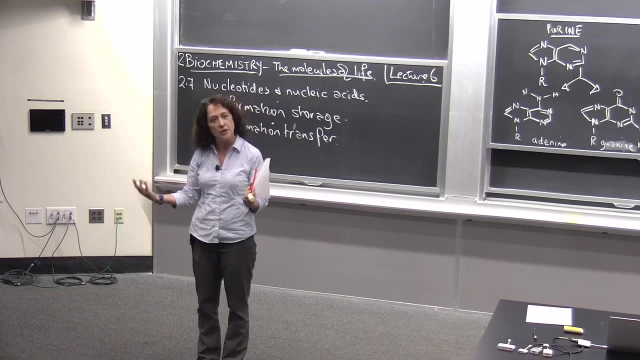 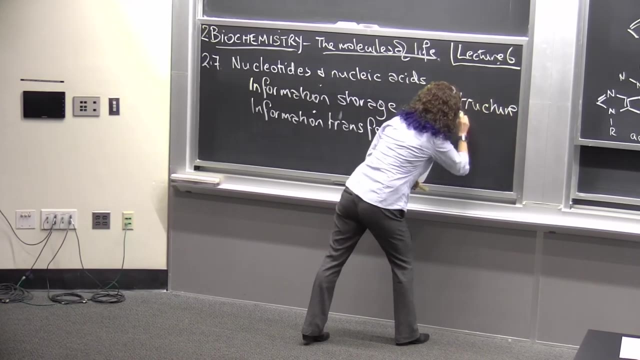 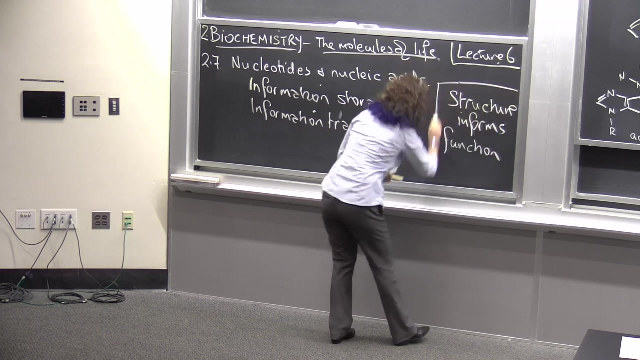 I'm going to stress to you with the fourth of these macromolecules is looking at how the last component of the biomolecules structure really informs function, And it's really cool to think about how it's done. So how is that chemical molecular structure something that we can understand from the 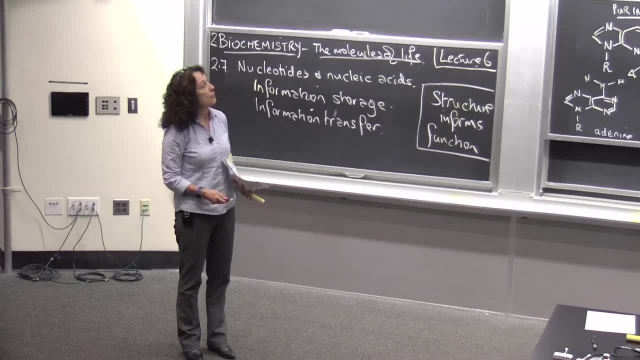 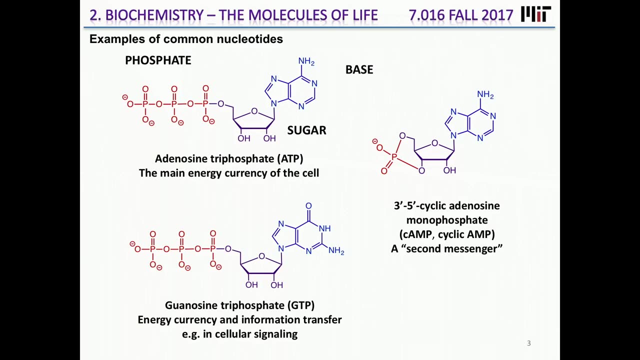 the perspective of function. OK, So what we need to do first of all is think about what nucleotides are and understand their structure so that we can move forward to understand how they come together to build these macromolecules that are so pivotal and essential in life for programming. 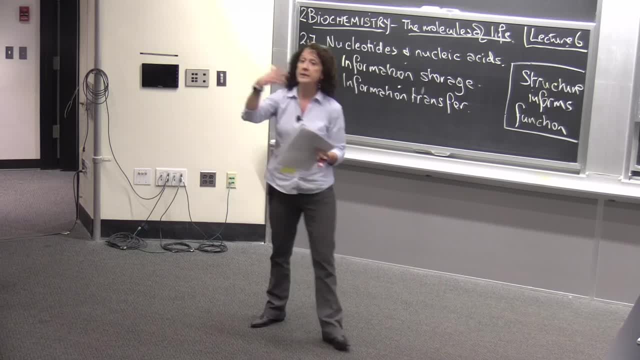 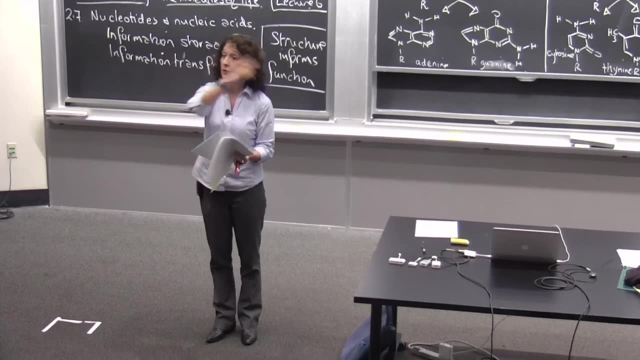 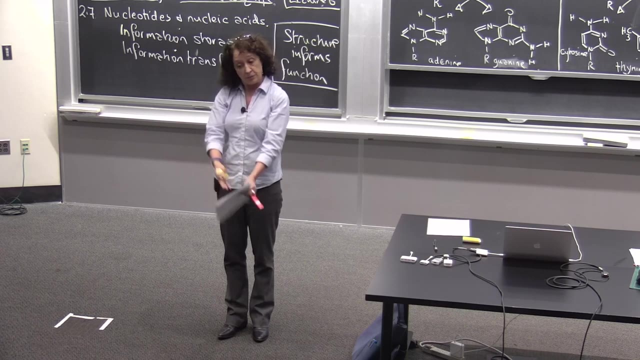 the biosynthesis of our proteins, And now we're understanding more and more about not only that, but also how RNA- not DNA- is involved in a large number of regulatory processes. So it's not just DNA. double-stranded DNA goes to a messenger, and so on. 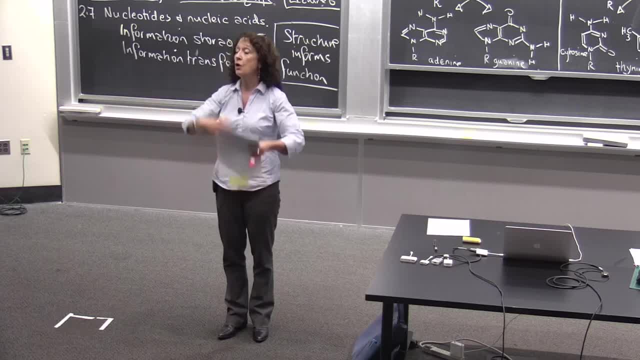 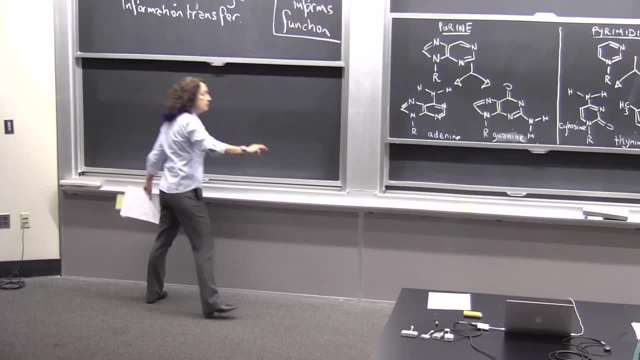 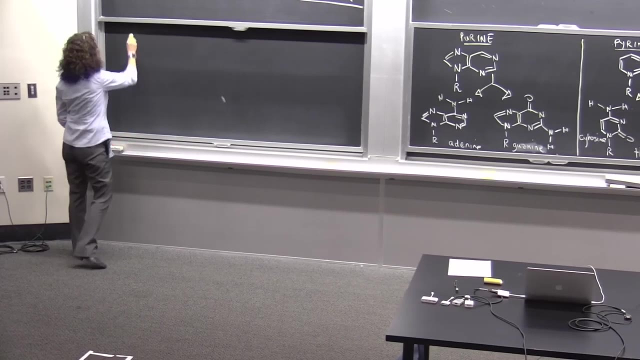 There's also a lot of regulation occurs because of a lot of the other nucleic acids that are within the cell. So I'm going to go here because I want to describe the composite components of nucleotides so we understand their structure. We understand their structure and their properties. 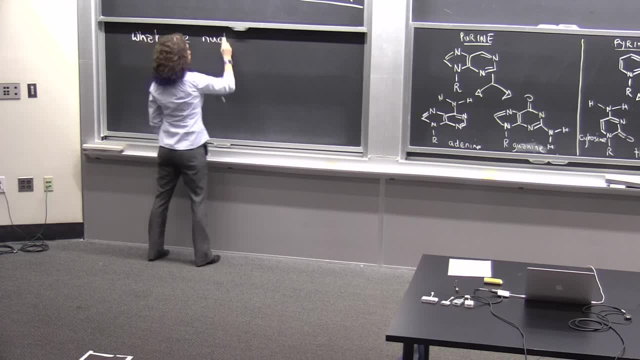 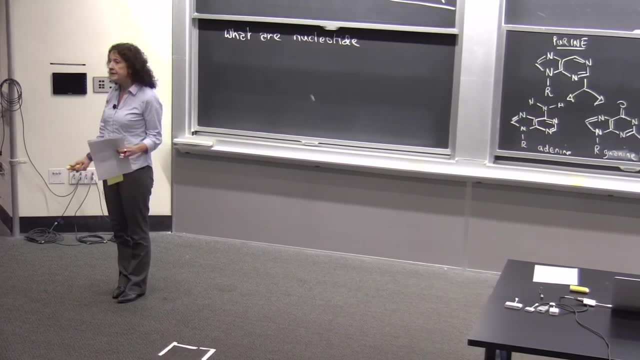 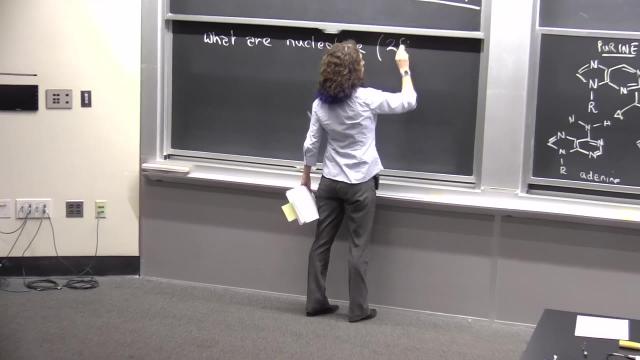 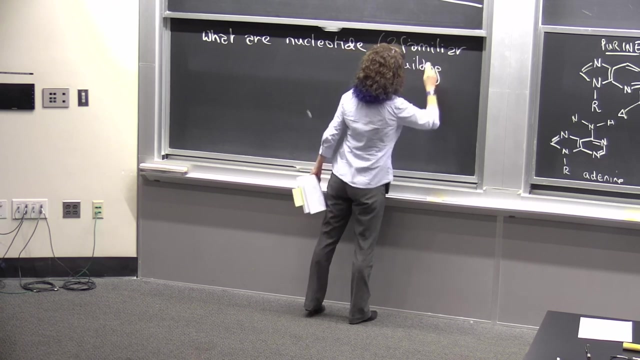 So what are nucleotides? And you look at these structures up on the board, they look kind of complicated, So let me deconstruct them for you. It'll make life a lot easier. So they're two familiar building blocks And one new one. 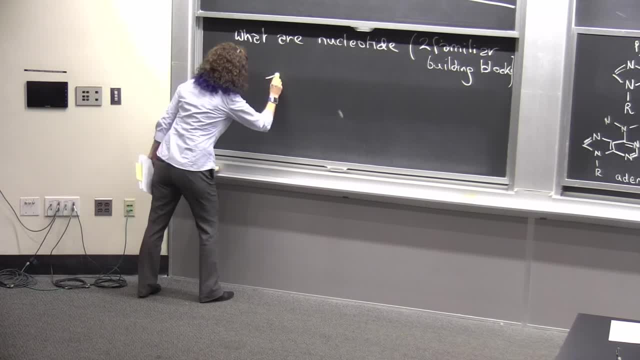 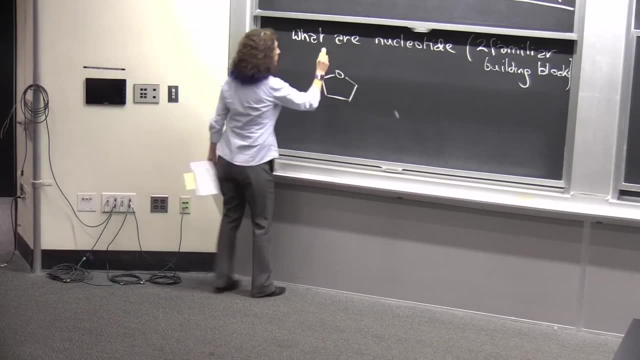 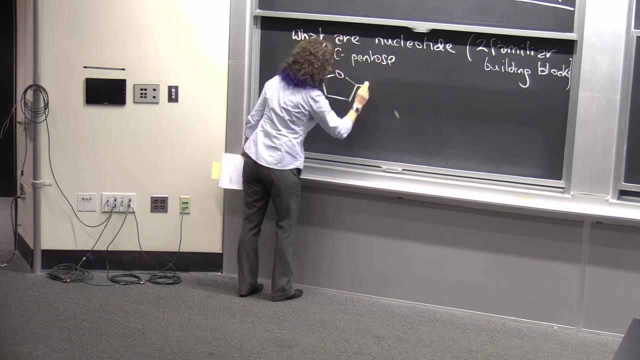 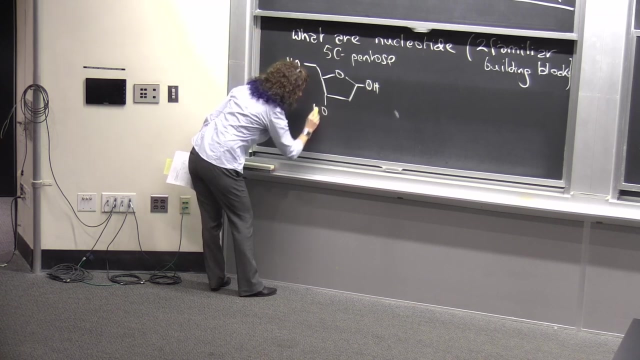 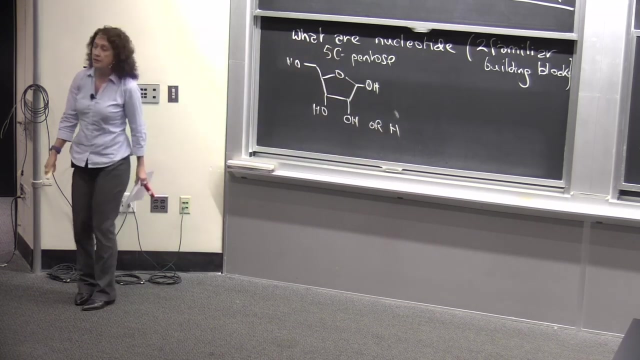 So the familiar building blocks are first of all carbohydrates. So the key carbohydrate in nucleic acid is a 5-carbon pentose sugar Which looks like this: You can count the carbons 1,, 2,, 3,, 4, and 5.. 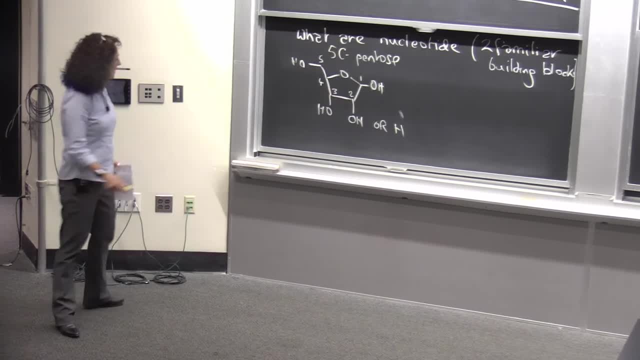 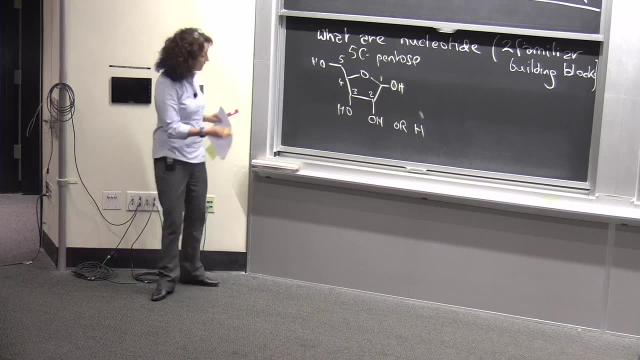 And you can reassure yourselves: everything is there. with respect to the carbons, by translating this line angle drawing into a drawing where you put all the hydrogens on and you know where everything is. There are two types of 5-carbon pentoses that are used in the nucleic acid. 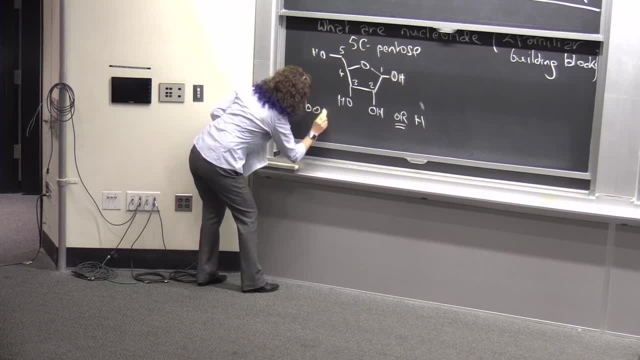 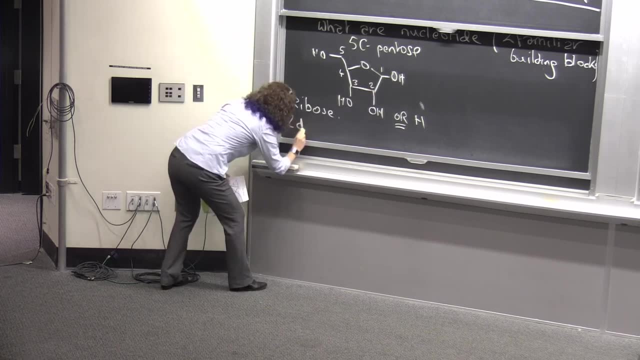 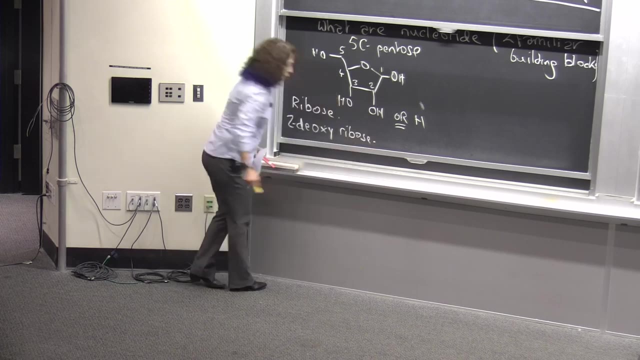 They are ribose. OK, So ribose, which is shown here, with all OHs, on all of those carbons, and 2-deoxyribose, which is a building block of DNA, whereas ribose is a building block of RNA. 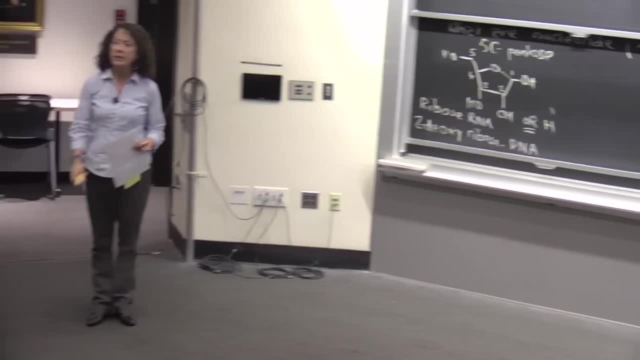 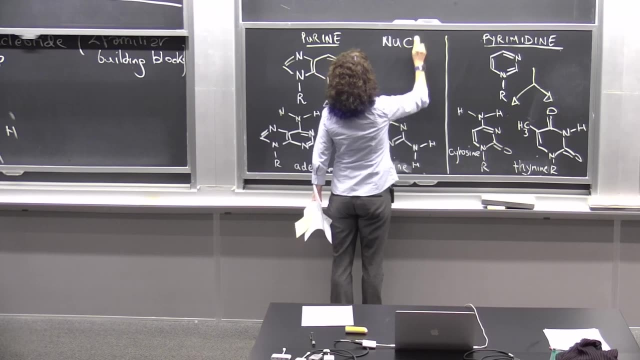 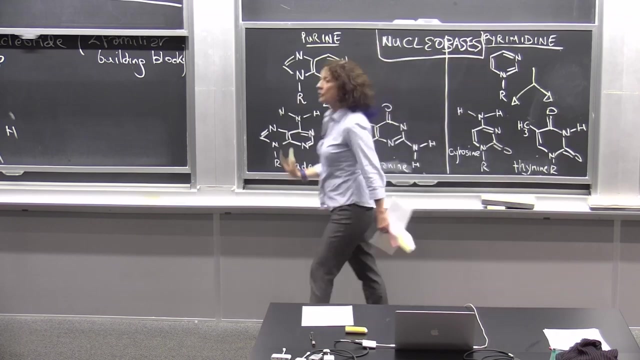 What else do I need to tell you- You'll see this later on- That ribose sugar ends up being called ribose, which is the ribose that's being connected to these, what are known as nucleobases. You do not necessarily need to draw those. 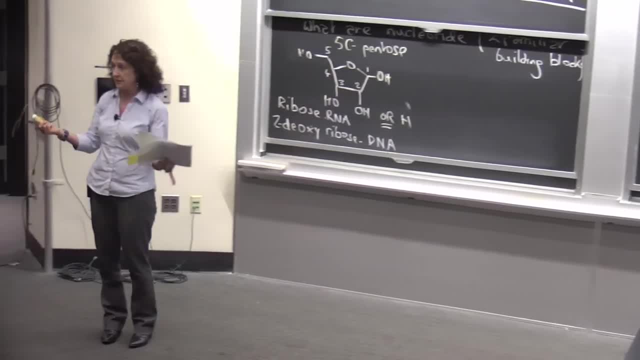 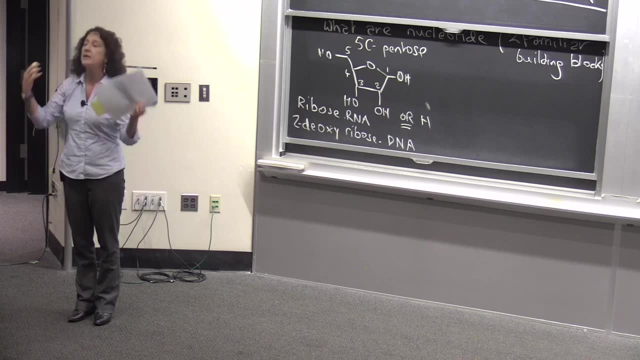 because you've got them on your handout to put sketches on. So I put them on the board for my, so I don't have to stand here and draw them for you And I want to explain certain things. So the nucleobases in the numbering system: 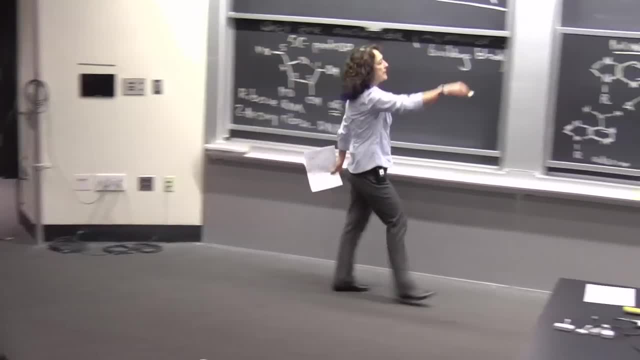 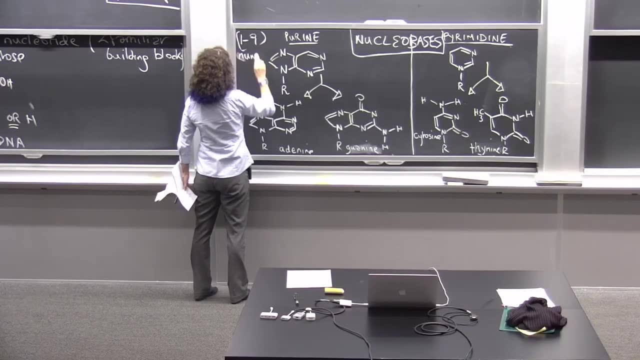 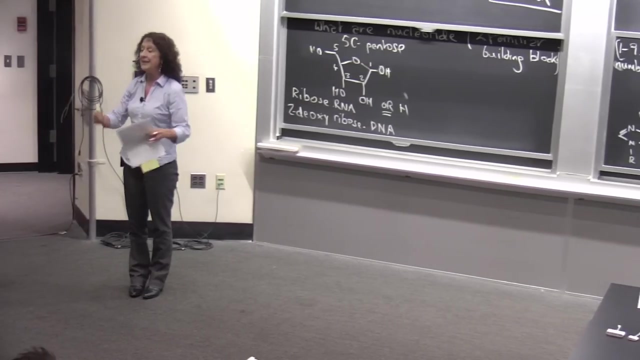 and I'm going to keep on reiterating this, so you'll get along with it- number the carbons one through whatever it is, or rather the atom numbers, when you're walking around the ring. So when we talk about the ribose component, 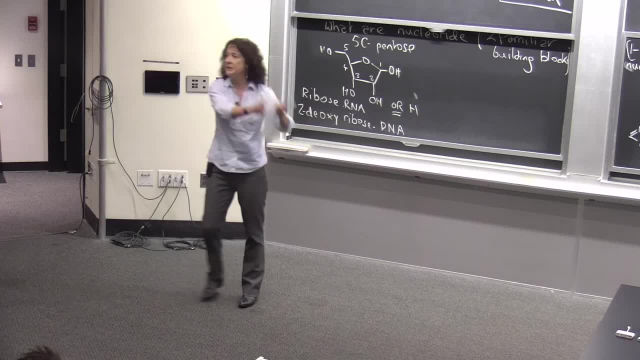 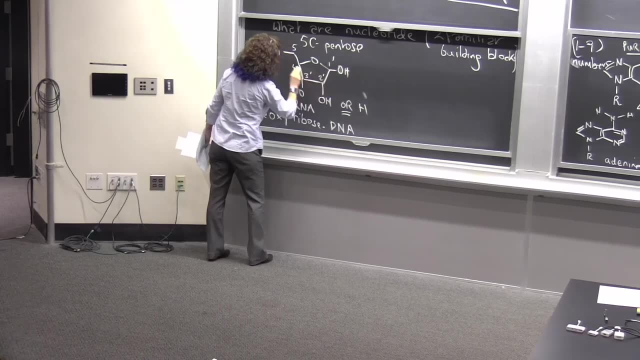 they have what's known as a prime numbering system to differentiate it from the numbering system in the riboses. So this would be 1 prime, 2 prime, 3 prime, 4 prime or 5 prime. Why is that? 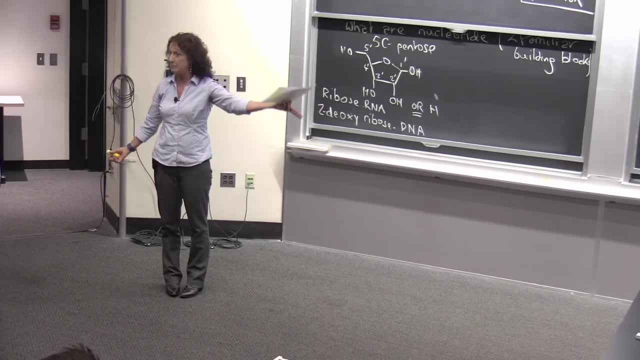 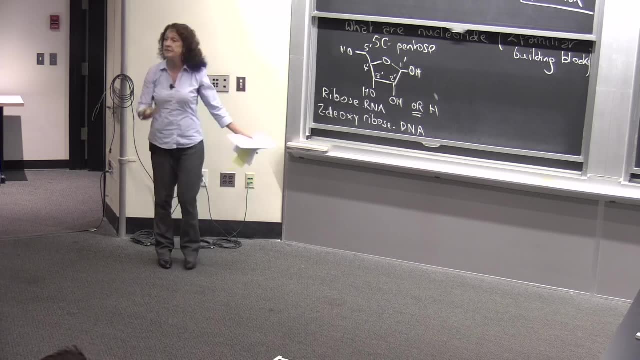 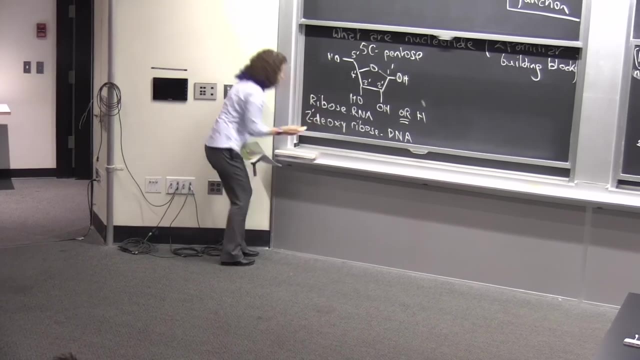 This becomes incredibly important when we talk about putting together polymers of DNA and the direction in which DNA is assembled in life, And also even when we describe 2-deoxyribose or ribose, because this would be called 2 prime deoxyribose. 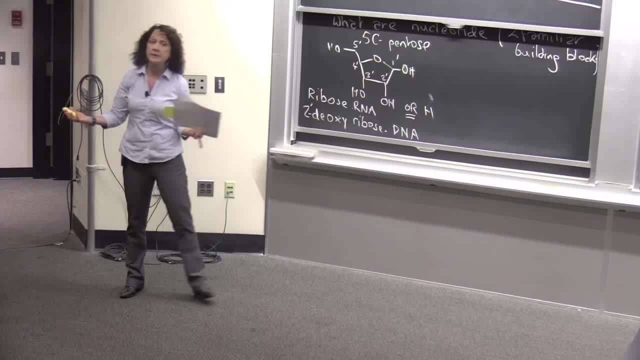 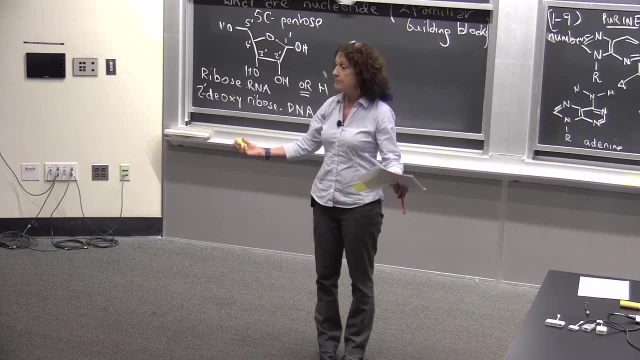 in the nucleic acid. So I'm going to bore you with that numbering system because I'll start to use it very commonly And it will make a lot of sense as we start to assemble the DNA, the macromolecule, when we talk about the way it's. 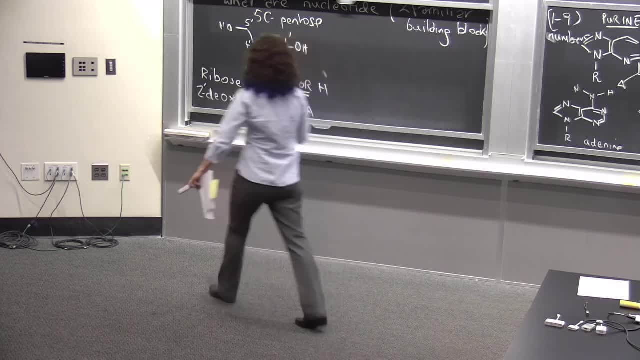 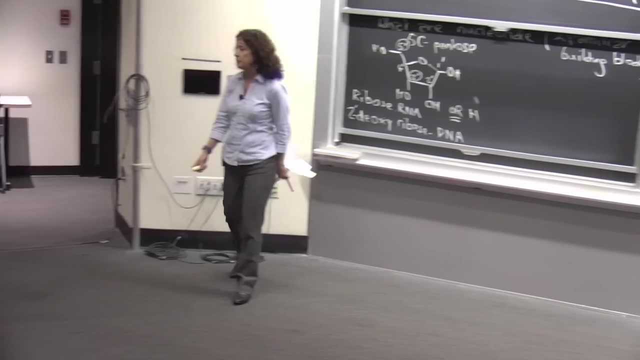 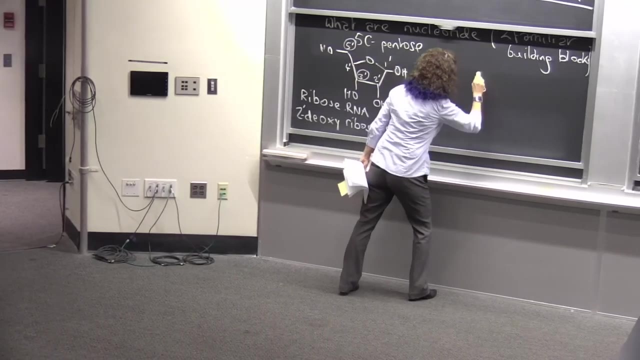 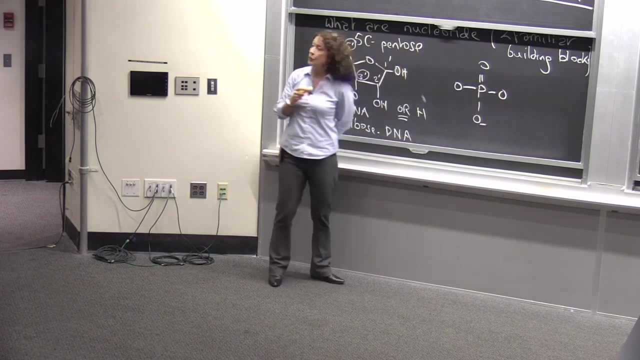 built and drawn and written. The numbering system will be important because we'll constantly refer to 5 prime and 3 prime. That's just a little preview for later. The next component of the nucleic acid is a phosphate. Phosphorus looks like this, but in nucleotides. 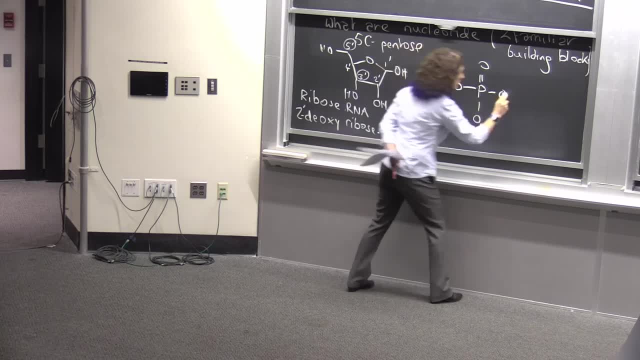 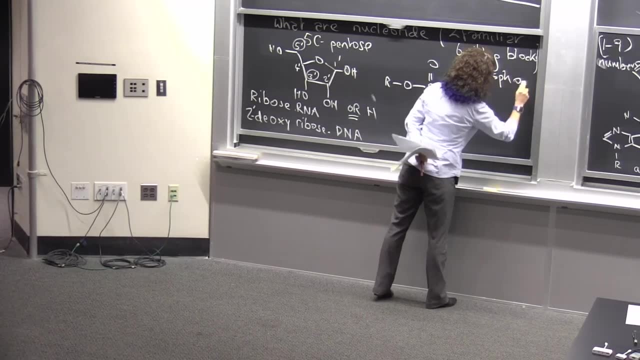 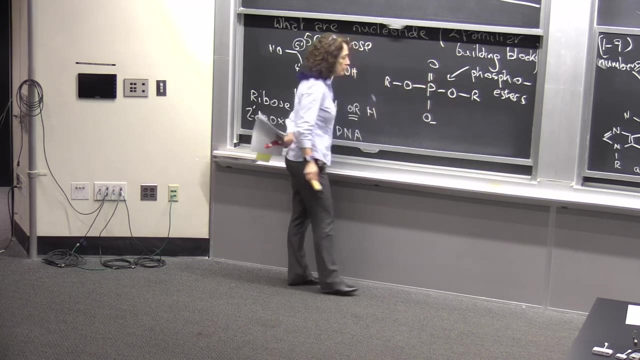 these are joined to other units as phosphoesters. But you want to remember that in phosphorus you have 1,, 2, 3, 4, 5 bonds to phosphorus And you commonly have a negative charge on one of those oxygens. 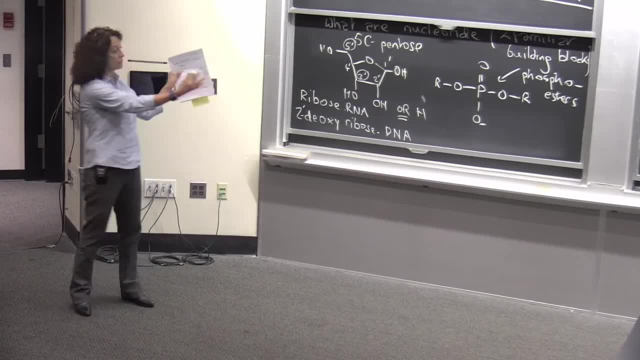 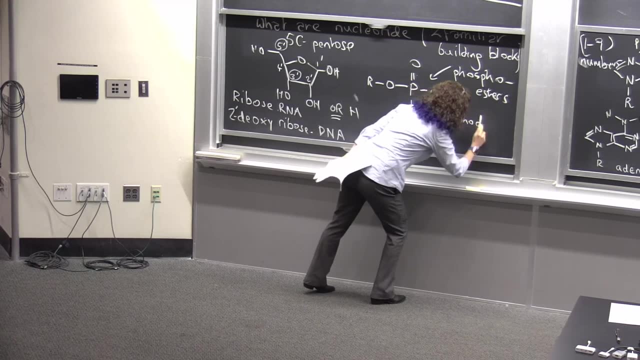 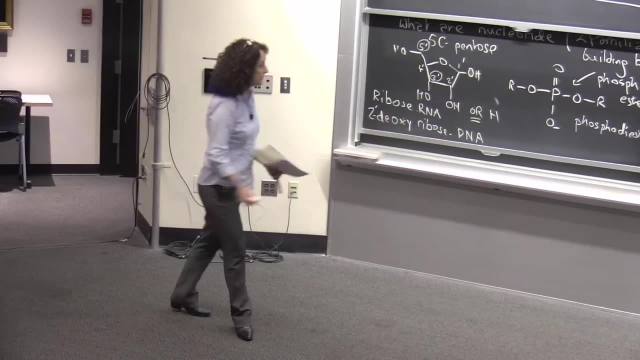 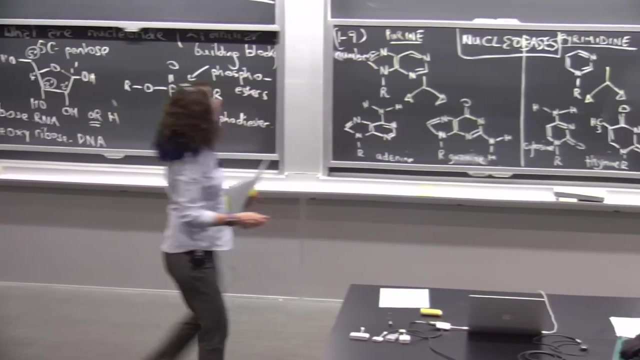 And in the structure of DNA you actually have phosphates occurring as phosphoesters, So diesters, And once again you will see that when we see the intact structure of DNA. So what are nucleotides? Nucleotides are a combination of a carbohydrate or a sugar. 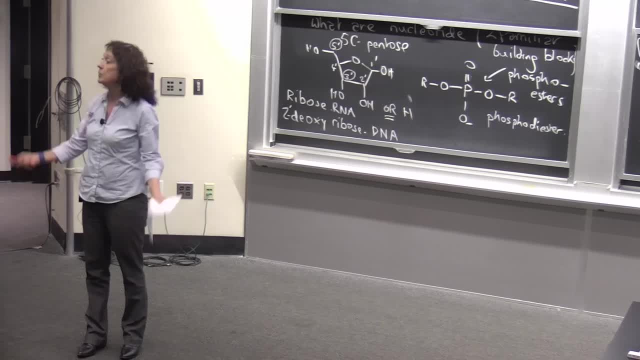 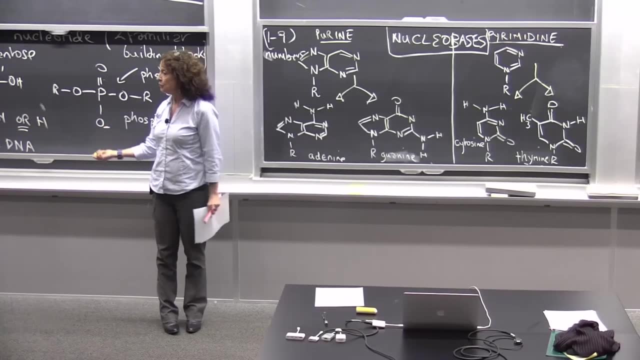 a phosphate and a nucleobase. That's the third component, the one we're going to learn about now. OK, So the nucleobases look like this: There are two families, two flavors of nucleobase. There is one flavor. 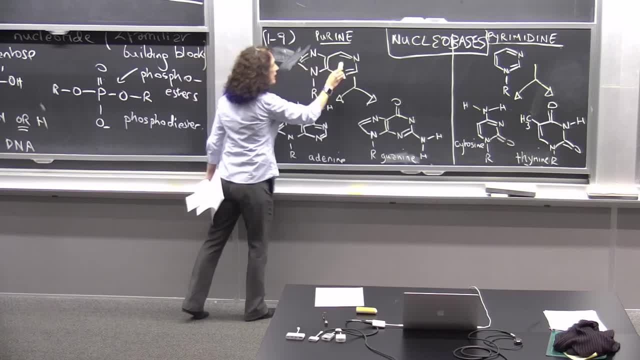 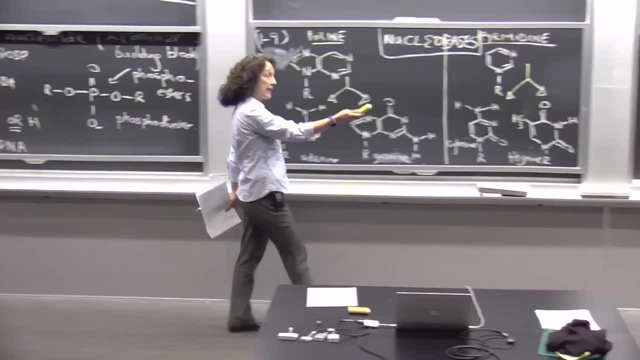 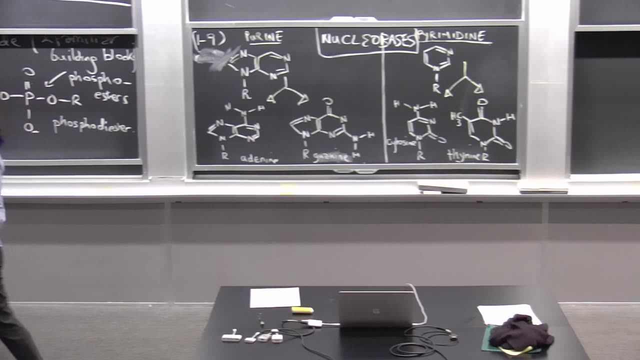 Let's get this cleaned up a little bit here. That has two rings and it has the shorter name, purine, And there's a different family or flavor of nucleobases that has one ring and it has the bigger name And that, to this day, is the way. 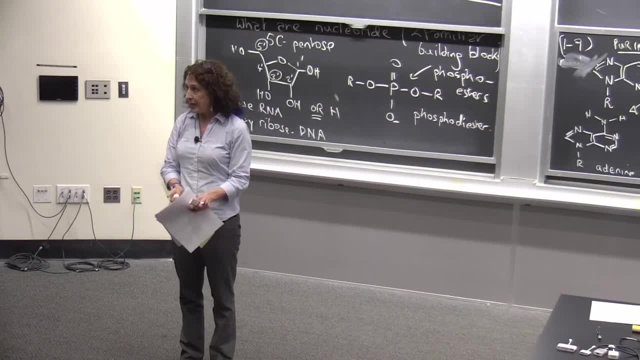 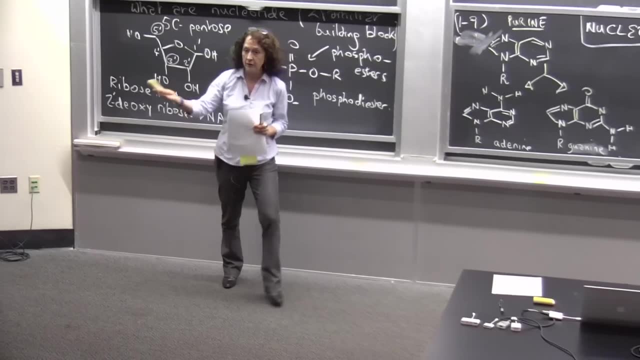 I remember purines and pyrimidines. So small name, big structure, big name, small structure. OK, If that's helpful to you, go for it, Use it. I haven't patented it or anything, all right, OK. 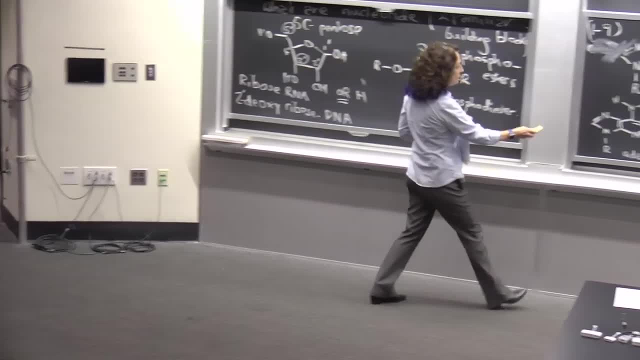 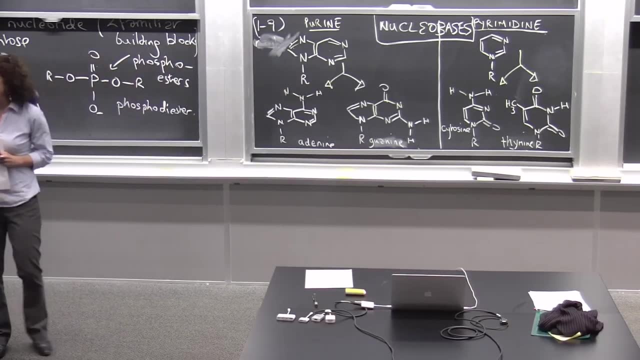 So in nucleic acids there are two different purines. They are known as adenine and guanine. You do not need to know these structures. I actually only know my favorite three of the five to draw easily, and the other two. 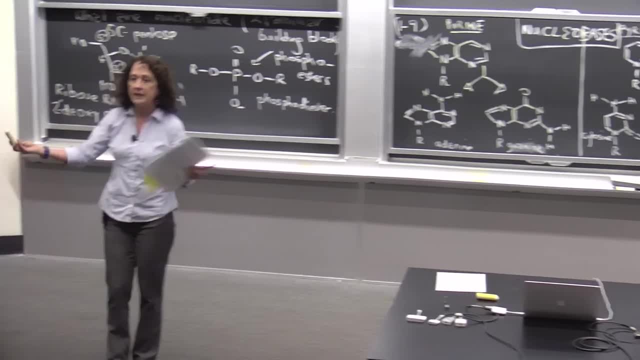 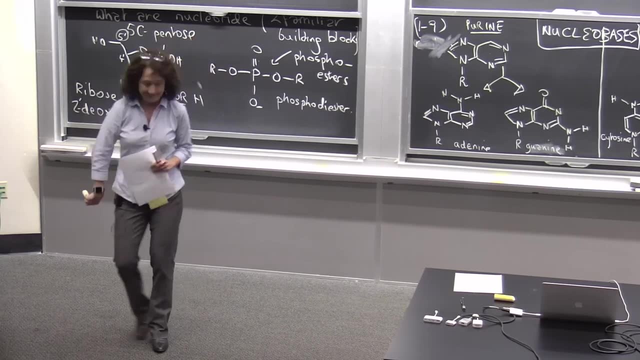 I'm always stumbling around the ring, So don't worry about that. We all get to know the ones we work with Every day. for me, it's uracil, it's adenine and it's cytosine, but not the others. OK. 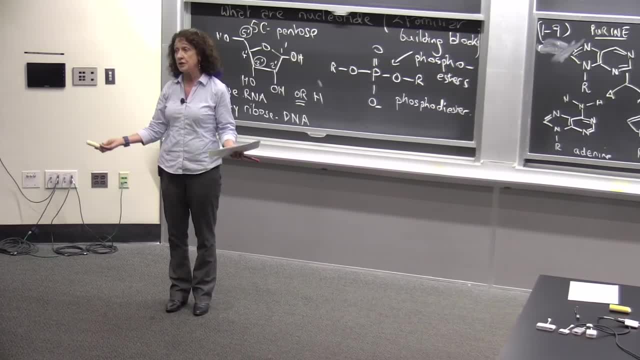 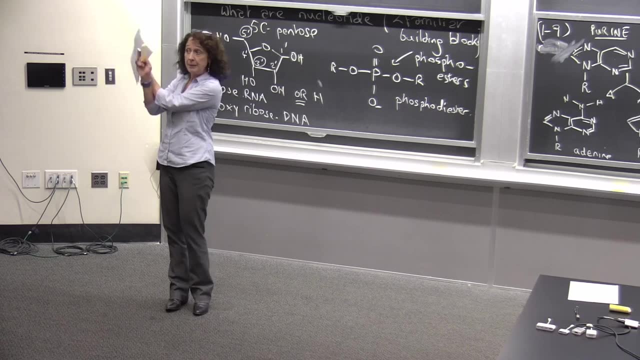 But what you do need to understand is a little bit about their structures, because when we start to talk about the non-covalent structure of nucleic acids, principally the double-stranded helix of DNA, we need to know where the hydrogen bond donors. 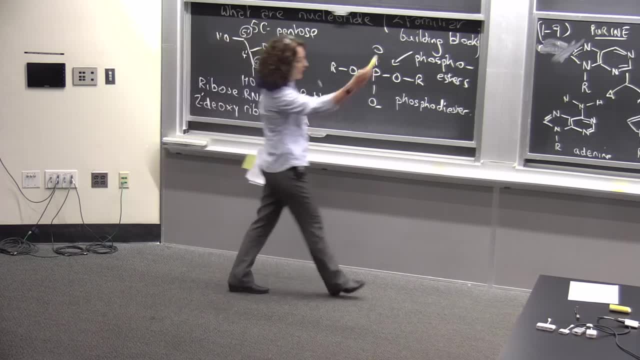 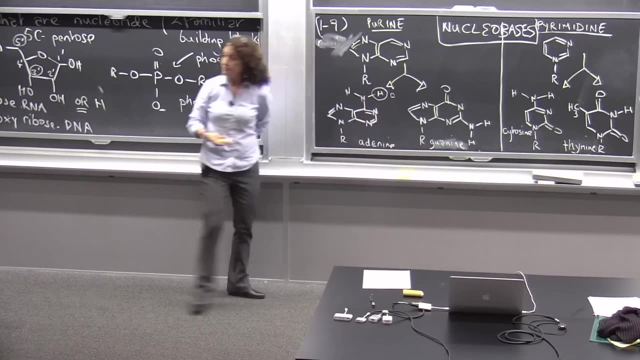 and acceptors are in these structures. So if you want to indulge me, you can take a look at these structures. This hydrogen would be a donor right. You can see that it's a hydrogen on a nitrogen. This nitrogen is interesting. 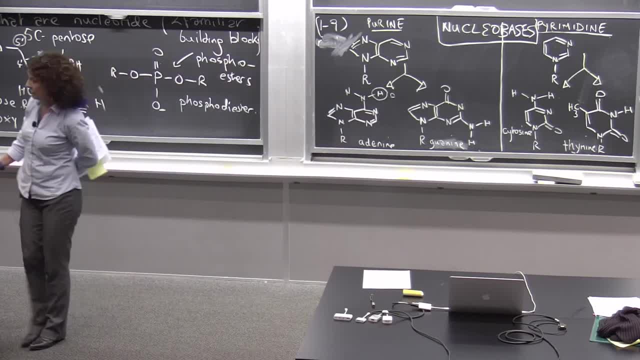 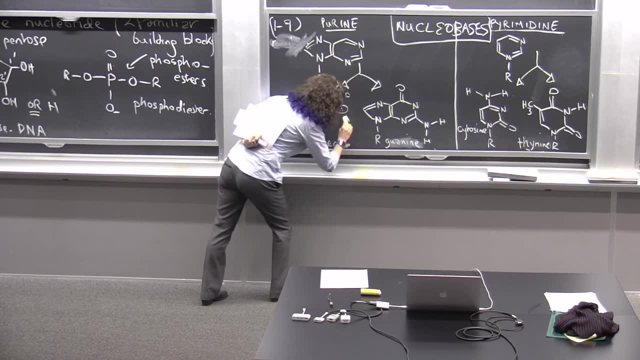 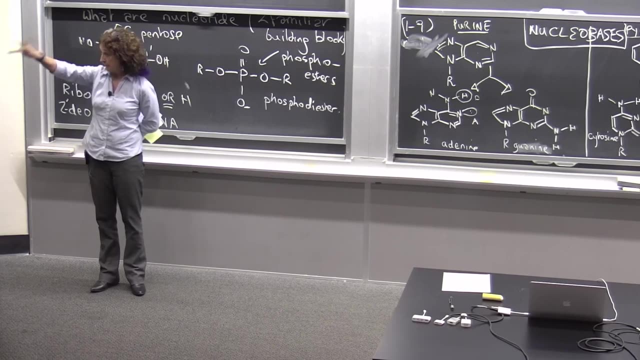 It has one, two, three bonds to nitrogen which means there are a lone pair of electrons also on that ring system. So that would be a hydrogen bond acceptor and the adenine nuclear base can accept and give a pair of hydrogen bonds. 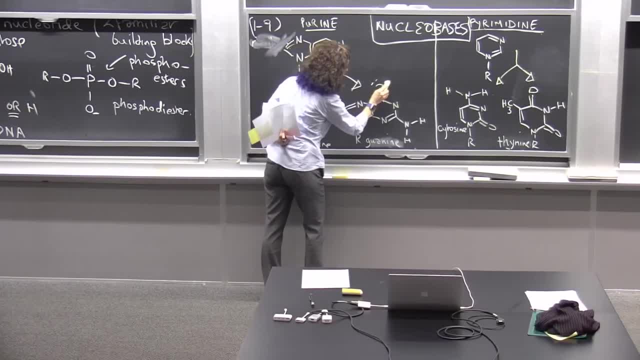 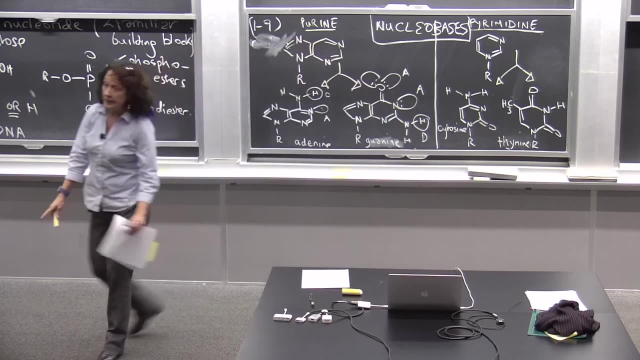 And you can work that out for all of the others. So in guanine there is an acceptor, another acceptor and a donor, and so on. So those rings in the nucleobases are very important because they have places. 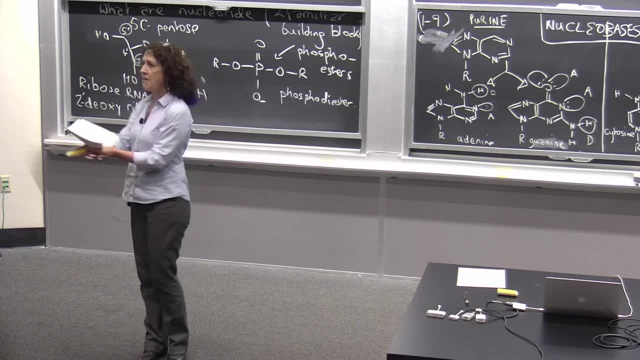 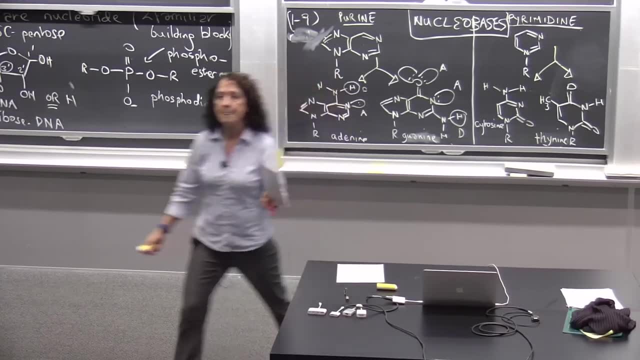 that you can hydrogen bond to Now. is everyone feeling comfortable about this? Does anyone want to ask me a question that might help clarify? OK, Because it's quite important. Yeah, Do you have a question? Would this urocyl play a part? Sorry, Urocyl, Urocyl These all are. I'm sorry, All these nucleobases have fancy names. OK, So so far I've shown you the structure of adenine, guanine, cytosine and thymine. 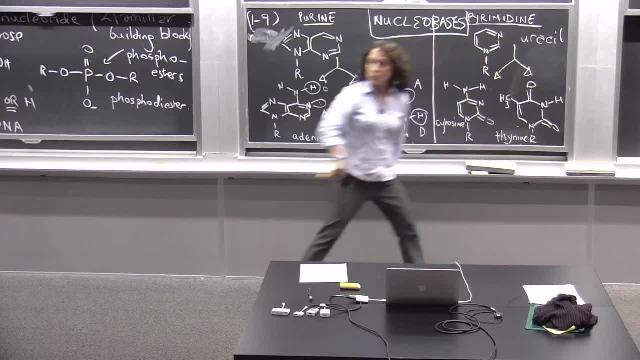 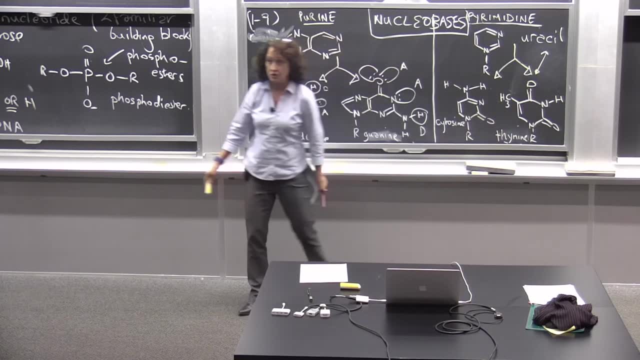 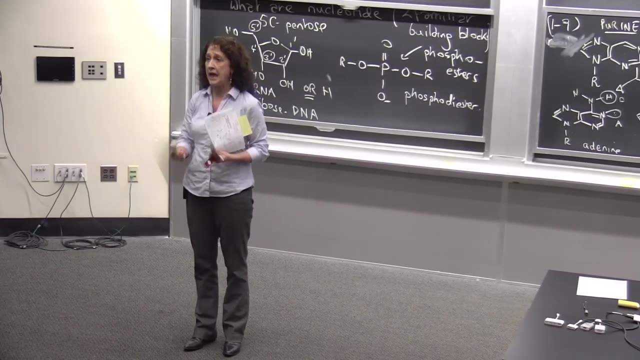 Urocyl, which is not drawn on the board, is very similar Thymine, except this methyl group is a hydrogen. OK, Knowing the names is also complicated. I really care that you understand the hydrogen bonding patterns, not to draw the whole structures. 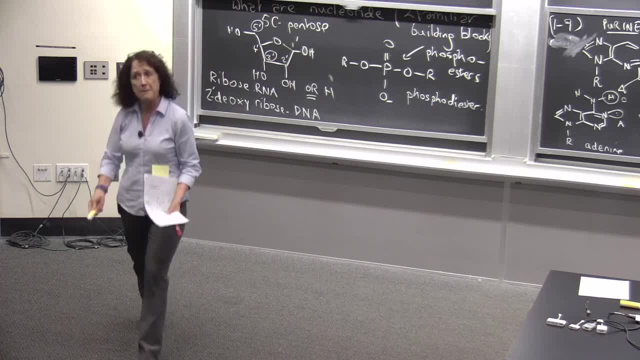 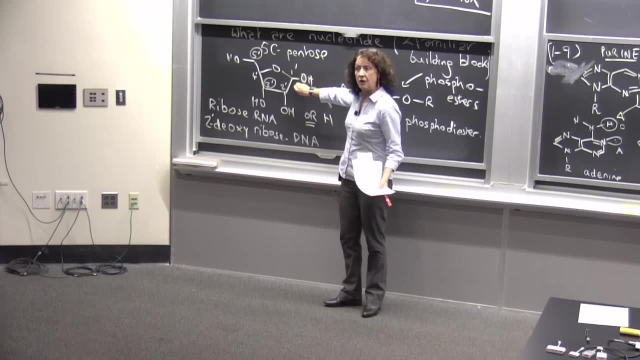 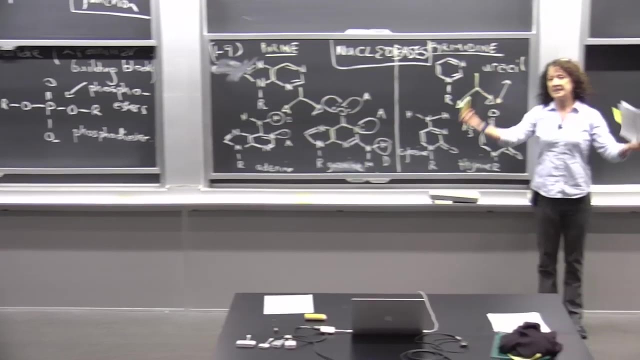 but to identify hydrogen bonding patterns, not to remember fancy names because there's no logic to those names, but really to remember ribose, deoxyribose, phosphate and phosphodiesters, Purines and pyrimidines- just the sizes of them. 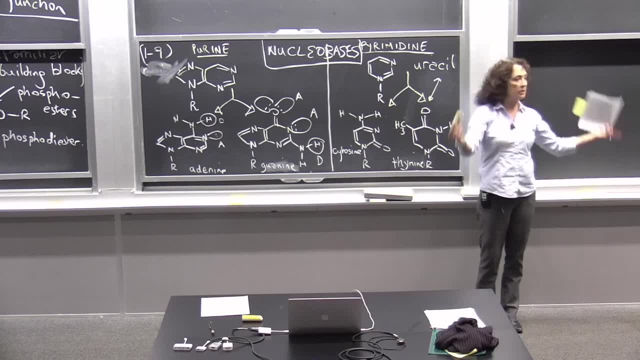 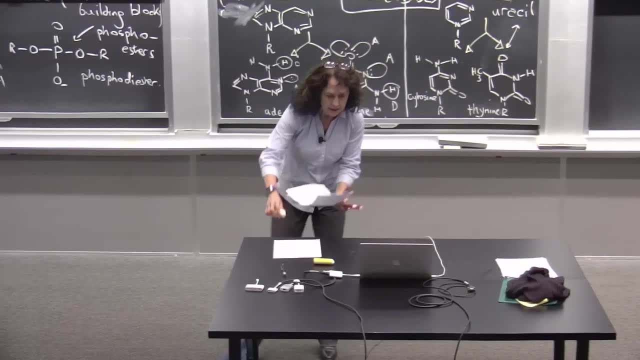 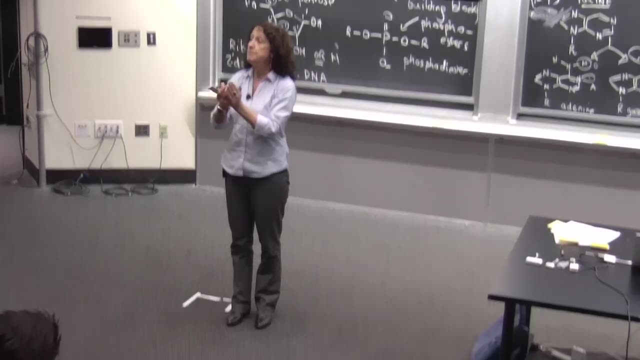 to pick them out. Does that make sense? what I want you to know and what you can remember. if you think it's interesting, OK, All right Now, in nature, we use the nucleotide building blocks or the nucleotides in many different ways. 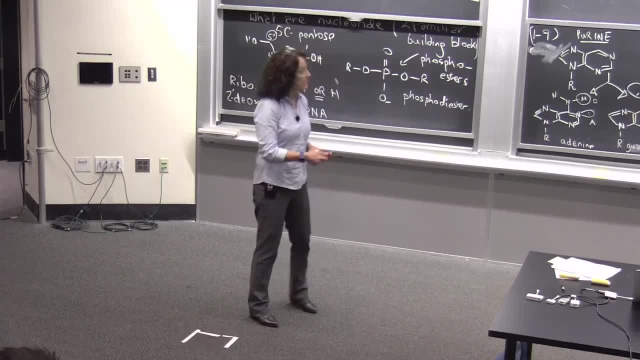 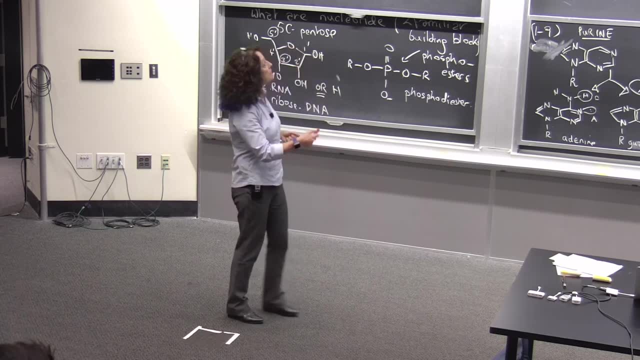 It's not just in DNA and RNA, And so here I'm showing you some really important nucleotides that are found in nature, And I'll give you a little bit of information about their signaling. So here are the components that you can pick out. 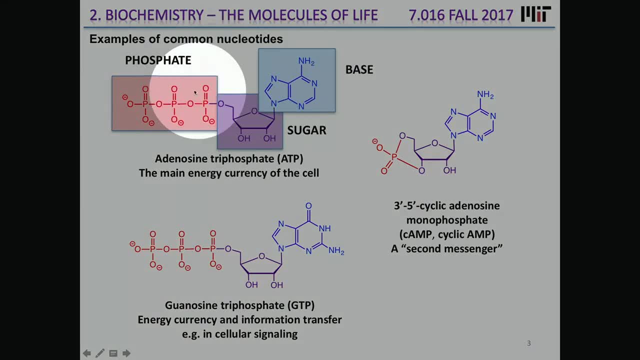 There is, in this case, a ribose sugar. In this case it's phosphate, but it's a phosphate triester. So it's got three phosphates in a row And here's a nucleobase which is a purine. 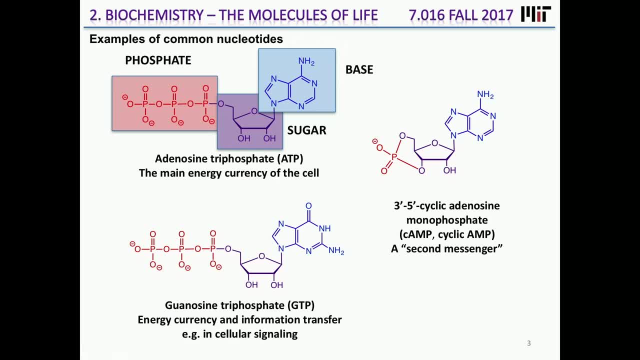 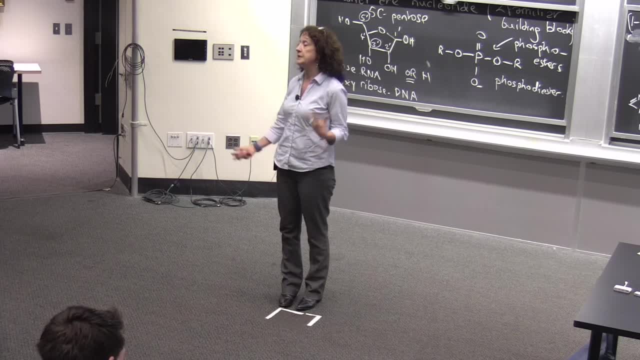 And this is adenosine triphosphate. So it's one of the bases, one of the nucleotides, a nucleotide that's used in energy, energy transfer. In a lot of metabolic processes we use ATP as a molecule that has energy that can be unlocked. 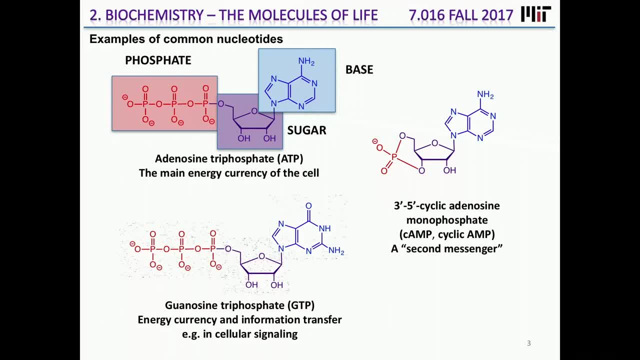 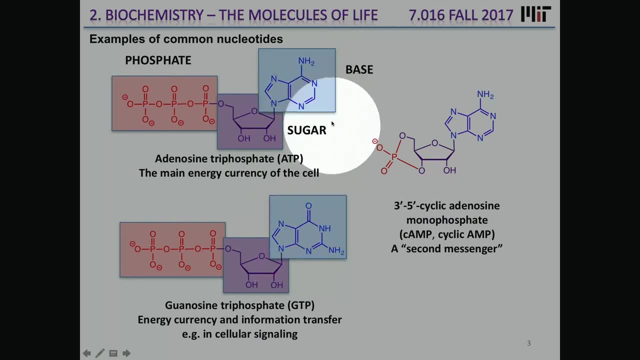 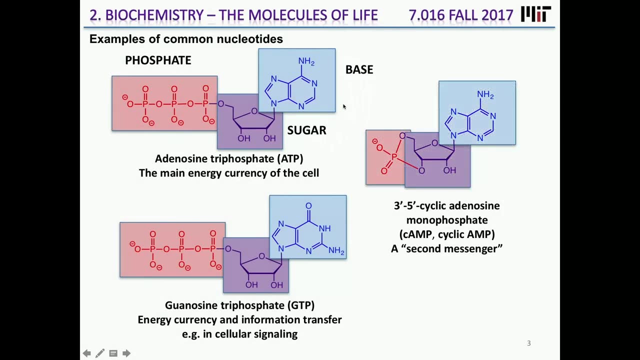 for chemical processes. There's another one of these, which is guanosine triphosphate, where the nucleobase is different. They're both purines, but they have different structures. You can see them there. And then, finally, the last one I show you. 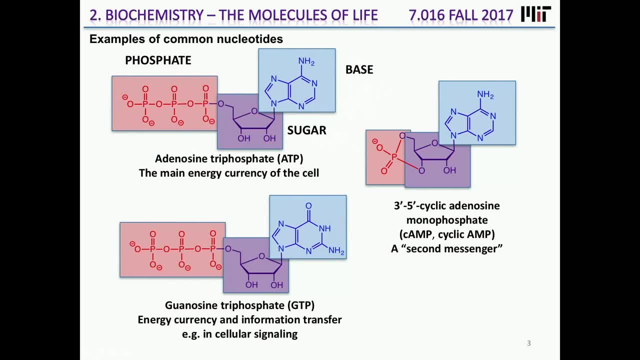 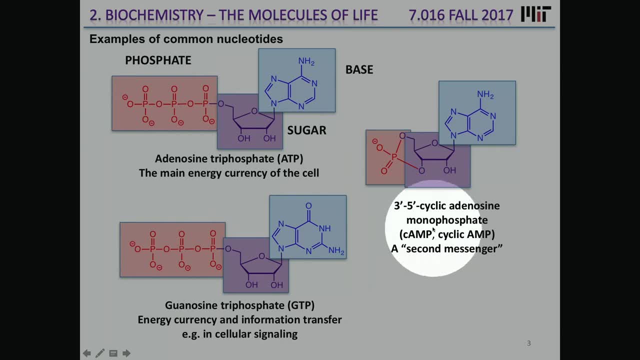 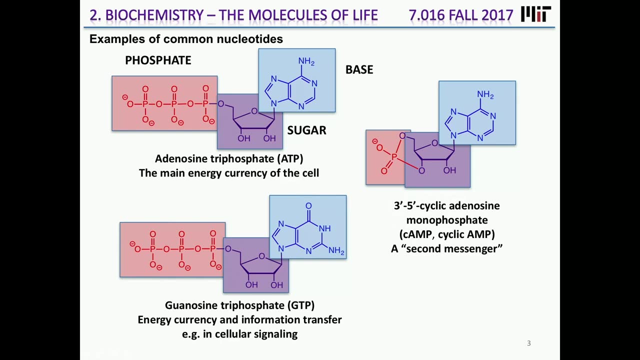 here is a nucleotide that has a cyclic phosphate, but it still has a nucleobase, a ribose and a phosphate, And this is cyclic AMP. And when I come back, after Professor Martin has talked, we'll talk about the role of cyclic AMP. 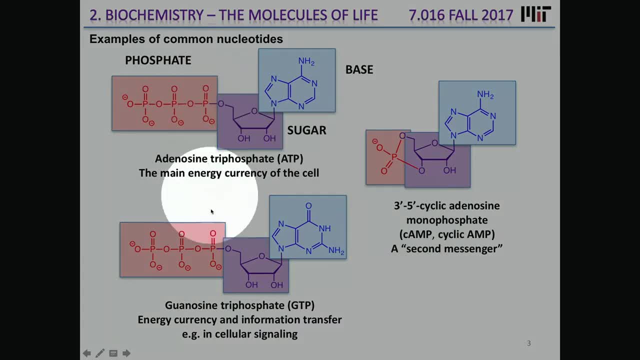 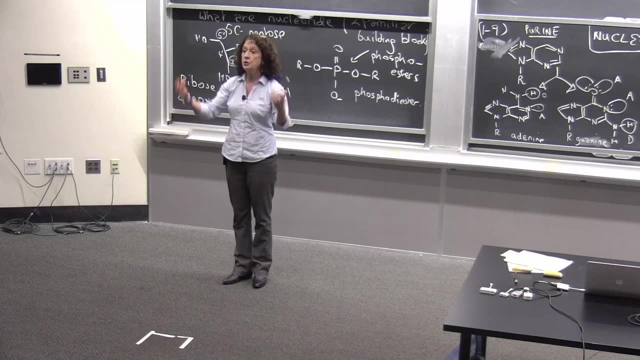 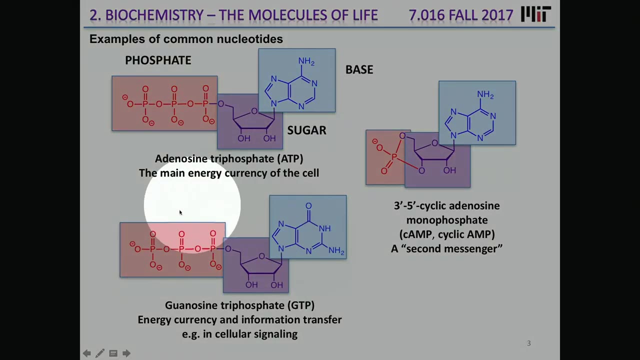 as a second messenger. So these two molecules, in addition to being building blocks for DNA and RNA, also are forms of energy, where you can use ATP or GTP as a form of energy in a lot of metabolic processes. And in fact, though, when we start. 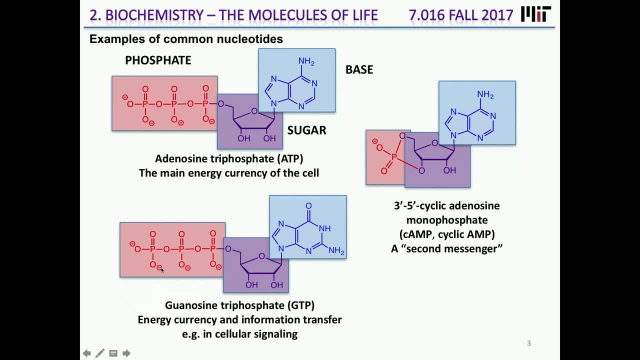 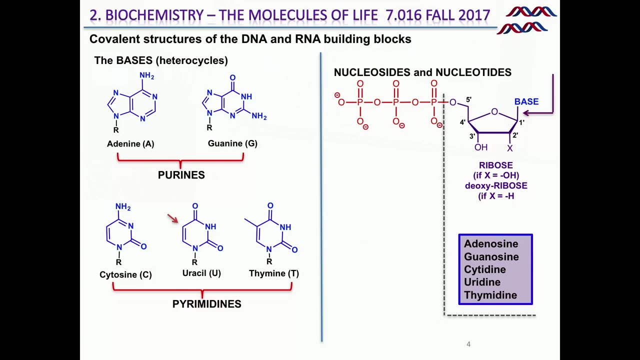 constructing proteins using the ribosomal system. you'll notice we use GTP as a form of energy, not ATP. It's interesting how nature chooses to do that. Any questions about this? OK, all right, One tiny wrinkle left to deal with. 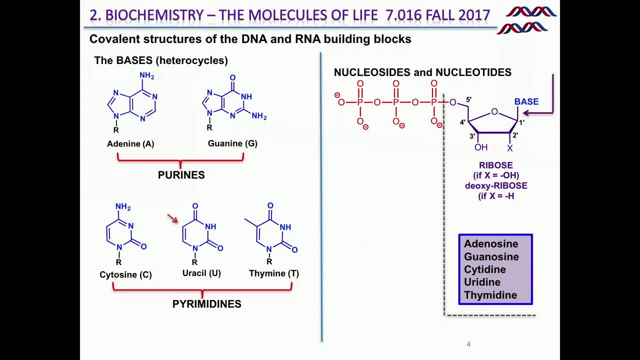 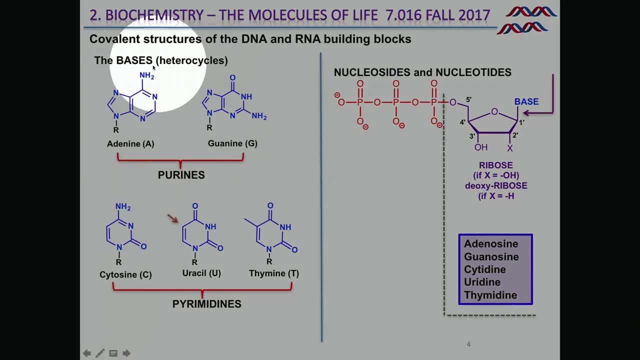 and that's a little bit more about those building blocks for the nucleic acid and one more item that it's useful to understand the name of. So here are the five nucleobases, two purines and three pyrimidines. 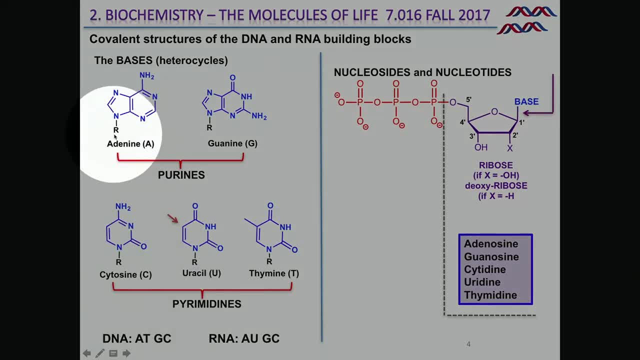 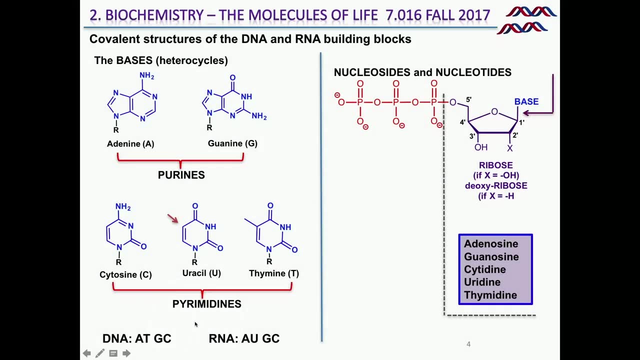 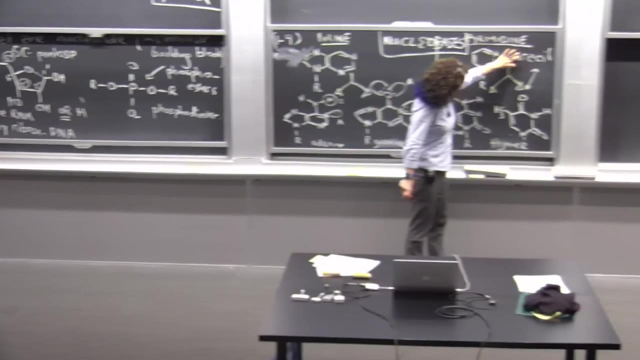 In DNA. we have A, T, G and C. So A, T, G and C. So we have different building blocks. Three are common to both polymers. One is different: Uracil and thymine are exchanged. 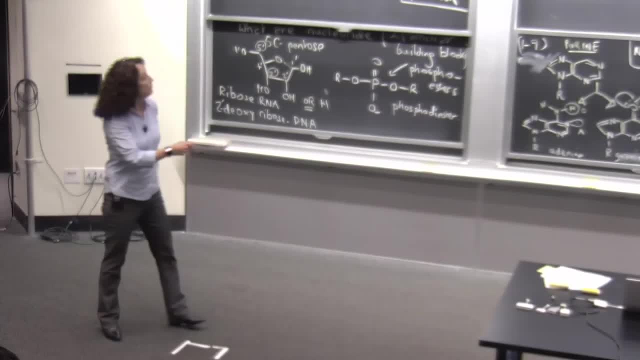 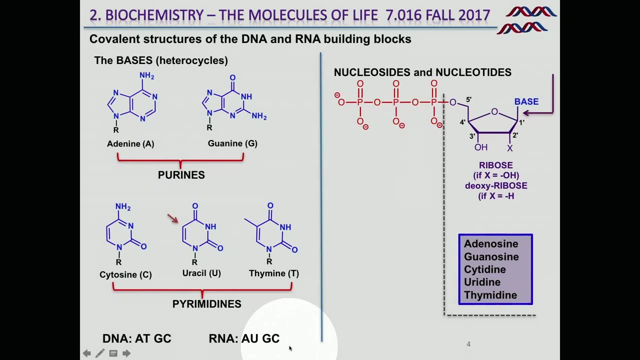 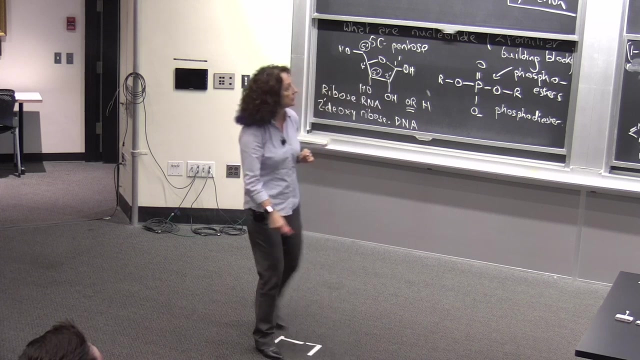 when you go from DNA to RNA. The pyrimidines are cytosine, uracil and thymine, And in RNA you have A, U, G and C. So there are reasons for these differences and I'll nudge into some of those chemical differences. 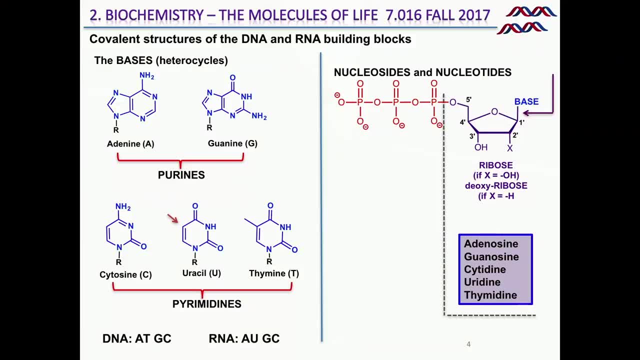 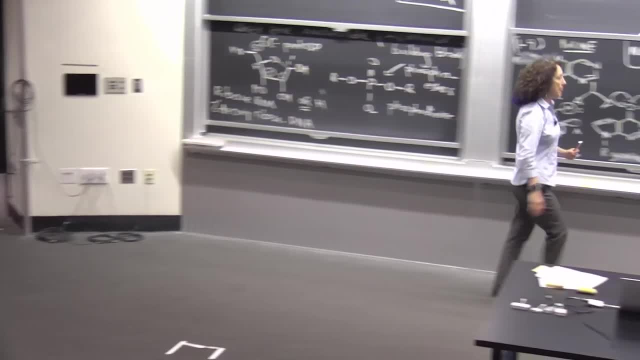 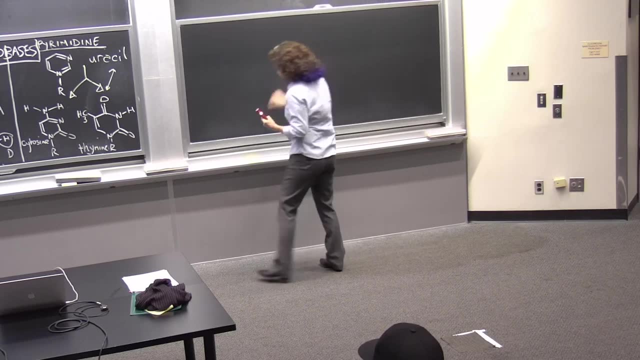 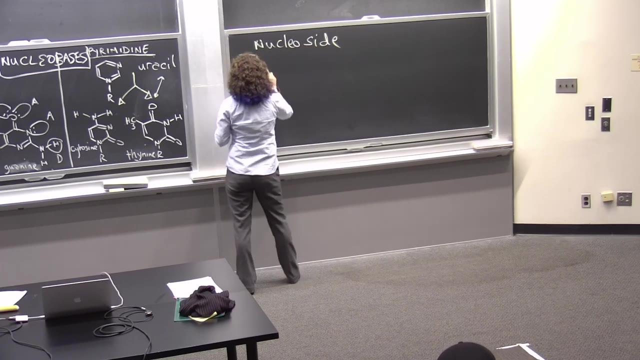 in a moment. So the information up there is the same information that I have on this board. The next thing I need to talk to you is: we very commonly use the term- well, two terms: nucleoside and nucleotide. How irritating is that. 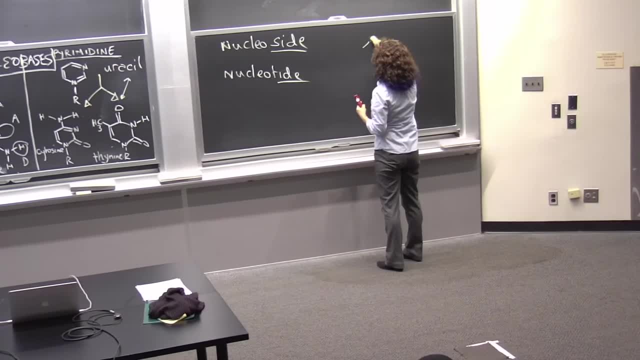 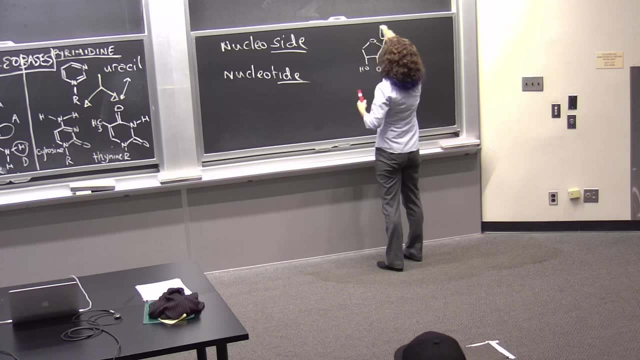 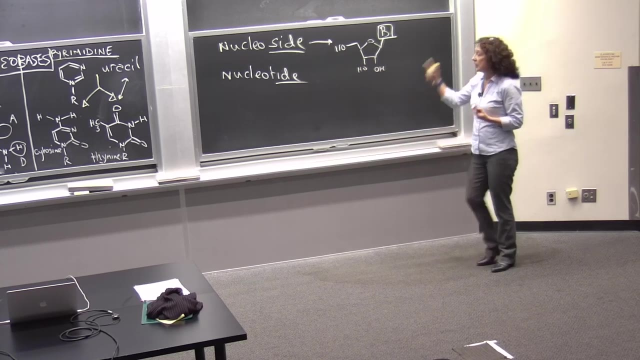 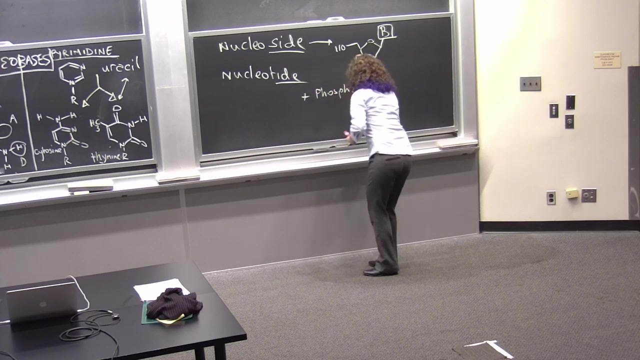 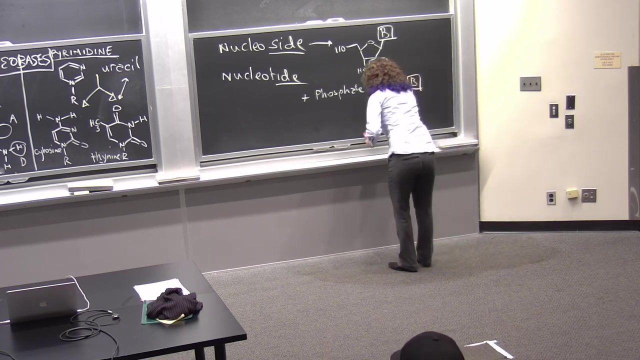 The nucleoside is just the ribose. The ribose has two probes plus the nucleobase, but no phosphates. As soon as you put on phosphates they become nucleotides. So for example, nucleobase, ribose and in this case a phosphate on it. 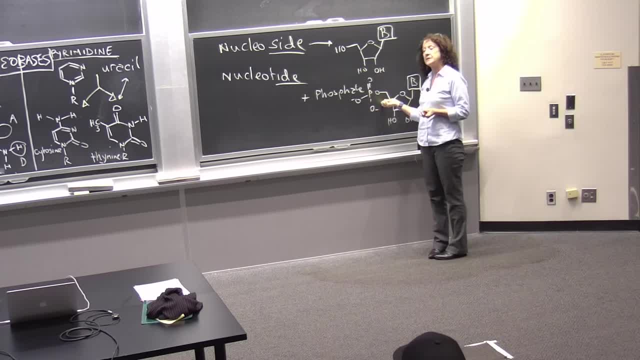 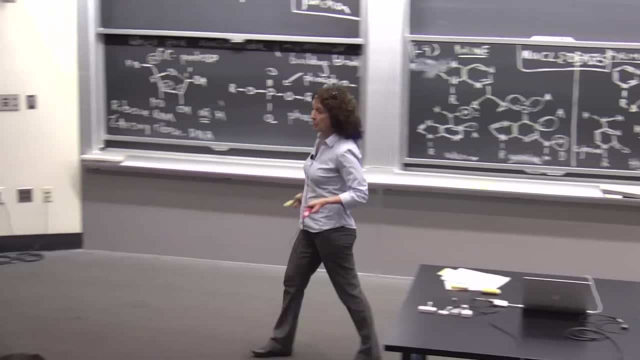 And that becomes a nucleotide. No matter how many phosphates they are, it's called a nucleotide. I'm less concerned that you remember that nomenclature more than you know what it's all about, because otherwise it might become a little bit confusing. 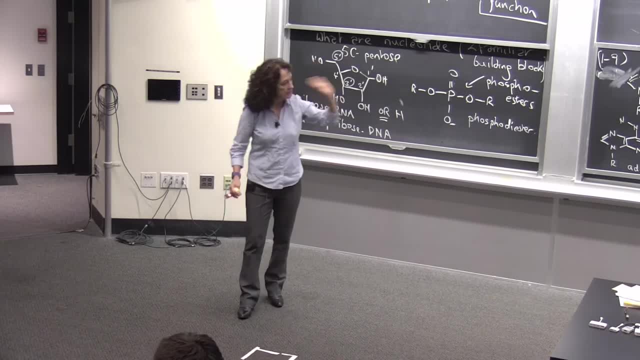 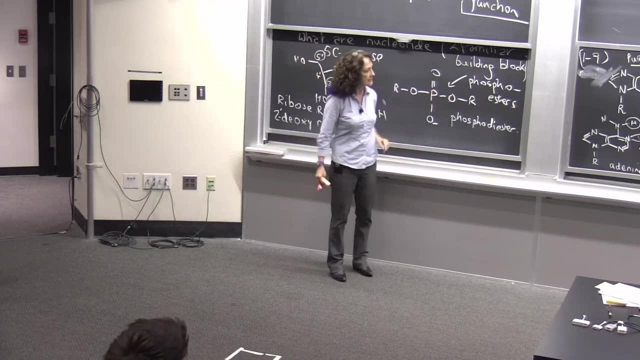 So just remember, if you can remember that, But I think I've tried to define the things I would like you to remember: the building blocks, their numbering system, the phosphodiester linkages and the nucleobases. as far as understanding where donors and acceptors. 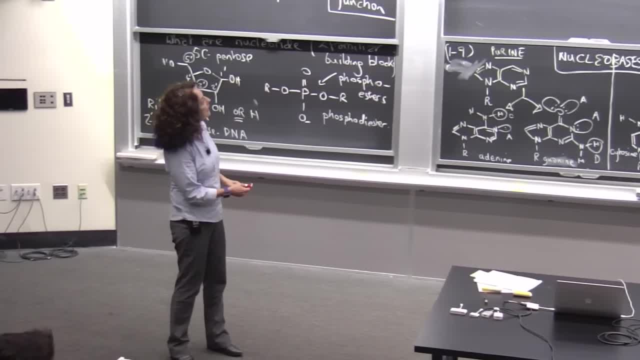 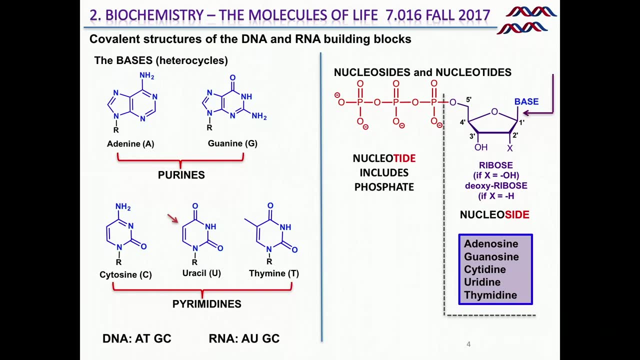 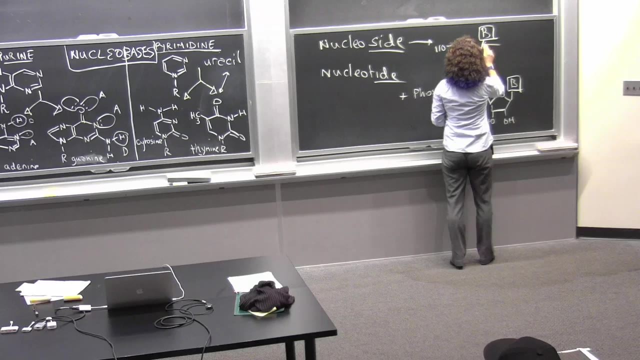 are for hydrogen bonding. all right, OK, And there's one thing: so we call that a nucleoside, whereas we call it a nucleotide when it includes the phosphates. And there's one thing that you want to notice is that the bond from the nucleotide 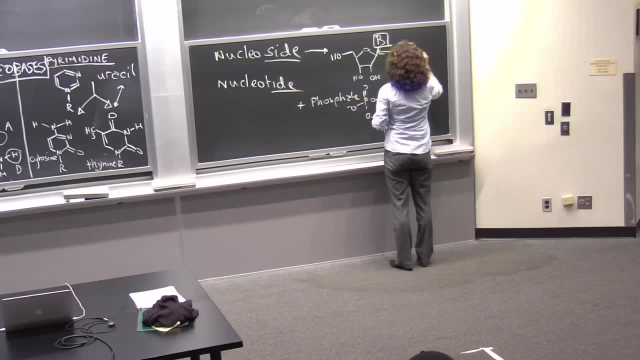 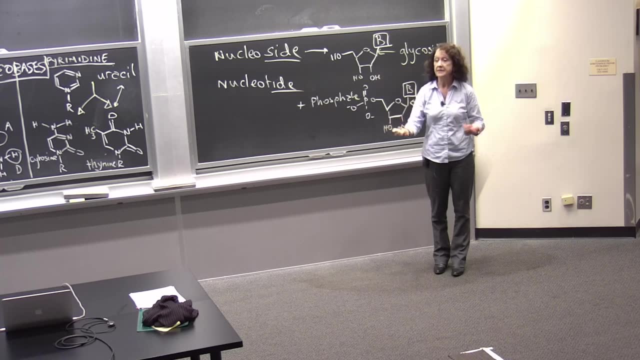 or base to the ribose, is a glycoside bond. It's a bond to a carbohydrate, so that's why it's called a glycoside bond. There are glycosidases that cleave the bond from the base to the sugar. 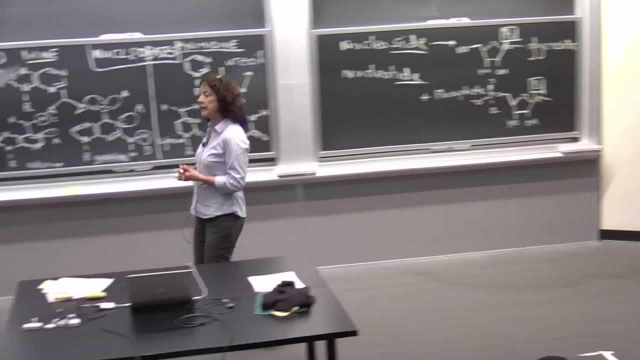 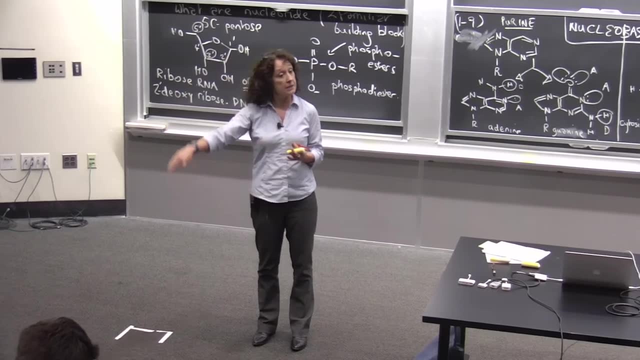 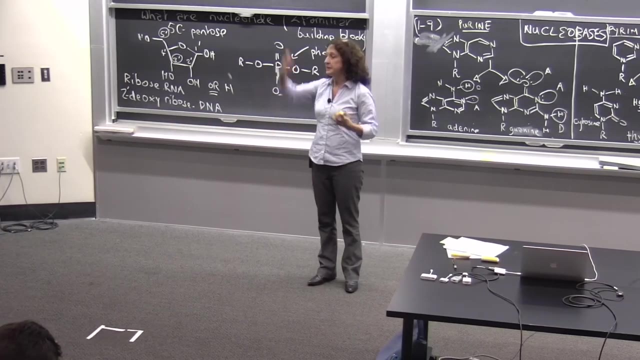 Those are very important when we have mutations in our DNA and we want to cut out the sugar, to fix it so it doesn't get misread in the biosynthesis of DNA, In the biosynthesis, In the biosynthesis of messenger RNA. So that bond is important. 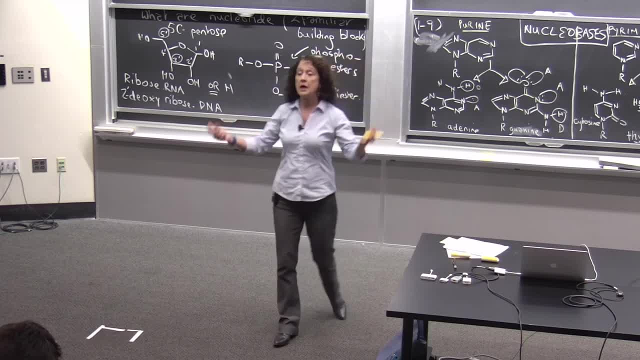 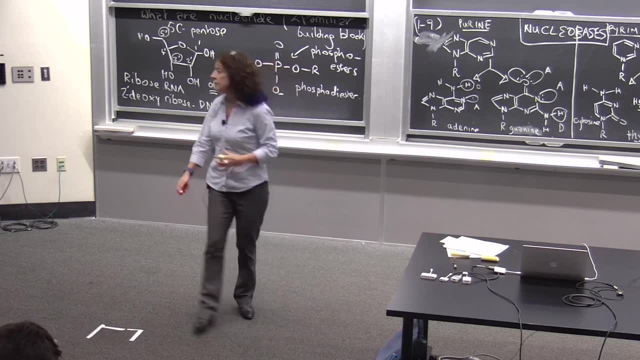 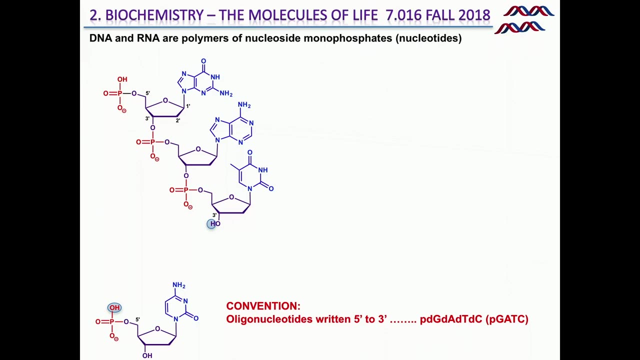 We may often talk about it, but only when we get to learning about how DNA sequences are corrected if there are mistakes in those sequences- and that will be later on, OK. so let's start to now look at the polymers. Now I want to tell you that by the early 1900s, 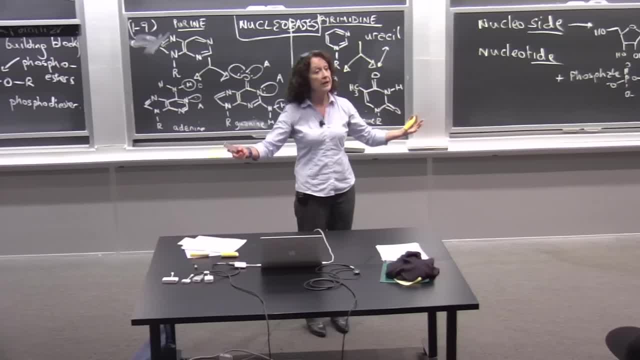 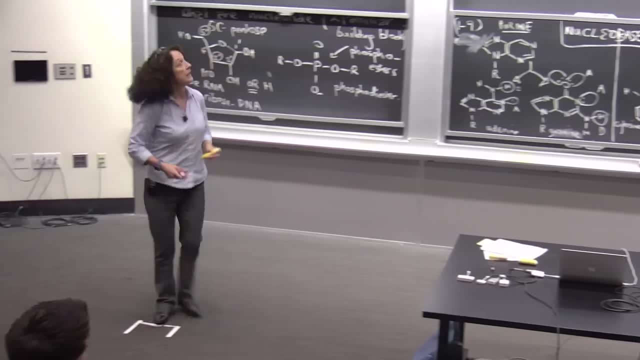 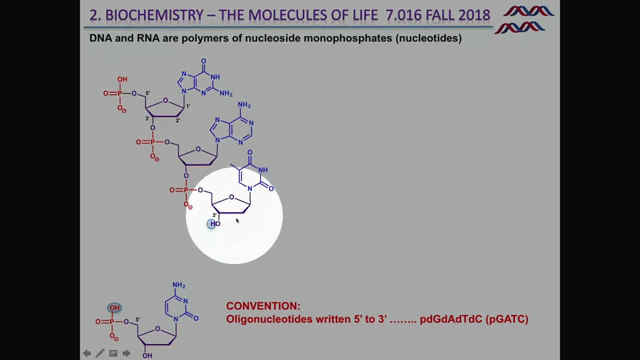 people pretty much knew the structure, the non-covalent structure, of DNA, and I'll describe it to you now. DNA is made up of nucleotides and this is its basic structure, where you have a phosphodiester backbone linking riboses. 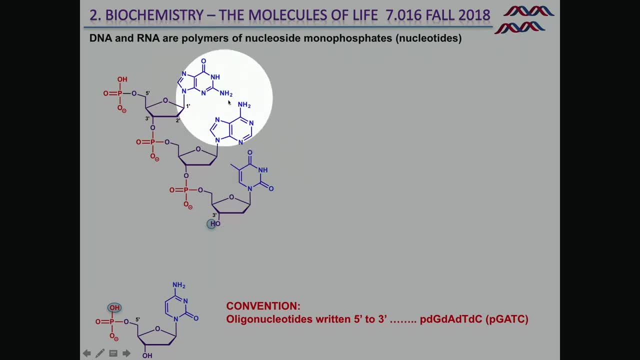 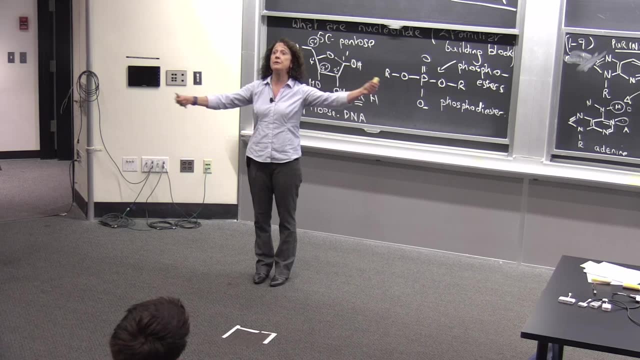 and each of those riboses is modified with a purine or a pyrimidine, And that is the basic structure of a nucleic acid polymer. only it's very, very, very, very long. So let's take a look at the components here. 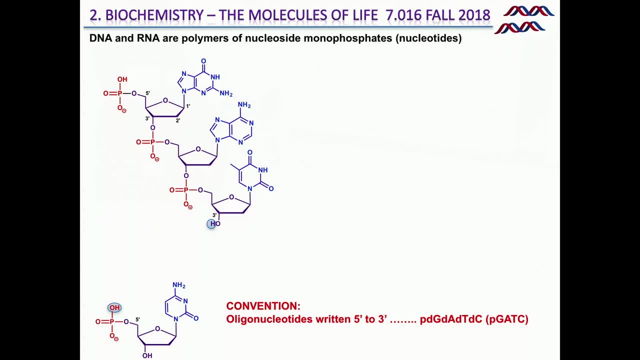 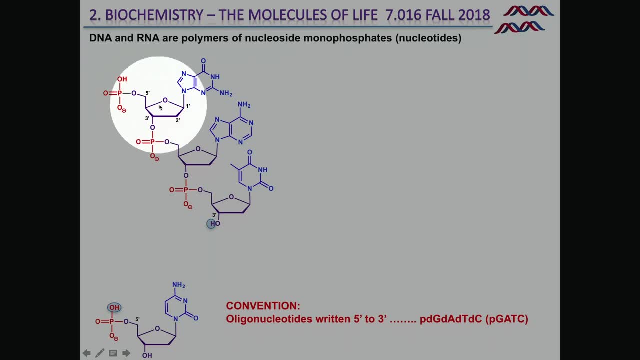 look at the bonds And maybe on your notes just highlight the bonds and some of the things I'll talk about. So first of all, the numbering system. here we always talk about a nucleic acid and we describe the sequence of the nucleic acid based. 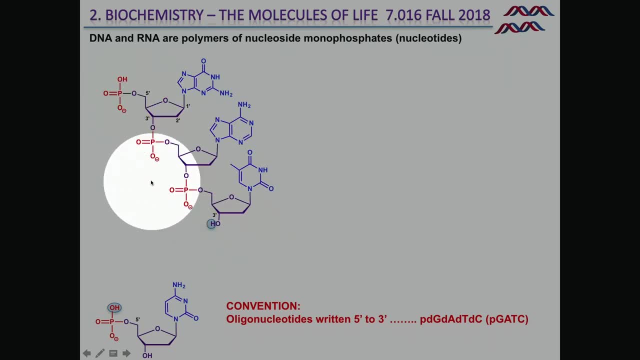 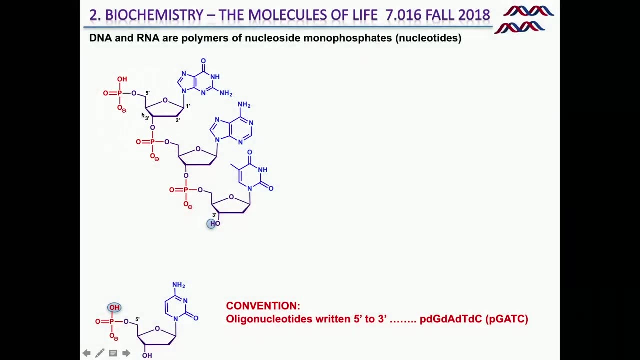 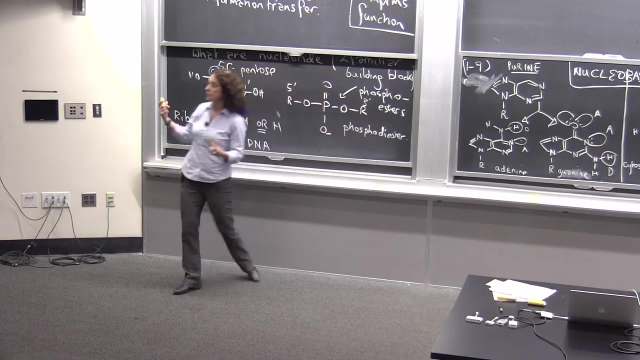 on from 5 prime to 3 prime. because the phosphodiester bonds join the 5 prime. there should be a number there and the 3 prime site. So the linkage would be here would be 5 prime and 3 prime joining to the ribose molecules. 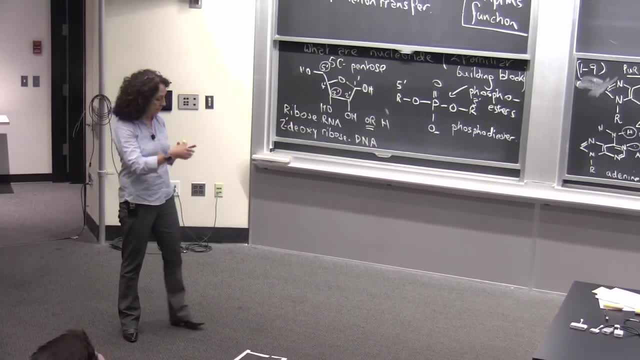 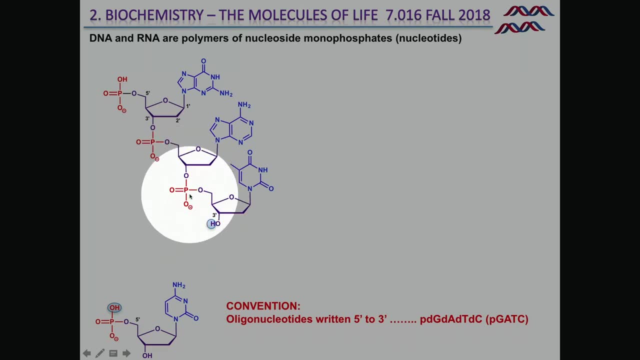 So the architecture of that nucleic acid is a polymer that includes a phosphodiester backbone linked by phosphate esters. that's one phosphate ester, that's the other one on two of the OHs of the ribose sugar. When this is DNA, there's no OH group at that carbon site. 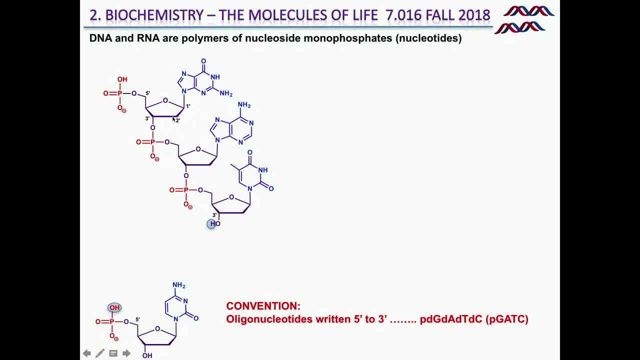 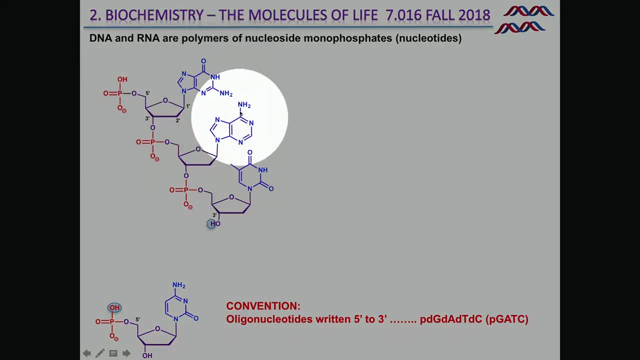 That would be the 2 prime site. You can see, you can pick straight out that this is DNA. The sequence is then defined by what the identity of the base is here. So this would be guanine adenine thymine. 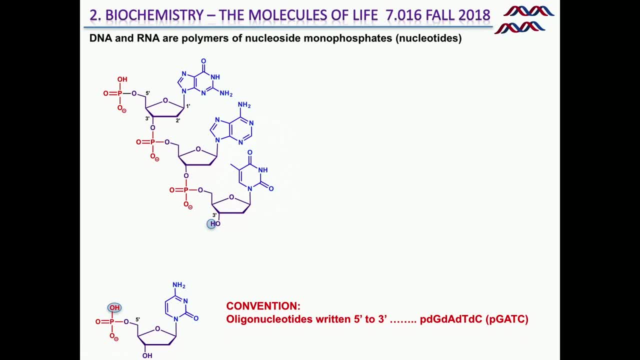 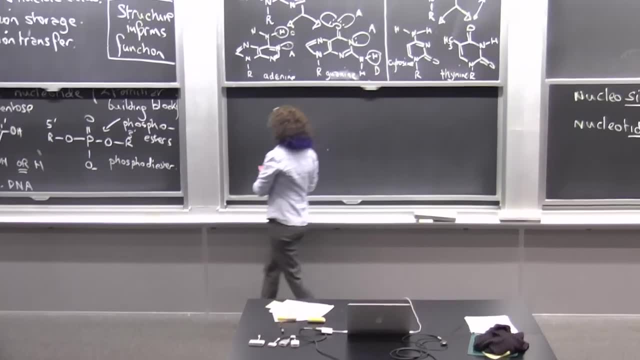 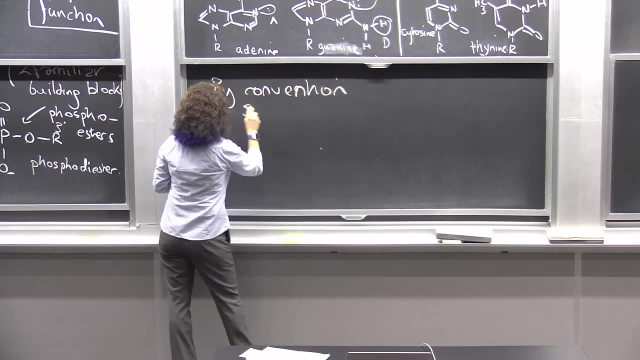 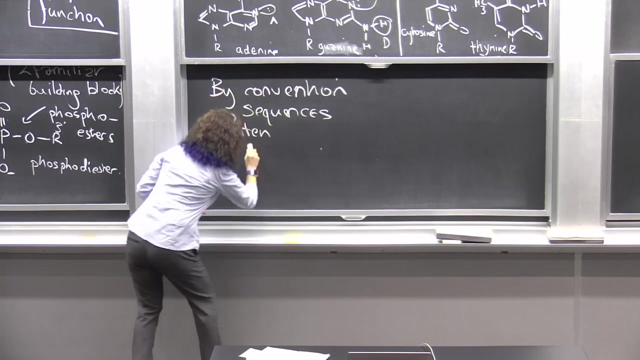 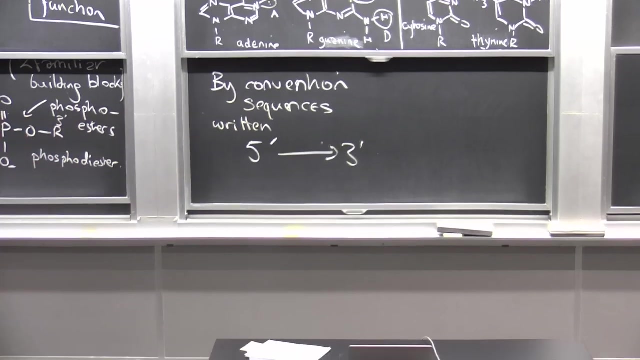 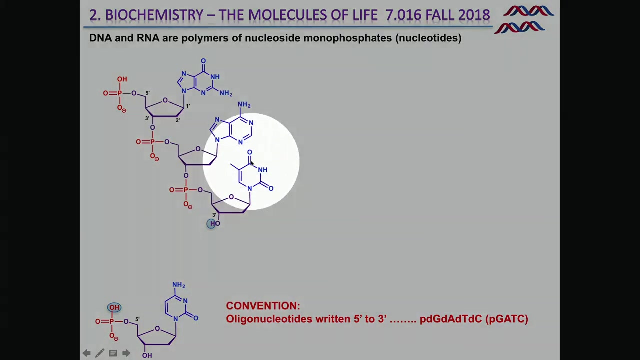 on that sequence. Now, by convention, if we write out this sequence, the way the sequences are written are 5, prime to 3, prime direction. So if I look at that I would be able to name it as an A-G-T. 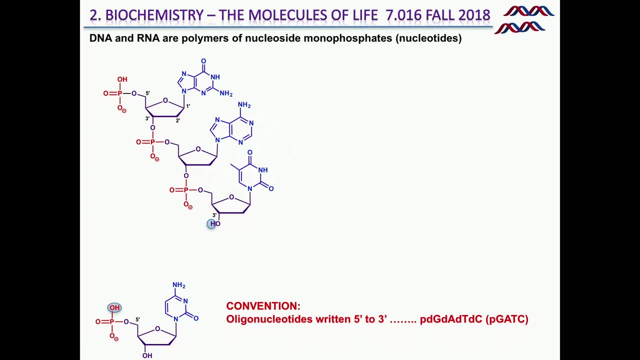 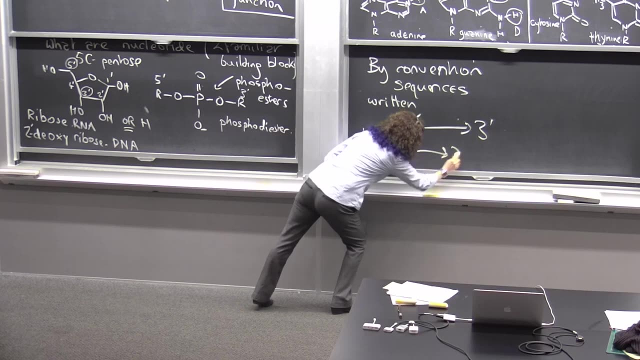 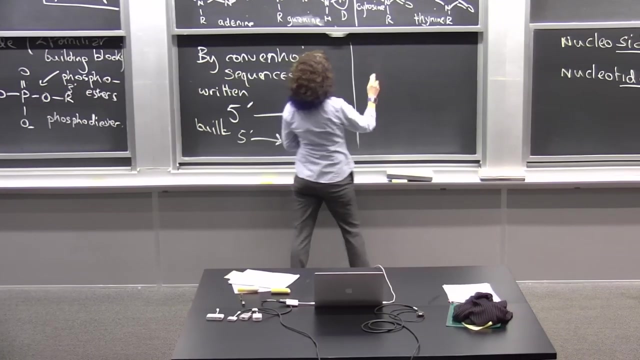 sequence, because we always write the sequences 5 prime to 3 prime. We can remember that later on because we actually also build sequences 5 prime to 3 prime. So there are some conventions in biology and biochemistry. You want to remember that by convention? 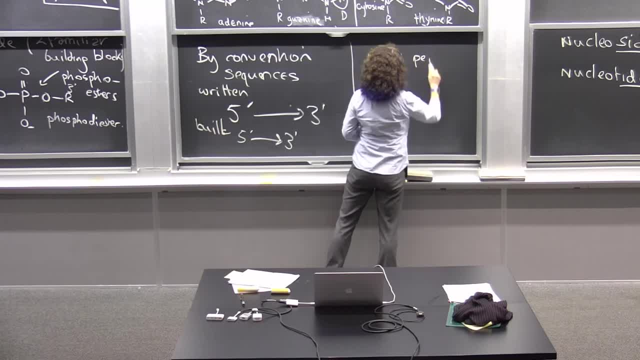 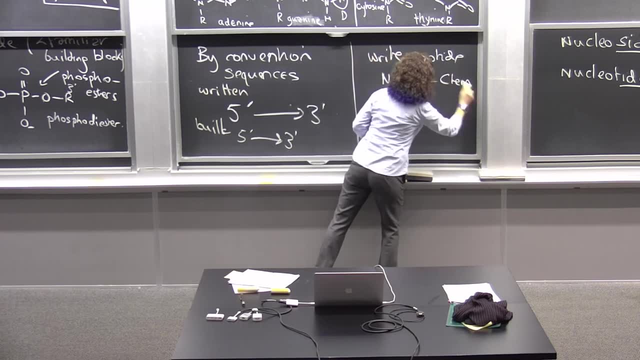 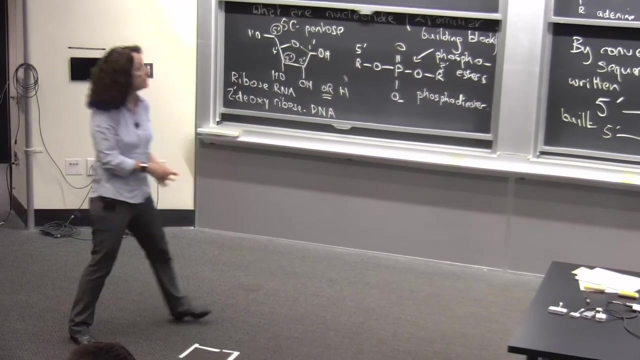 we write peptides N-terminal to C-terminal, but we also build them N to C. So that's why the convention is strong And it's good to remember, because it can get you out of a lot of trouble if you remember those things. 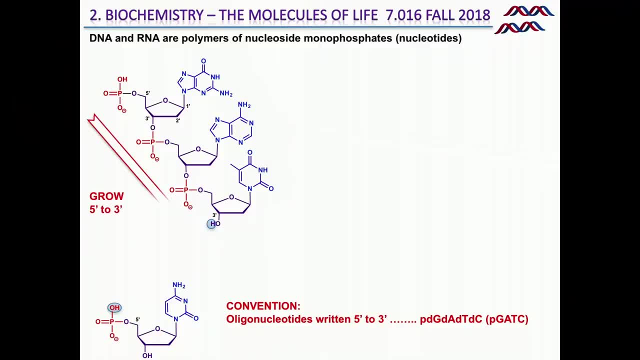 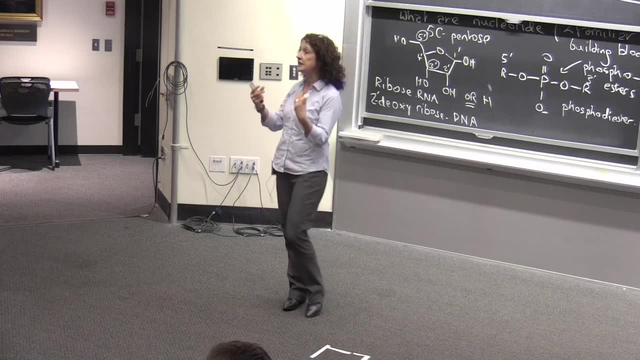 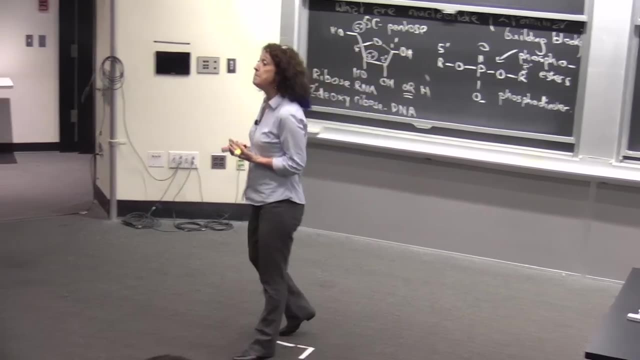 Now, when we are building a DNA polymer, we grow that sequence. You'll see the biochemistry for all of that polymerization in the next class. It's amazingly cool how the entire contents of a cell, the DNA, can be replicated. It's been replicated in amazing time frames. 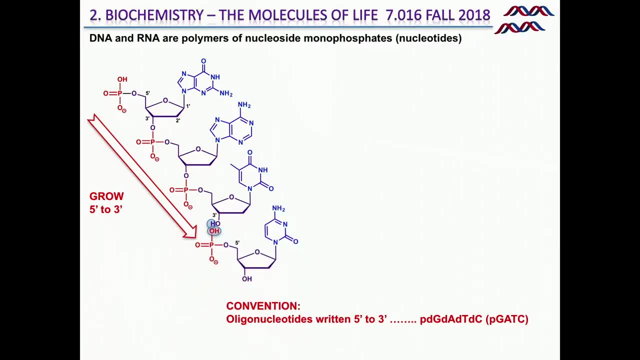 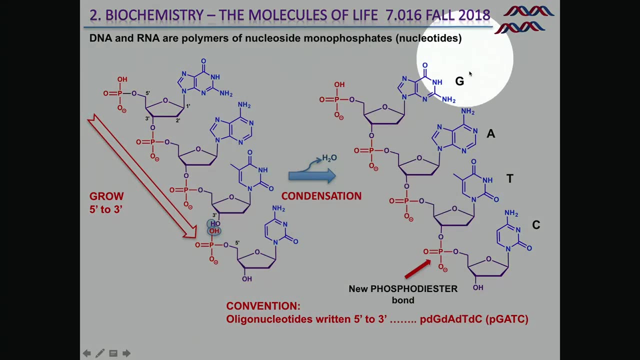 but all through growing those chains from 5 prime to 3 prime. So when we add another building block on, we remove a molecule of water, So that's a condensation reaction, And we form a new phosphodiester bond. So in the biosynthesis of DNA you 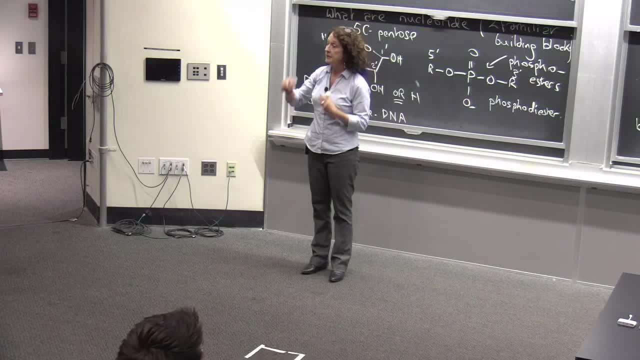 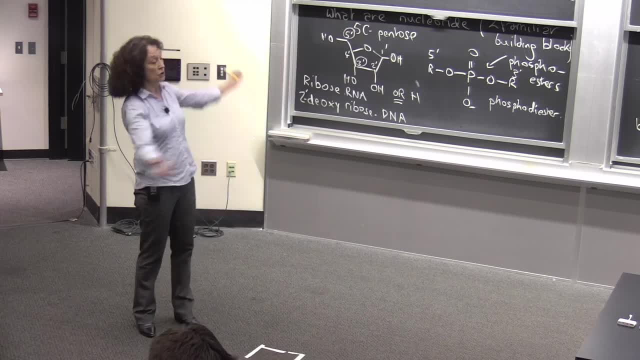 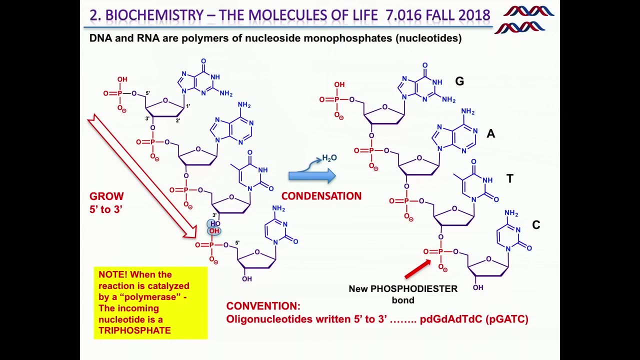 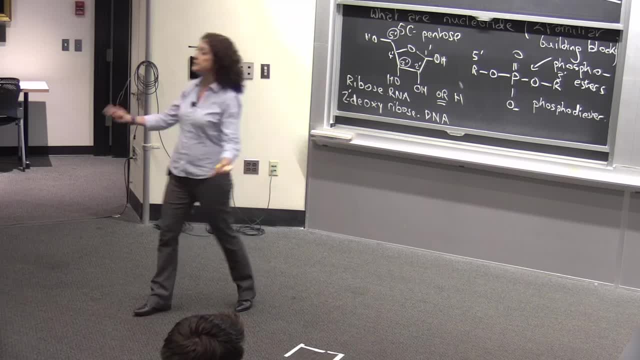 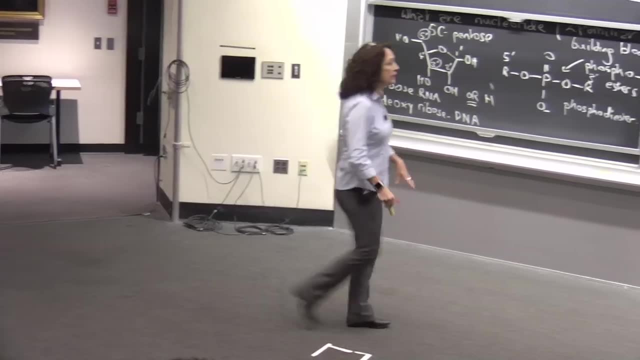 as the new building block And you kick out triphosphate And you'll see that when we talk about DNA synthesis. But what I want you to remember here is this is another condensation reaction. We talked about them when making peptides. We talked about them when making carbohydrates. 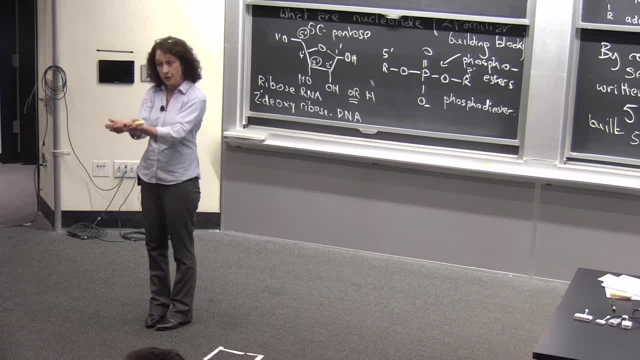 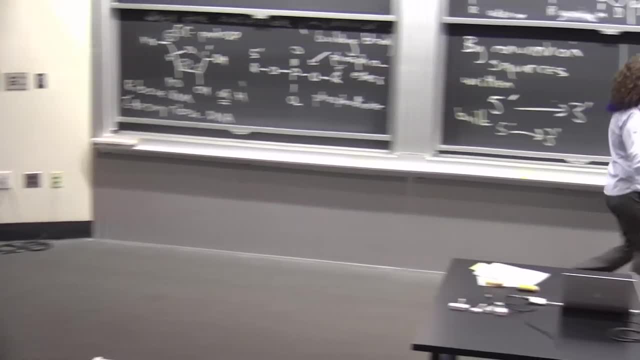 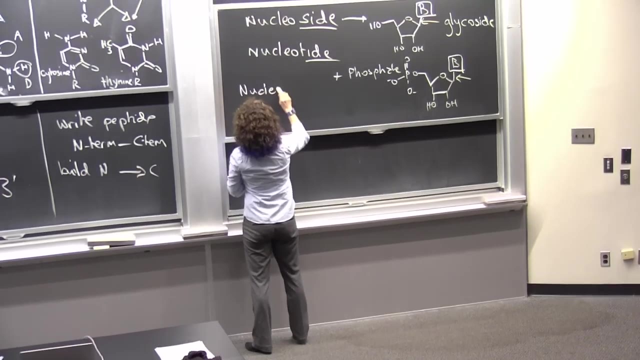 We talked about them when making substrate polymers, And now we're seeing once again a condensation reaction to make a nucleic acid polymer. Now, the last term that's kind of worth mentioning is the word nucleic acid. What's that about? 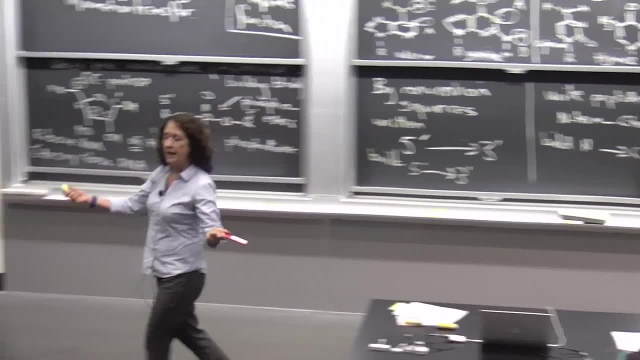 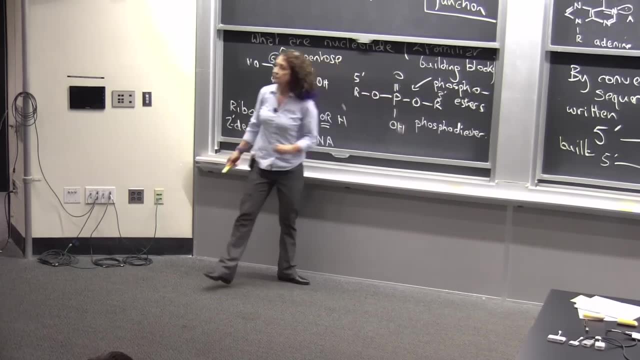 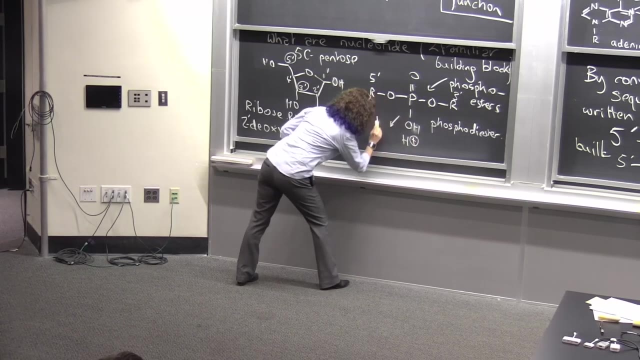 I don't see any carboxylic acids. It turns out that polymers of DNA are very acidic. The OH group on those phosphodiester backbones is very acidic. So you give up H plus And this is in its most stable form as O minus. 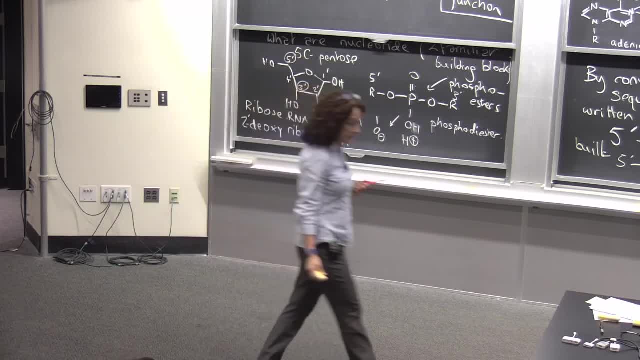 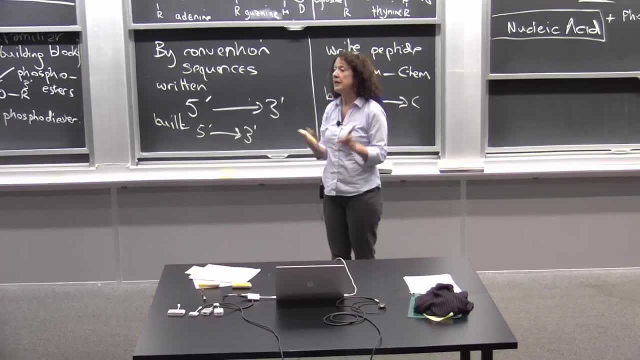 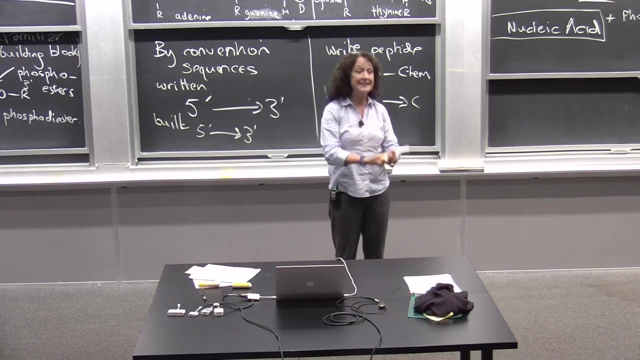 So when DNA was first isolated, it was isolated from white blood cells by isolating the nucleus And it was found that it was a very acidic material packed into the nucleus. That's why it was called nucleic acid- Nucleic acid acids in the nucleus. 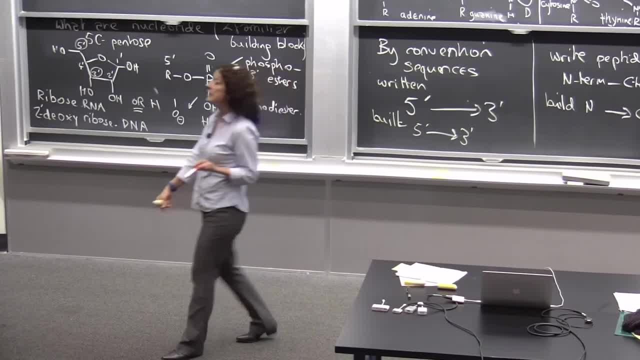 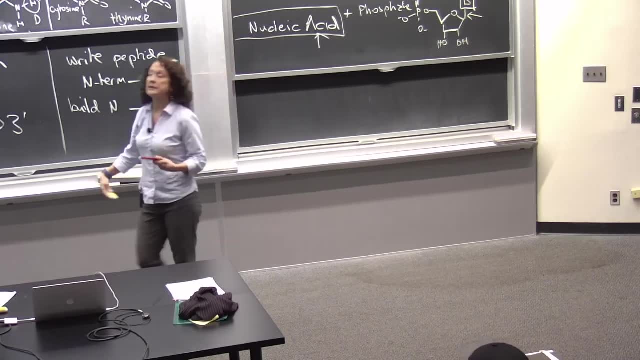 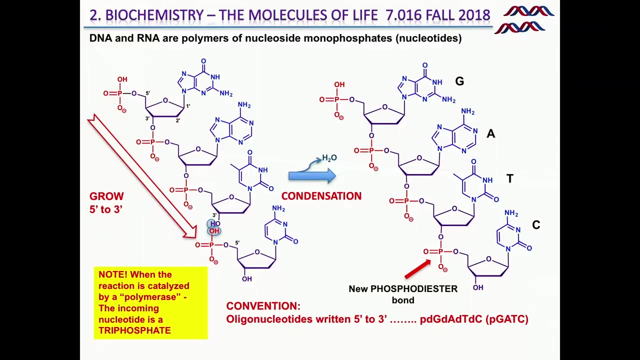 Before people even understood anything about the composition, it garnered that name nucleic acid. So when we talk about polymers of nucleotides, we call them nucleic acids. OK, All right. so then, with respect to writing our sequences, 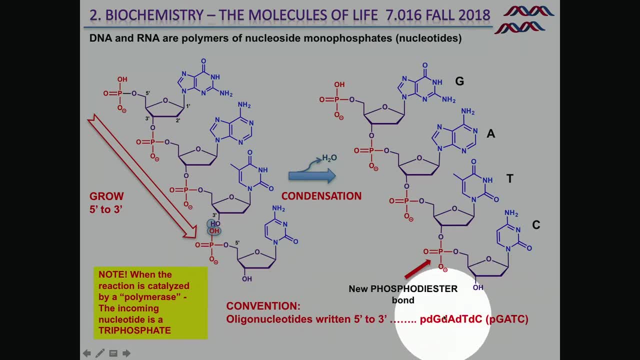 we could write them in this way, So P, D, G, A, T, C. That would be that structure. What do all the little extra P's and D's stand for? The P stands for whether there's a phosphate at this end. 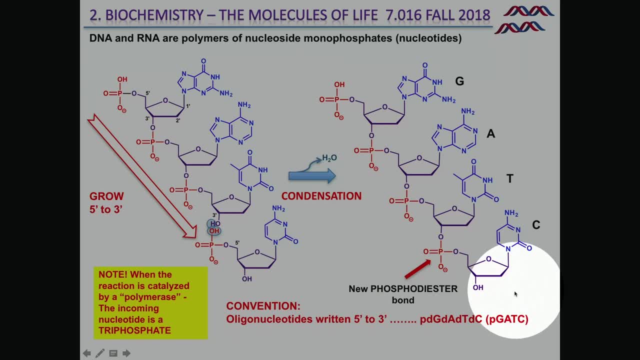 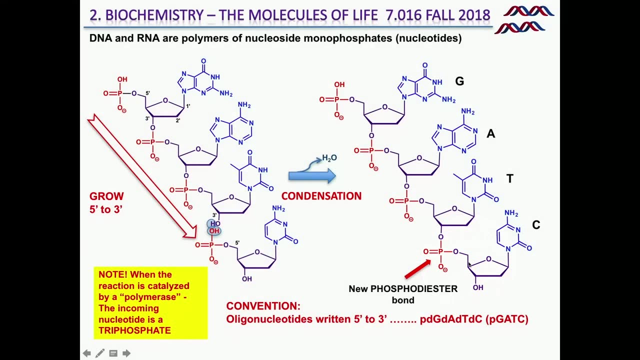 The D stands for whether it's a deoxysugar as a building block going all the way to the other end. There's no little P at the other end, so it means that OH is free. Does everyone understand that shorthand writing? 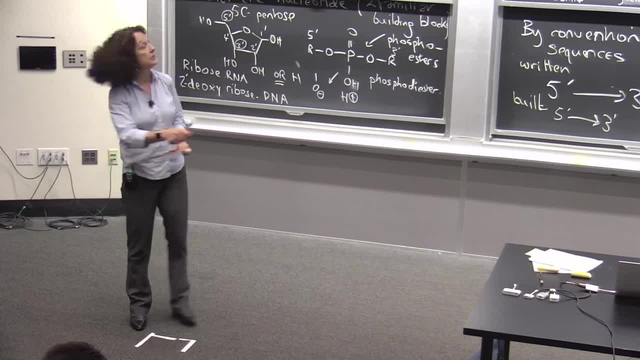 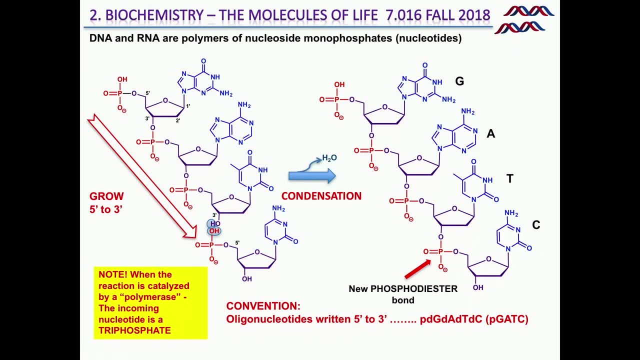 There's another way I could know this was DNA without needing to put deoxy on each of the the building blocks. Does anyone know how? I know immediately it's a stretch of DNA. Yeah Yeah, there's no uracil and there's thymine instead. 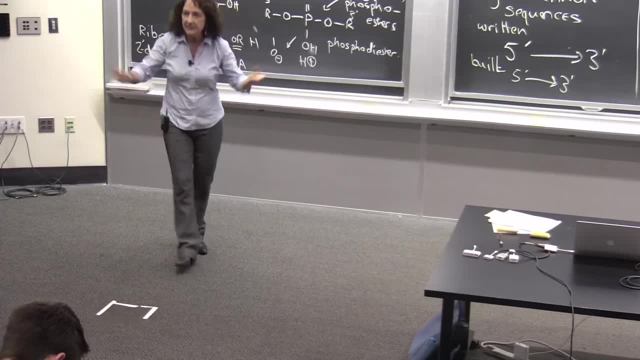 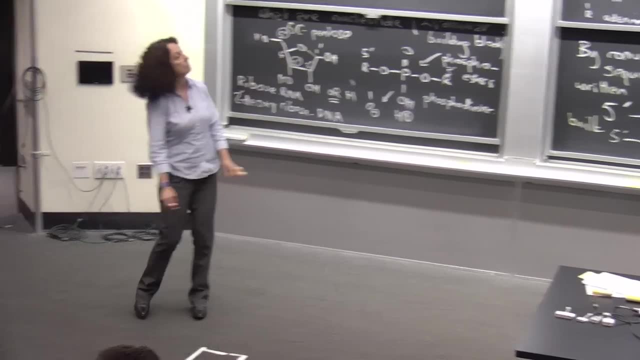 So, in the principle, as long as there's a T in there, you know it's DNA. As long as a U in there, you know it's RNA. OK, All right. now let's talk about the non-covalent structure. 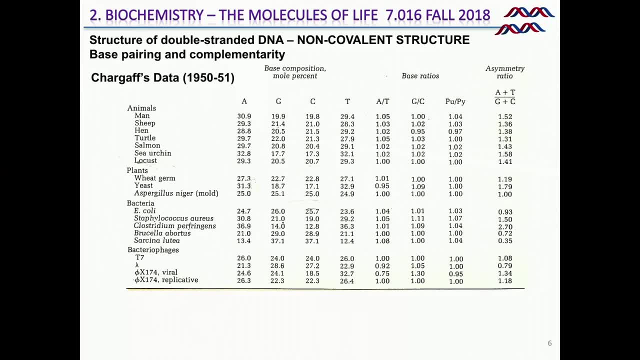 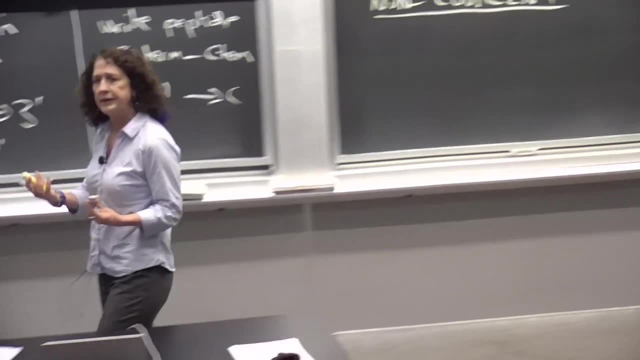 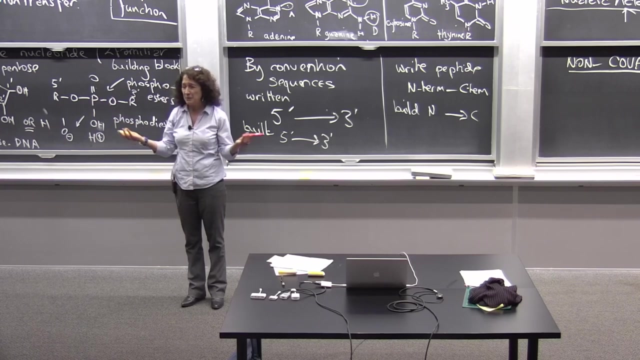 because I really feel that that's the most exciting part of this. I'm going to go through this entire endeavor Because the covalent structure really doesn't allow us to understand how DNA stores information for building proteins. It doesn't tell us that much about it. 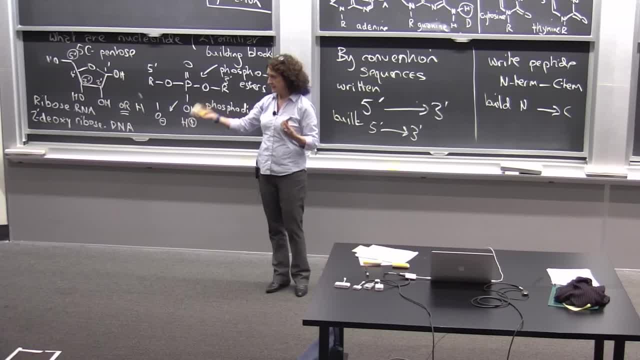 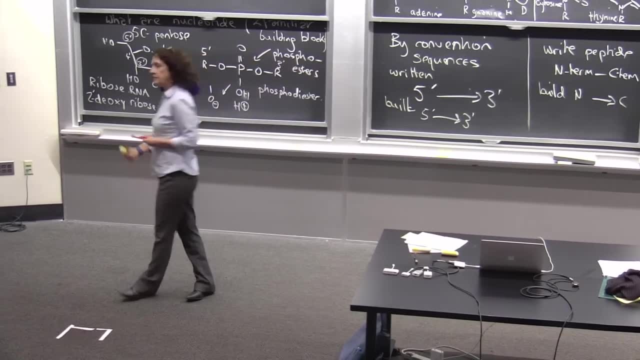 It just it looks like a cool polymer, but we can't really understand the details by not looking at the covalence of the non-covalent structure. So there was one key piece. There was a piece of information and it's called Shargaff's data. 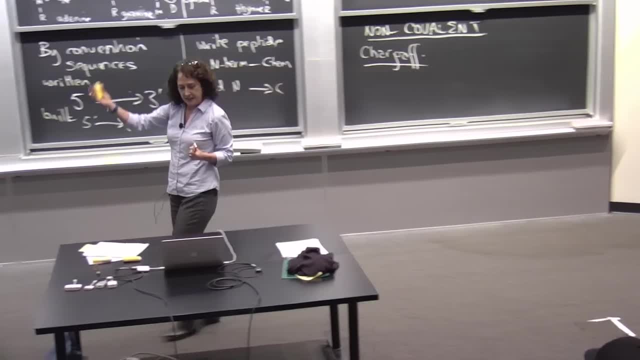 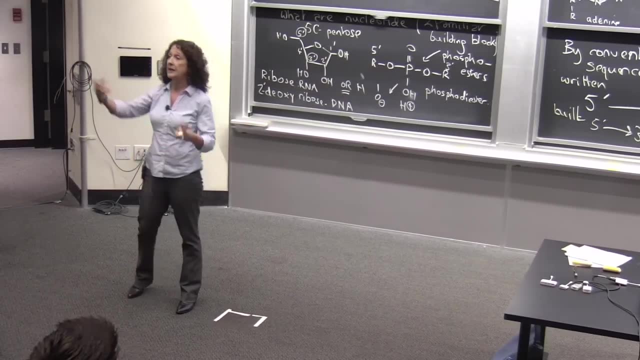 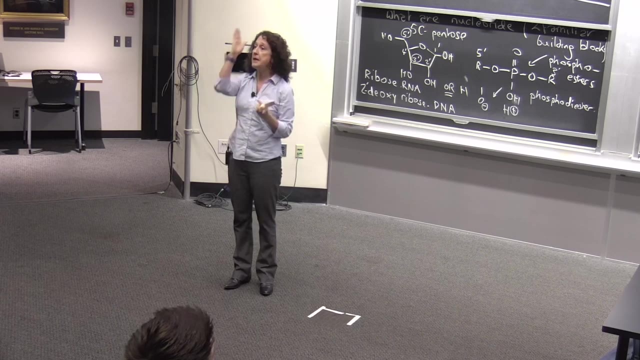 And this piece of scientific information ran around the scientific community in the early 50s because it seemed incredibly important. And what Shargaff's data was? he collected all kinds of organisms and then their nuclei, and then measured all their DNA and then measured the ratio. 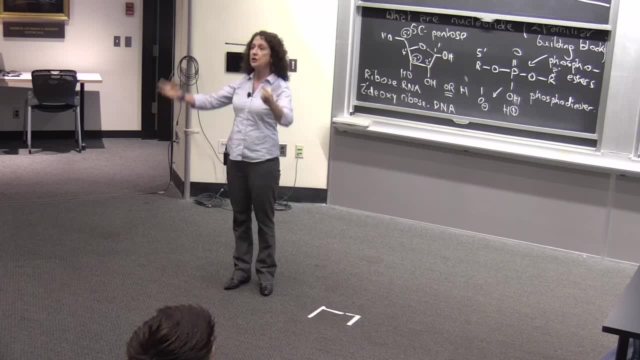 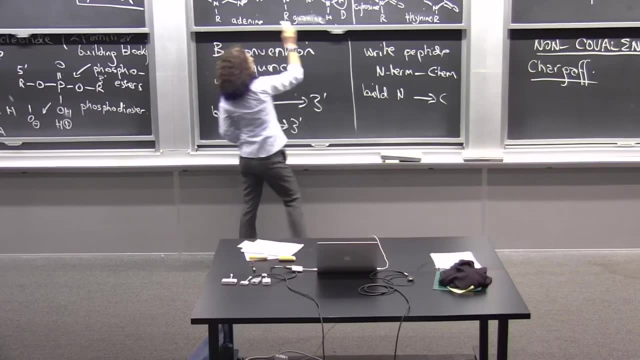 between the purees, OK. The purines and the pyrimidines, OK. He measured the ratio of the large ones and the small ones of the nuclear bases, So how many of these relative to how many of those, OK. And what he found by looking all across organisms. 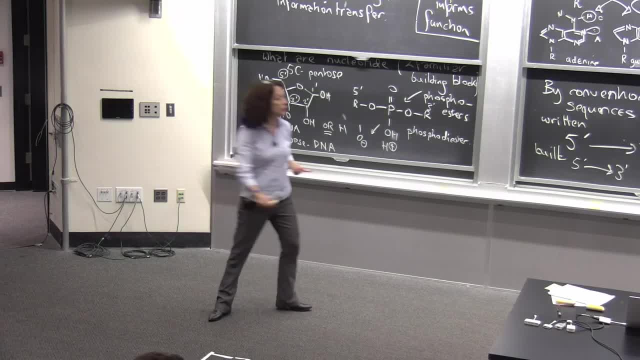 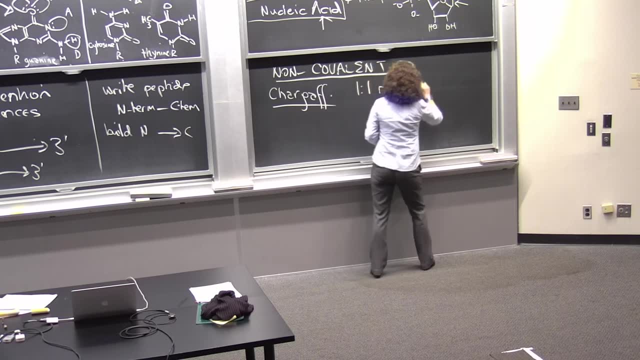 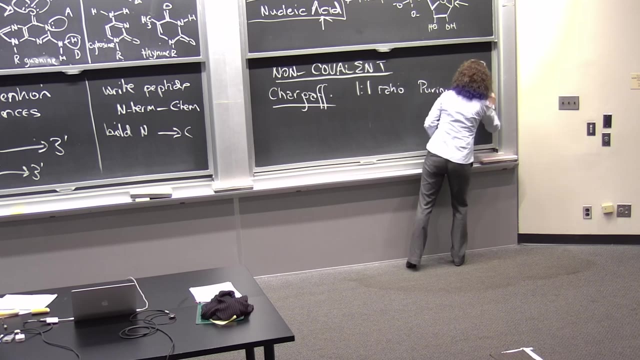 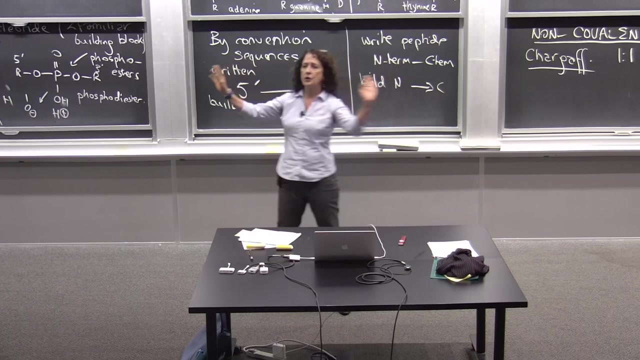 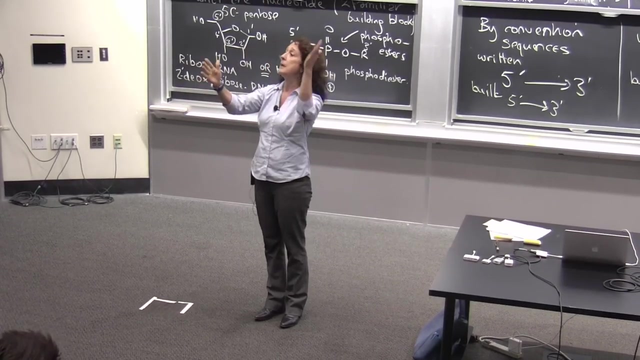 from all domains of life is that there was a one-to-one ratio of purine to pyrimidine And he found that the number of purines and the number of pyrimidines was the same. So that became very interesting, because what it suggested- 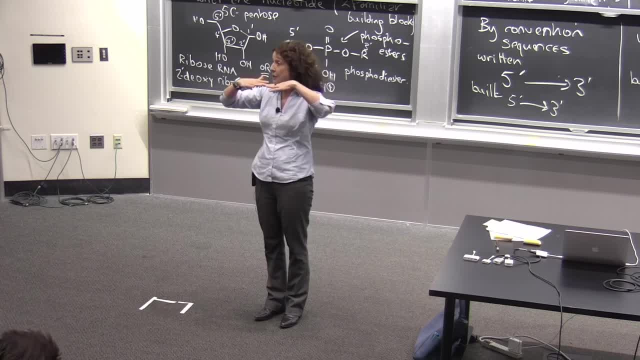 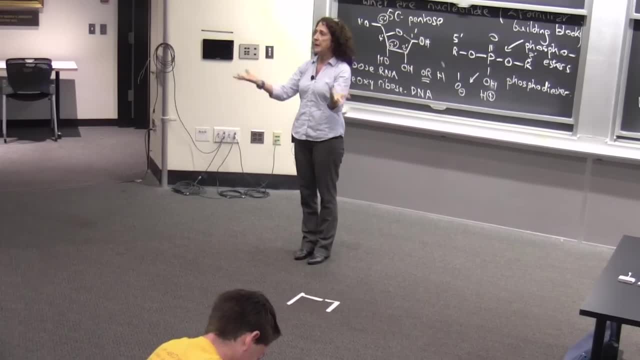 was that in some way the non-covalent structure of nucleic acids had some correlation between the number of the purines and the number of the pyrimidines, And it's like the light bulb that went on with respect to understanding the structure of double-stranded DNA. 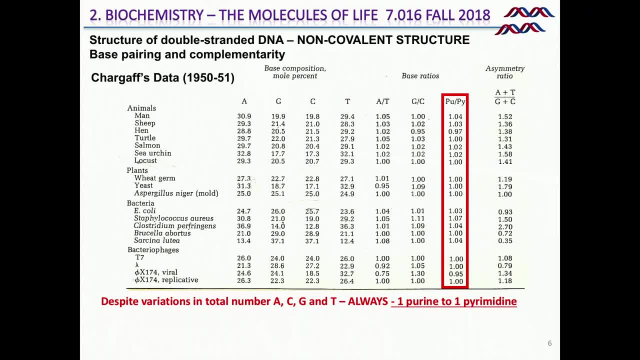 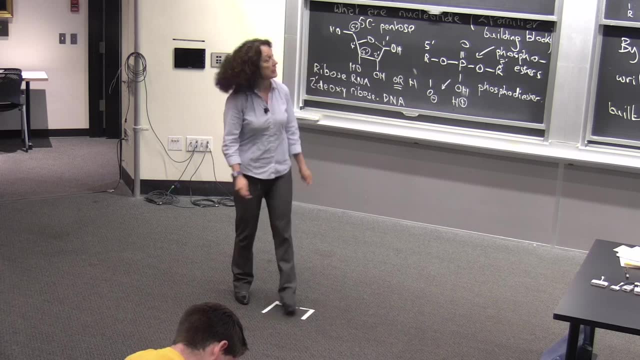 So, despite all kinds of variations, some organisms have a lot more GCs, Some have more ATs, But no matter what, the ratio is always one-to-one, And this ultimately led to understanding the non-covalent structure of double-stranded DNA. 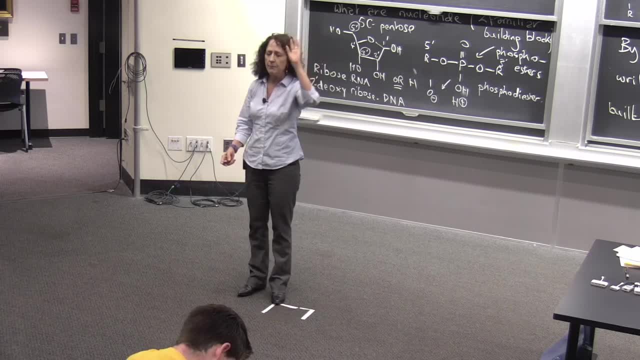 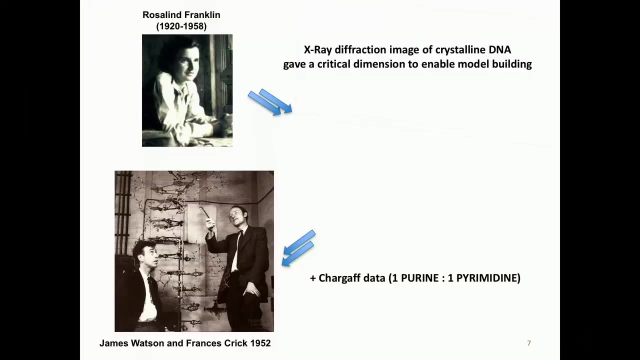 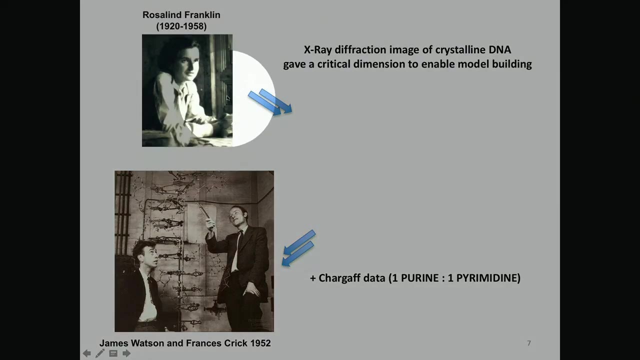 because it provided clues to how they're going to work And how there could be some way that information was coded but then could be replicated. Now the next thing that became the clue to the structure of double-stranded DNA came from a very talented researcher, Rosalind Franklin. 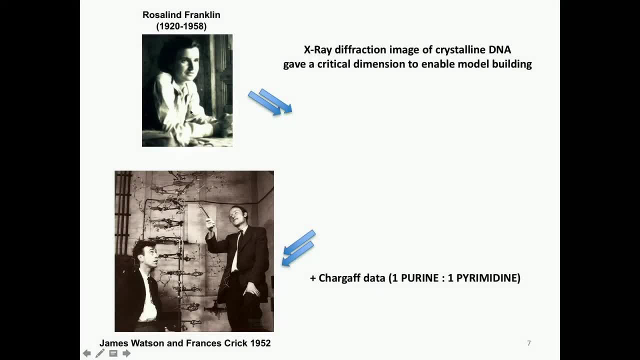 who sadly died way before her time of ovarian cancer, Really in large part because she spent a lot of time near x-ray beams, So that would have caused mutations to her DNA And she developed a very complex DNA And she developed a very complex DNA. 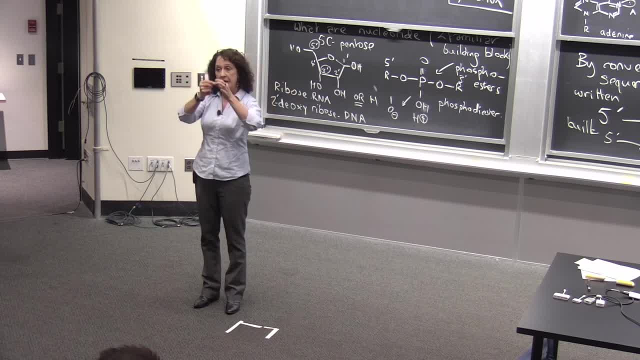 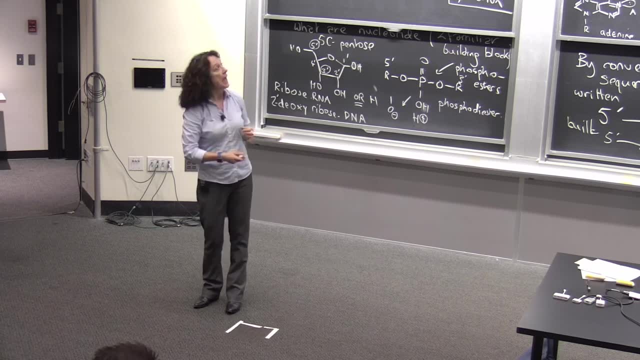 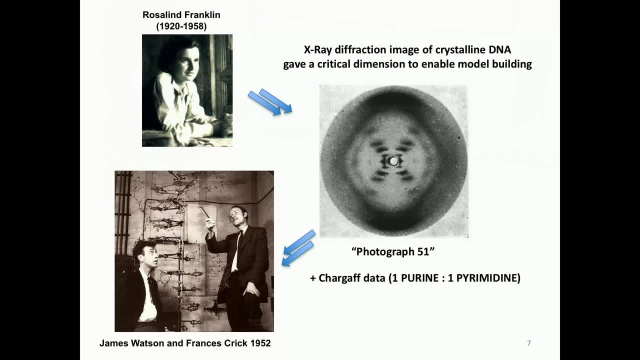 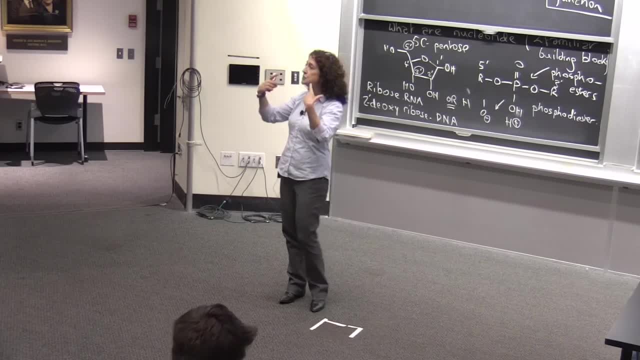 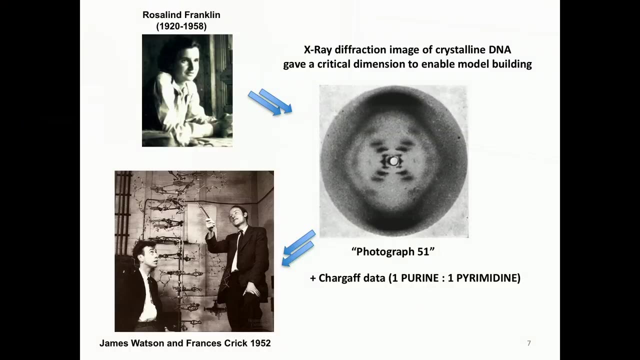 stranded DNA structure And it actually was the clue that told the spacing between the strands of DNA. So it really was a piece of information that you simply couldn't do without. With Shargaff's data and with this what was called Photograph 51,, it really gave you. 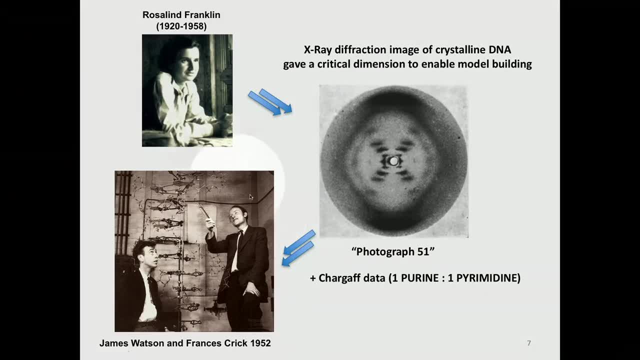 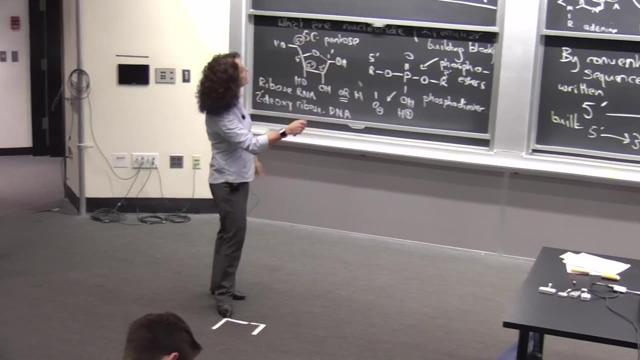 the clue, And it was really during those years that Watson and Crick were desperately model building to try to understand the non-covalent structure of DNA, And once they had those two pieces of information, they could actually put together hand-built models. 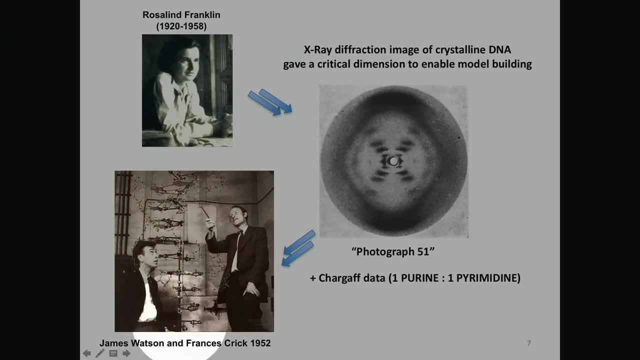 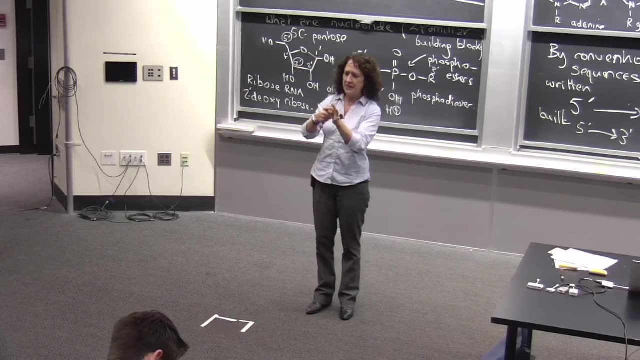 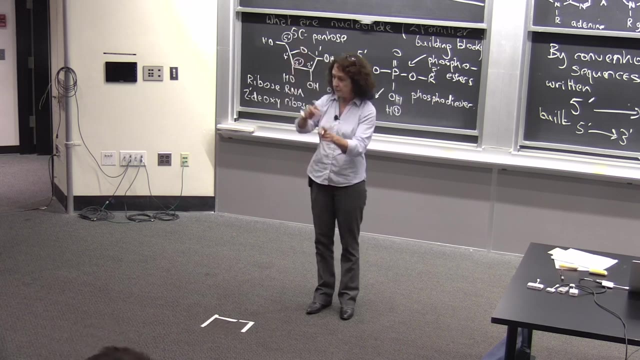 This looks kind of clunky but I know the room they took this photo in from my years at Caltech. in fact I can recognize the room. They built not just little tiny molecular models but big molecular models so they could make measurements. to say, the diffraction data told me this was so many nanometers apart. 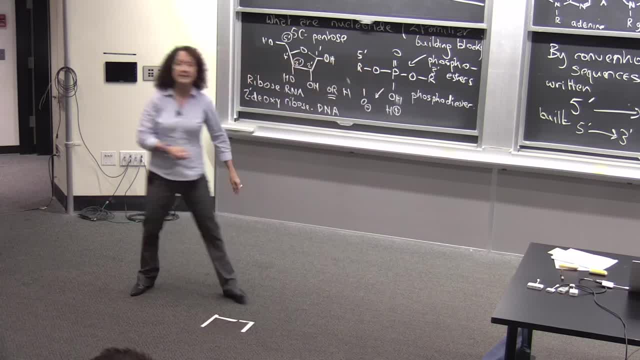 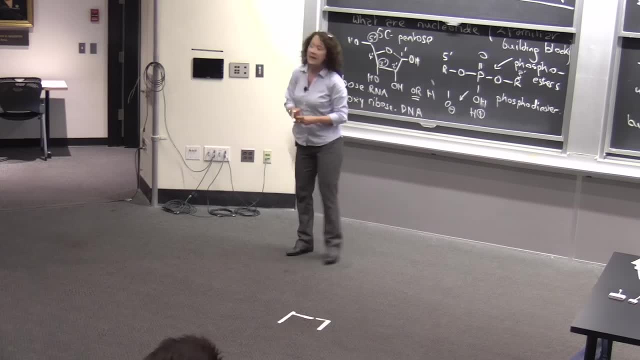 and they were able to piece together the structure of double stranded DNA, But I still haven't shown you how those two strands come together. It's really intriguing because at that very same time, Linus Pauling had done very well with the structure of the algorithm. 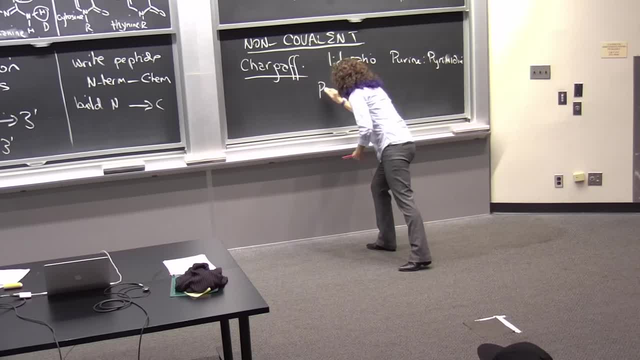 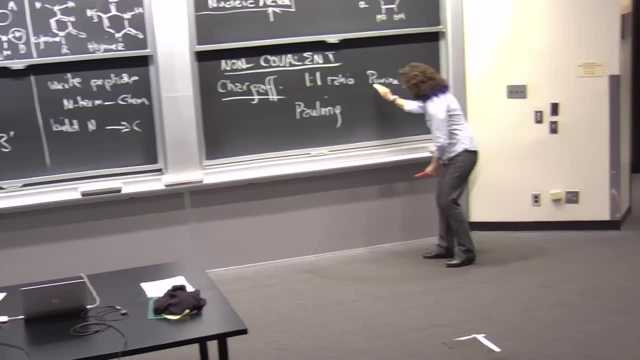 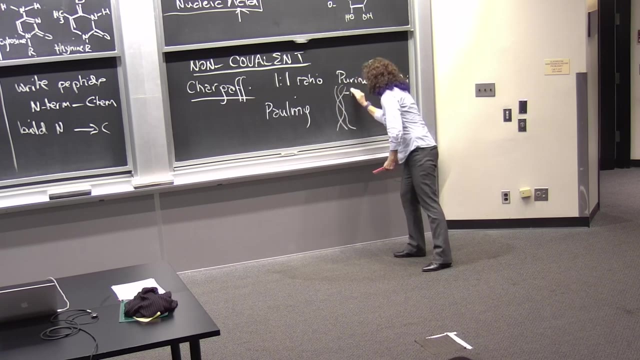 He looked at the structure of the alpha helix in proteins Also was trying to figure out the structure of DNA. But he came up with a sort of a crazy structure where he thought that it was a triple stranded structure where the bases actually stuck out. 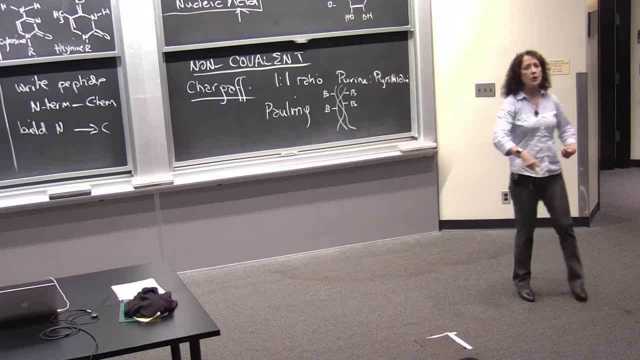 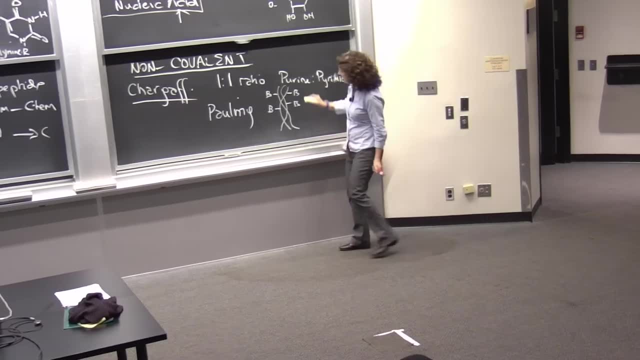 And somehow this triple stranded structure coded for replication of DNA. Now, there's a ton of things that are really awful. There's a ton of things that are awful about this structure. First of all, it's a triple stranded. But the other terrible thing is there's so many phospho-phosphates in the backbone there. 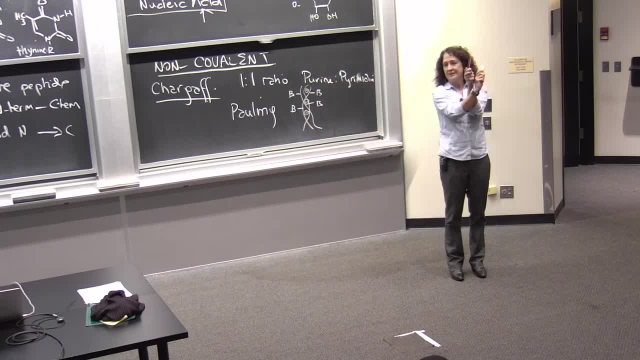 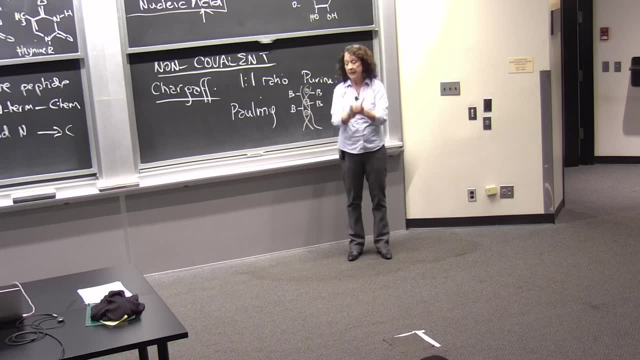 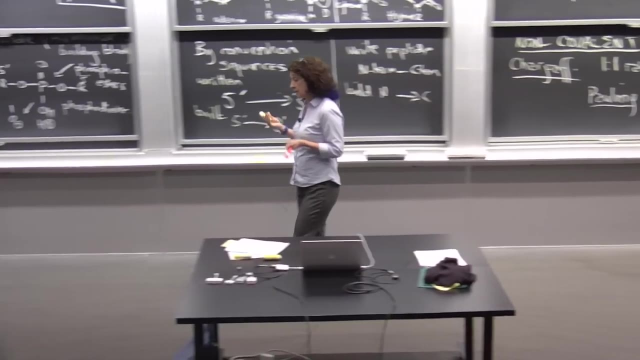 would have been massive electrostatic repulsion. Those sequences would want to blow themselves apart, because you can't cram that much negative all in one place. But it was really an intriguing sort of sociological phenomena. at the time Pauling was a major pacifist. And he was really, really active. He was very active in nuclear disarmament And they said that his mind just wasn't on some of this stuff and that this model came out of him really worrying about other things and not focusing on the DNA structure. 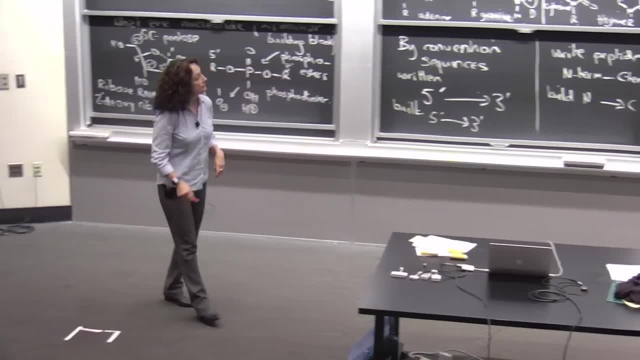 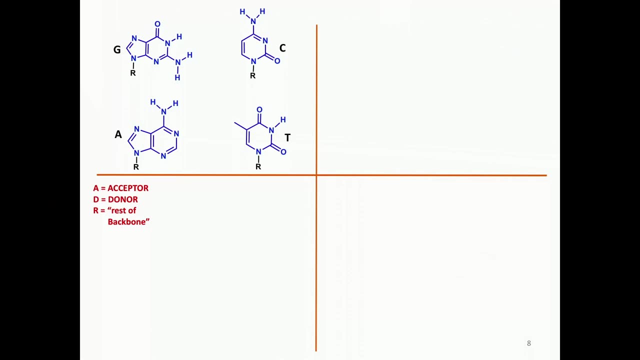 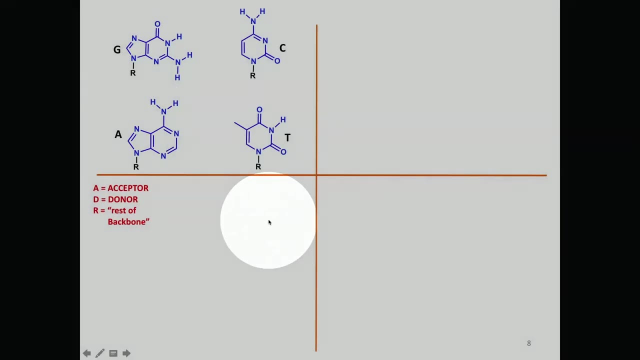 So let's try to explain Misha Agaf's data by looking at the nuclear bases and thinking about how they might come together. So here I show you the structures of the four nuclear bases in DNA. Wherever I have an R you can assume. 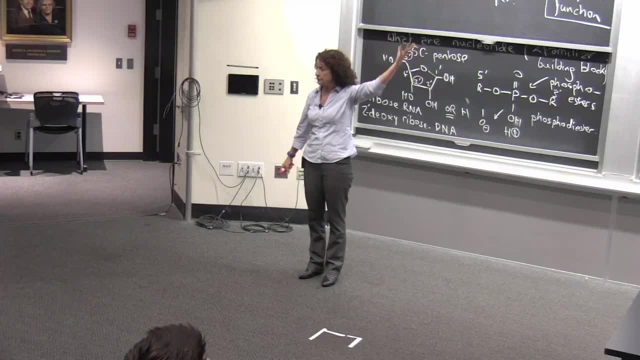 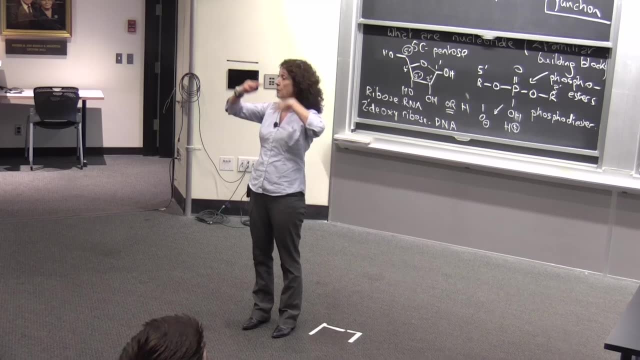 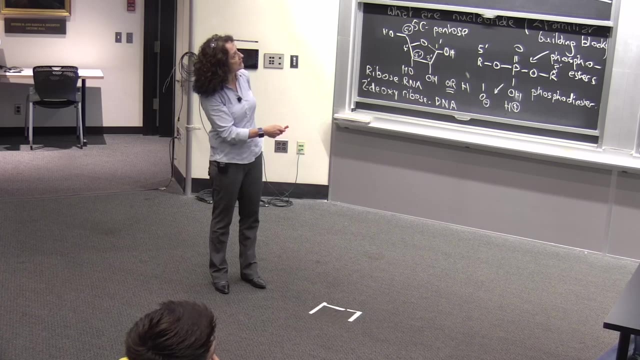 That's part, That's a ribose, that is part of the phosphodiester backbone. What we want to understand is how do the nuclear bases come together to form some kind of pair that could be useful to programming their resynthesis? So I've drawn them all here, but it's not quite intuitive. 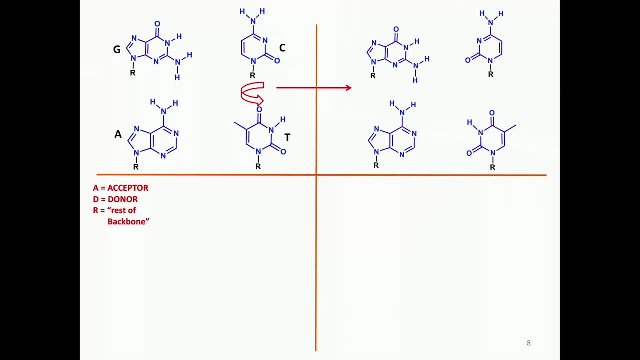 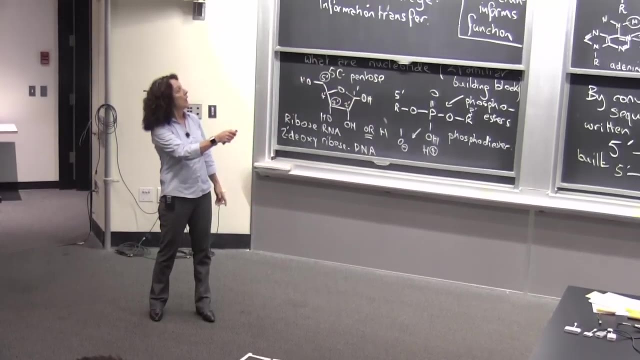 I need to do a little bit of flipping around to line things up better, And the other thing I need to do is get things at the right angle so you can start seeing how those bases move, How those bases might come together, Because Agaf's data dictates that you have a purine and a pyrimidine: purine- pyrimidine. 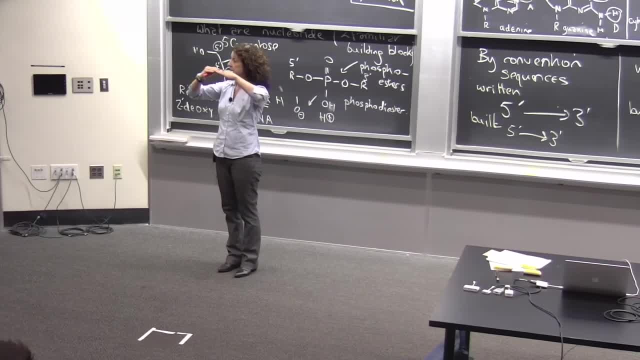 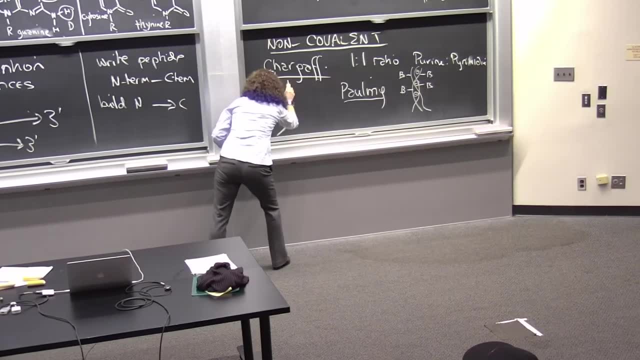 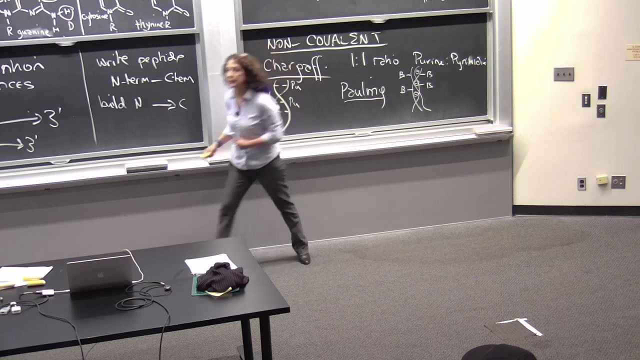 You have pairing between the nuclear bases in your double-stranded DNA in a structure that looks more like this, And in each case you've paired a purine and a pyrimidine. So what I want you to do is take a look. 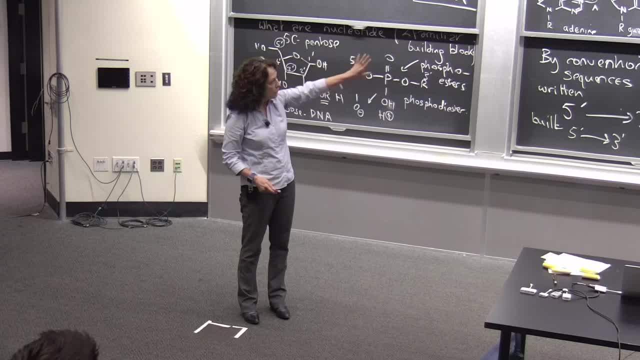 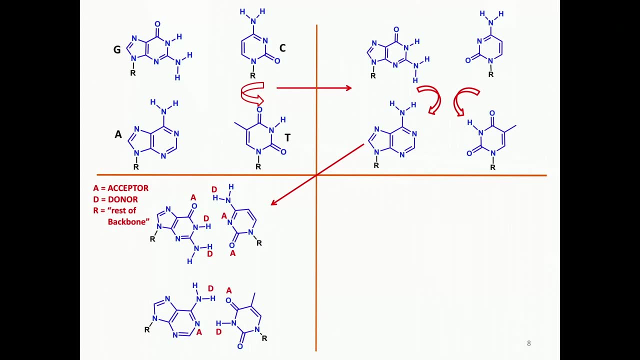 I've shown you now where donors and acceptors are. You can go back and do this for all the nuclear bases, but I'm going to do this for you right now by showing you the donors and acceptors of hydrogen bonds within those structures. 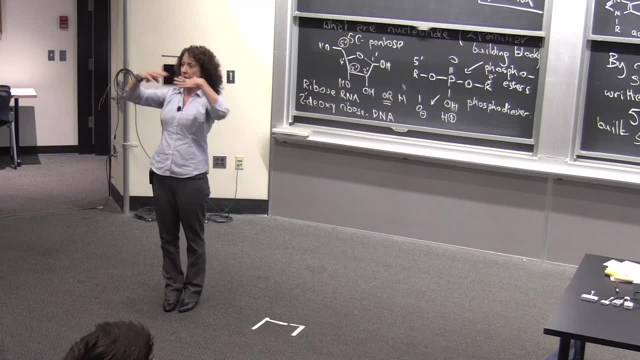 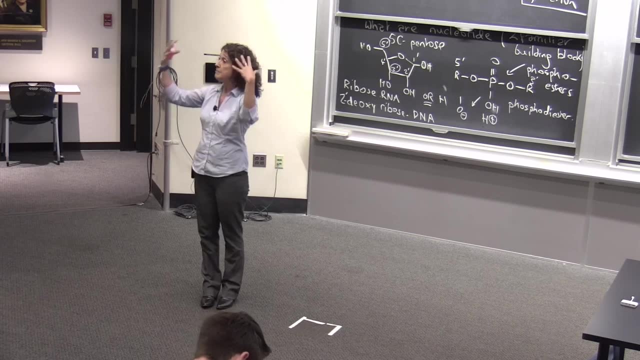 What I've done is I've lined them up beautifully so they look straight at each other, So you can tell that there is a complementarity Between a purine and a pyrimidine. that makes very nice hydrogen bonding, which is the non-covalent force. that's very important. Between G and C, I can set up three hydrogen bonds. Between A and T, I can only set up two hydrogen bonds. So one purine is complementary to one of the pyrimidines. One purine is complementary to one of the other pyrimidines. 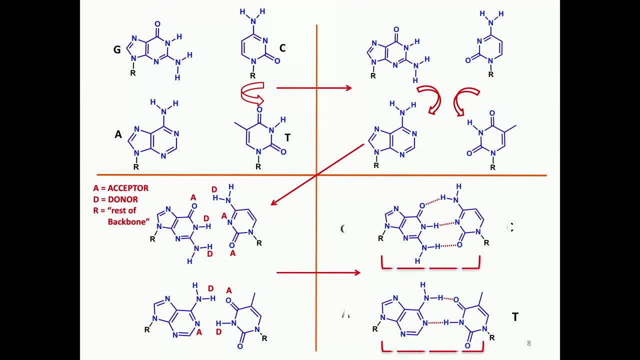 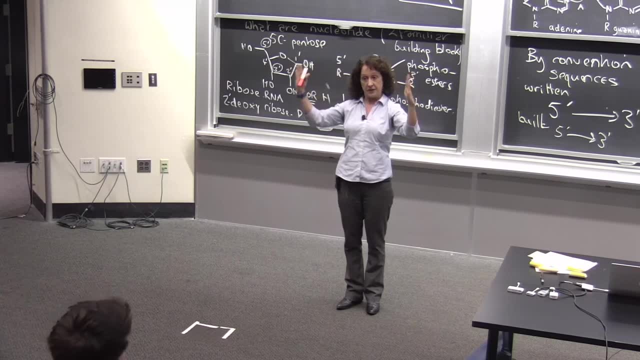 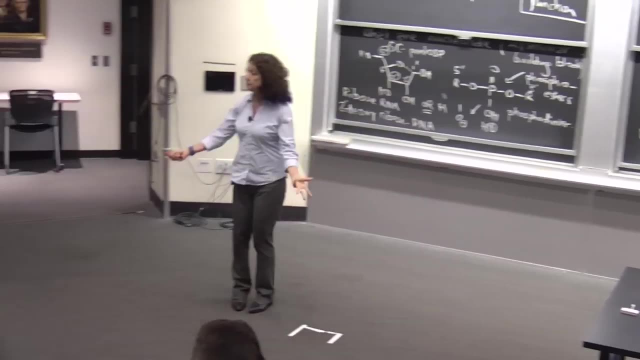 And then we can draw those hydrogen bonds in place. That totally explains the measurement from the Franklin data of the distance, the width of the double-stranded helix, because it's identical for both of those base pair options, And that gives you the structure that forms the non-covalent structure of DNA which is 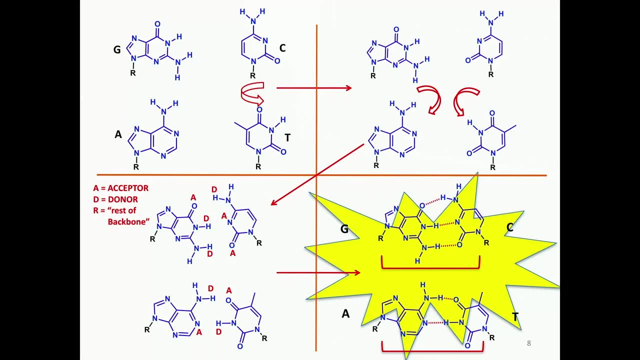 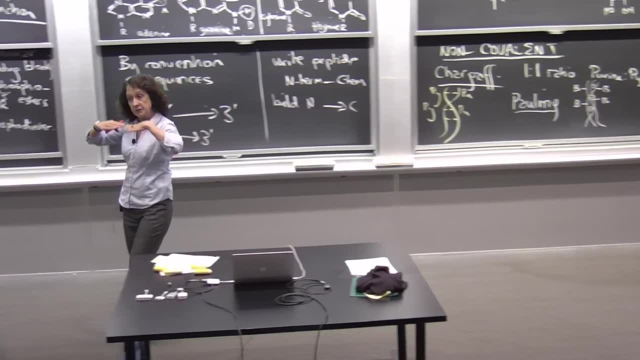 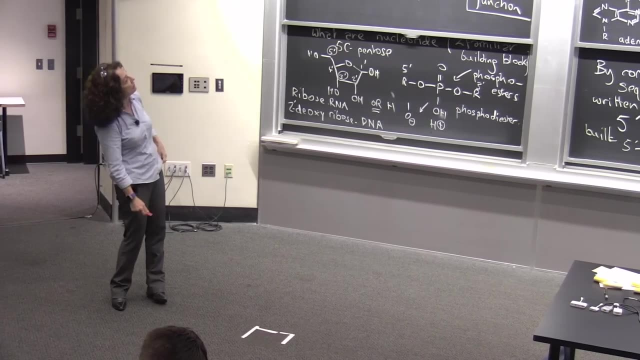 a series of interactions where the solid line is the phosphodiester backbone but sticking out like steps on a spiral staircase. The base is where each base is complementary to a specific additional base, So it predicts the Shar-Gaff ratio and it also predicts the distances. 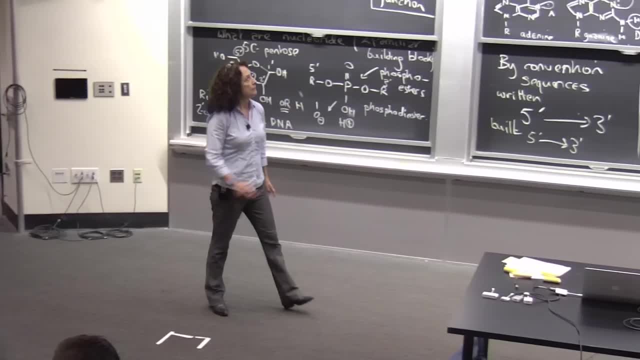 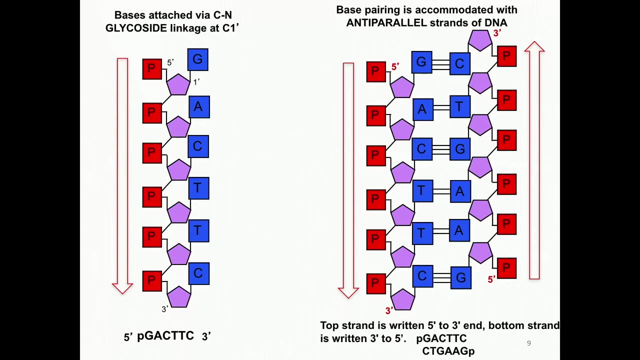 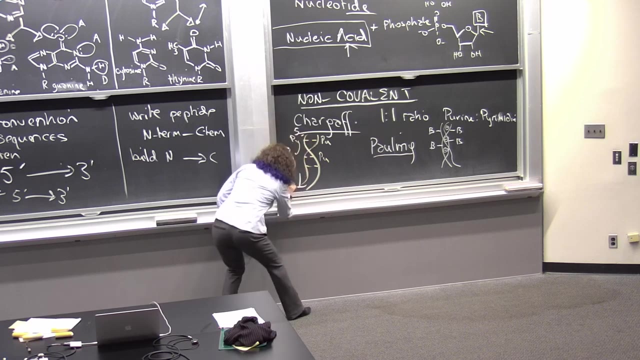 Now, within all the model building, it became quite clear that the structure, the non-covalent structure of DNA, was afforded by anti-parallel strands, where one strand went in one direction- 5 prime to 3 prime- And the other strand went in the opposite direction- 5 prime to 3 prime. 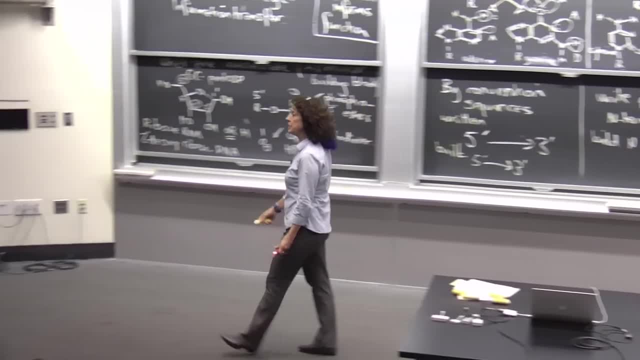 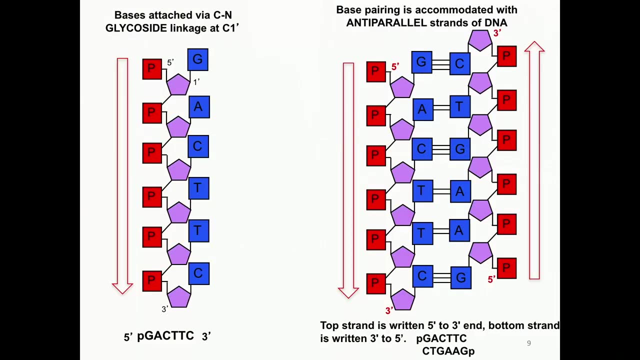 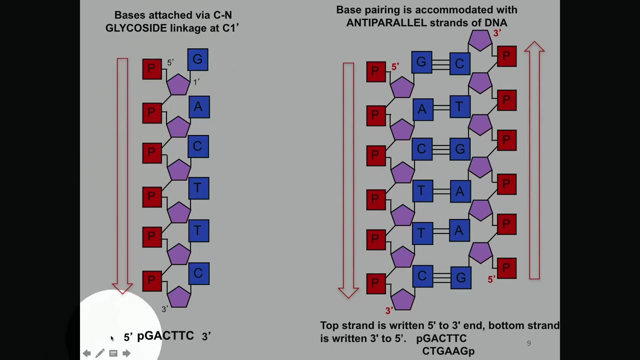 When we start replicating DNA we're going to see that that's pretty convenient, But thermodynamically it is also the favored orientation. So let's just look at the orientation where you would draw one strand of DNA: 5 prime to 3 prime. 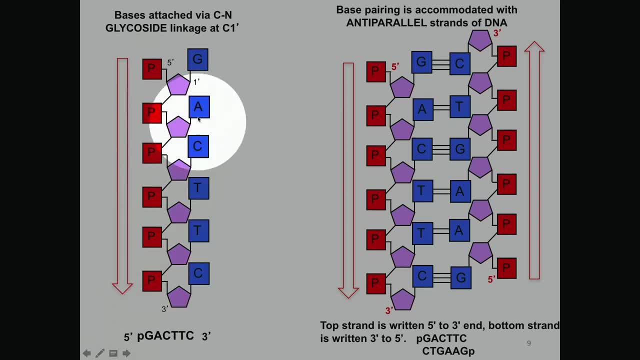 Now I've taken this all down to cartoon level. These are the phosphate diesters, The riboses, The 3 prime end and the 5 prime end And the bases that come off at the 1 prime carbon. And then, when you pair it with another strand, one strand goes in one direction: 5 prime. 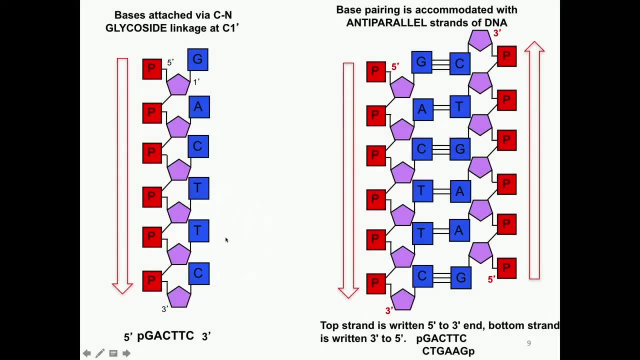 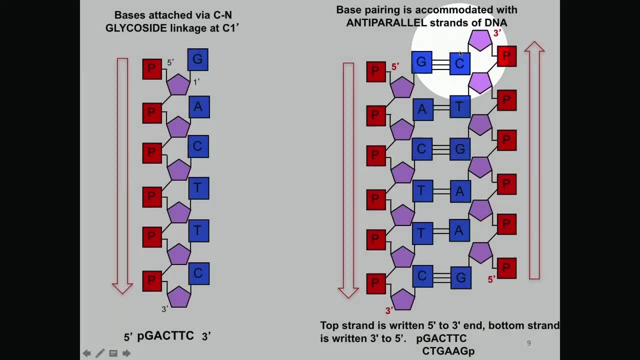 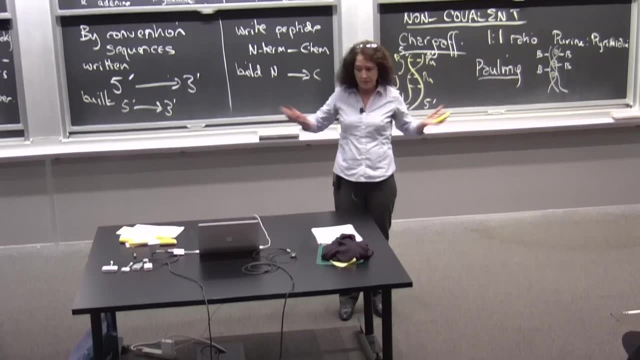 to 3 prime. The other strand goes in the other direction: 5 prime to 3 prime, And when asked this question a few years ago I couldn't really explain it very well that I just said it had to be because it always has been. 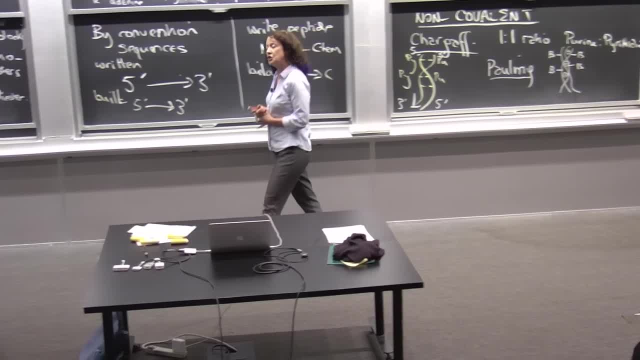 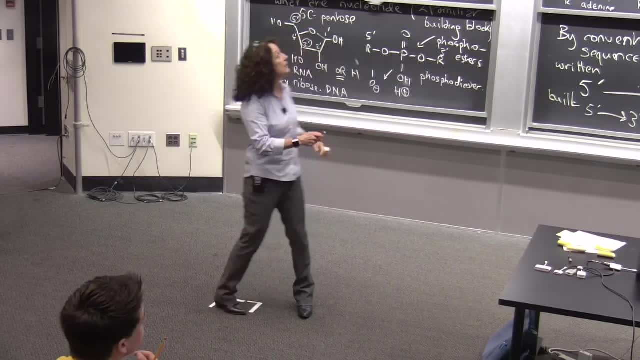 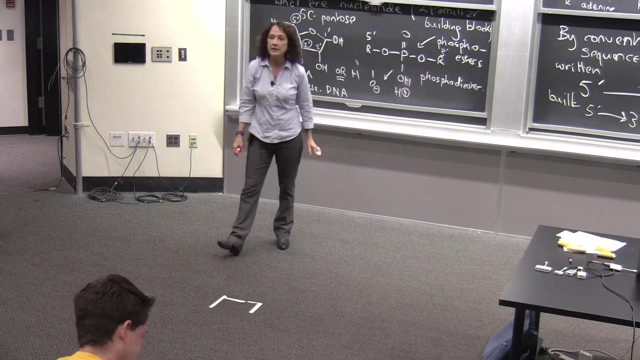 But what's really cool is if people have been able to solve the crystal structure of a parallel pair of DNA strands. So this is canonical DNA, the beautiful anti-parallel structure, And it's very regular, very, very even. It turns out, though, when you try to pair the two strands in a parallel orientation. 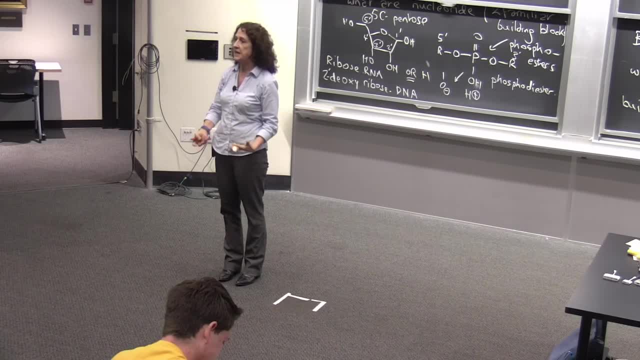 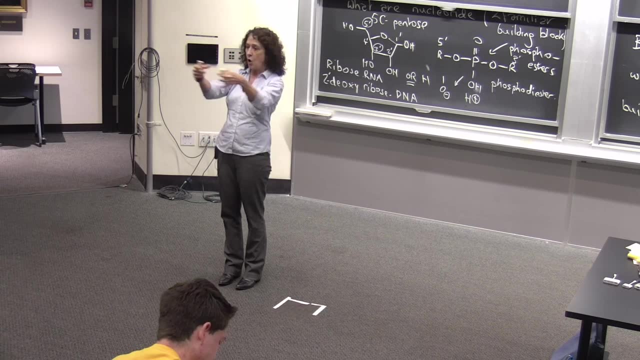 they're very uncomfortable And it's much less stable. So the anti-parallel orientation is very important for the thermodynamic stability and the optimum hydrogen ponding interaction of all those bases that are pairing. So it's actually what nature favors, because it is more stable. 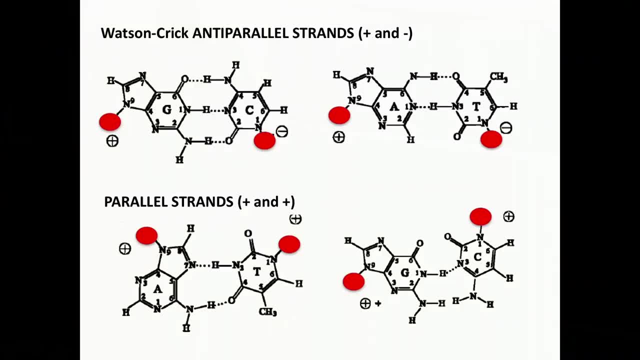 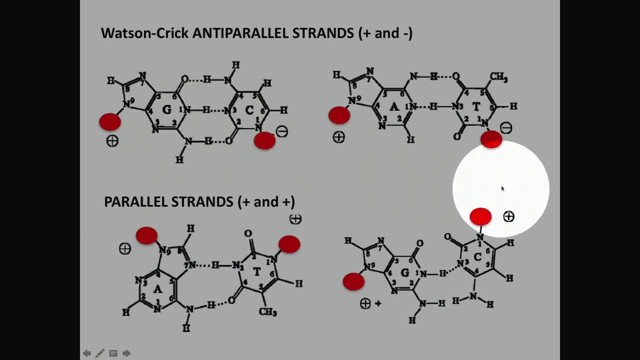 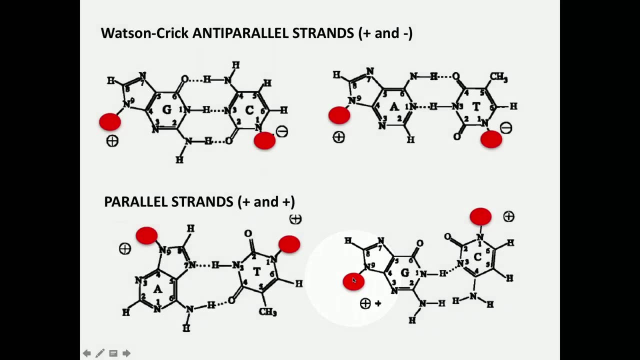 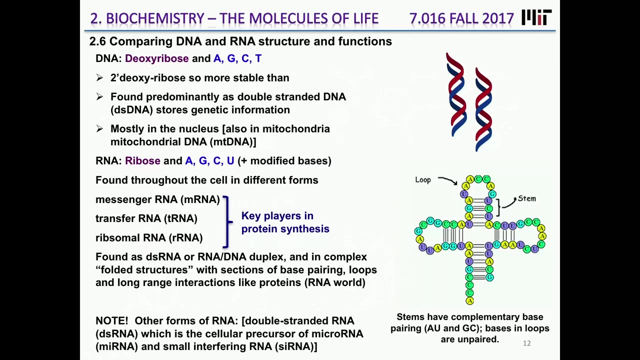 Any questions? OK, And it's on your slides, but you can see just how regular DNA looks so organized, whereas the anti-parallel one, The parallel one, really does not afford you good hydrogen bonding interactions at all. OK, So let us now. 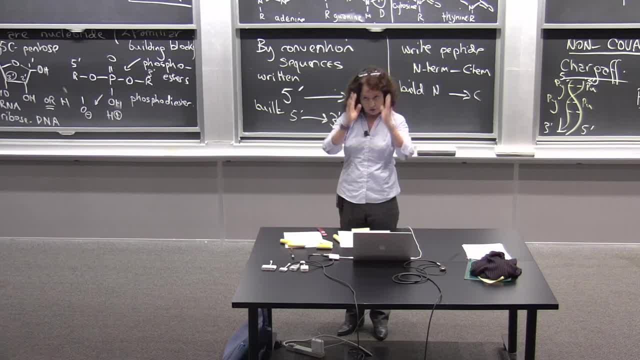 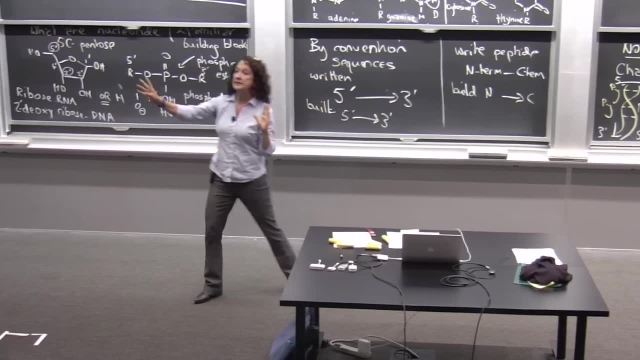 So what we've done now is we understand the structure of DNA, the non-covalent and covalent structure of DNA. We understand it's anti-parallel. What we'll do in the next class is show how you can peel apart those anti-parallel structures. 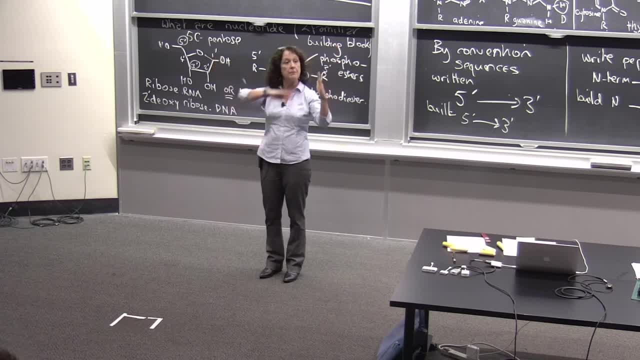 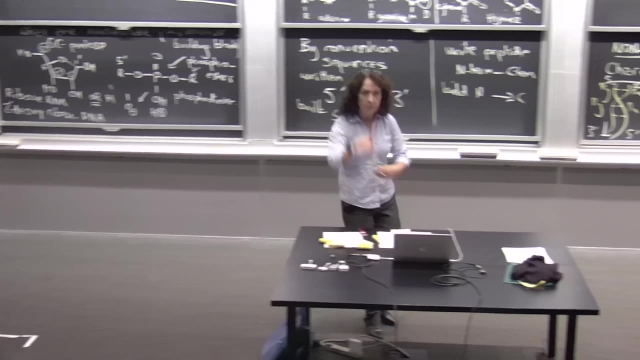 to make unpaired structures And you can use each of them as the template for the synthesis of a new strand of DNA. so you can get two daughter double strands from a single parent double strand. And that all comes from understanding the structure. Now what I want to do is move you just very briefly to the structure of RNA and comparing. 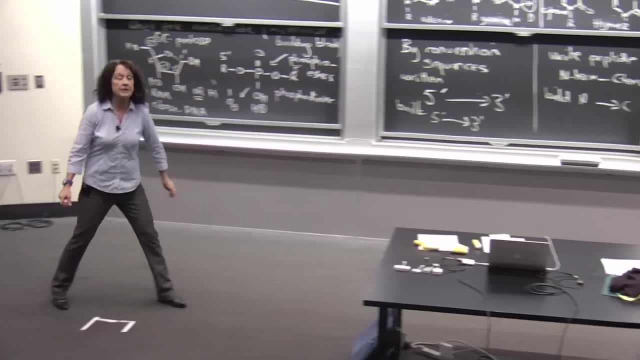 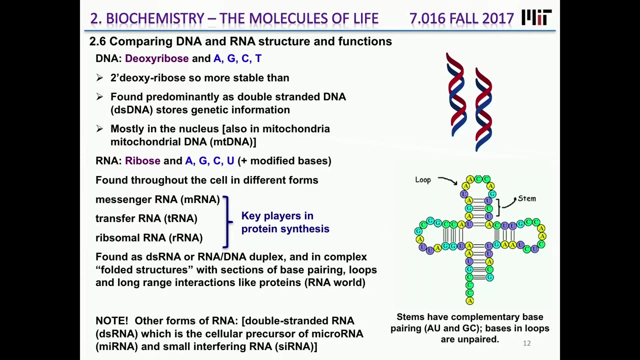 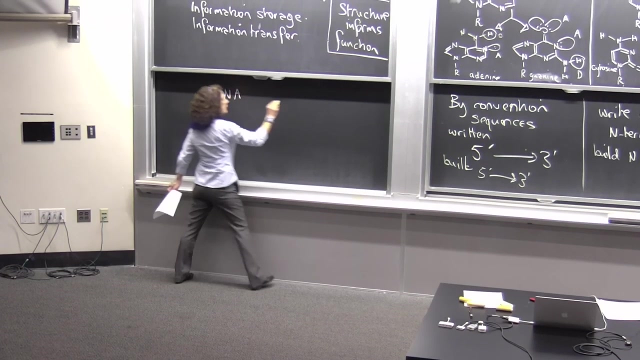 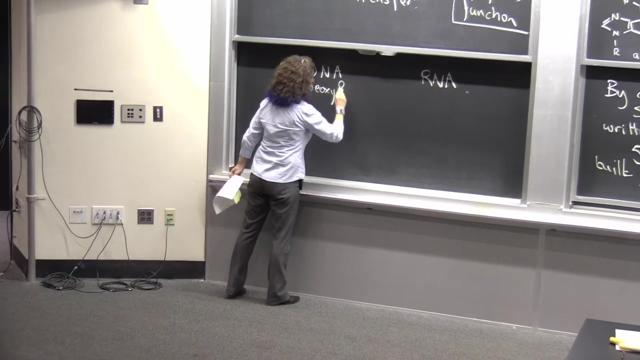 the DNA and RNA structures, because there are some differences. So let's just work through what the differences are. I have this written down And the differences are very important for the functional properties. So DNA, RNA, first of all, obviously, deoxy, ribose, ribose. 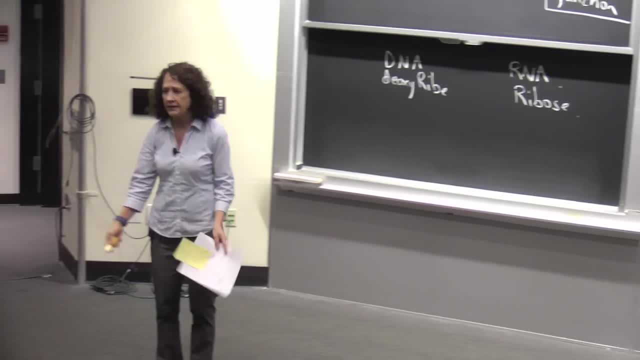 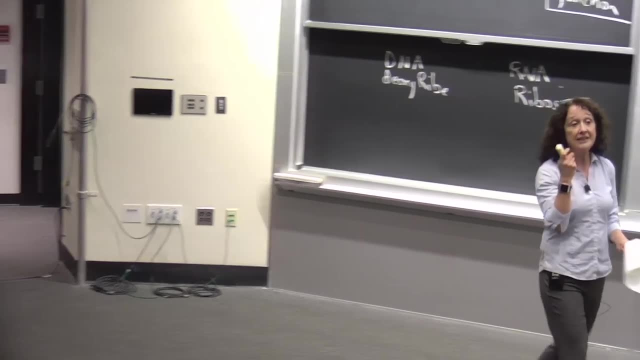 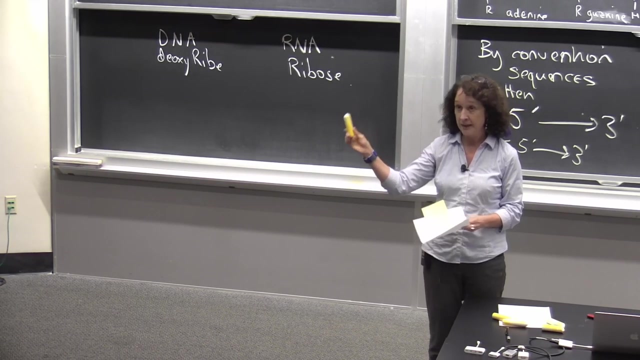 And you may go. why, Why, Why, Why, Why, Why, Why it's so complicated. Why do I have this extra factoid to remember about RNA versus DNA? And it's really amazing that the difference between having that hydroxyl on the two prime 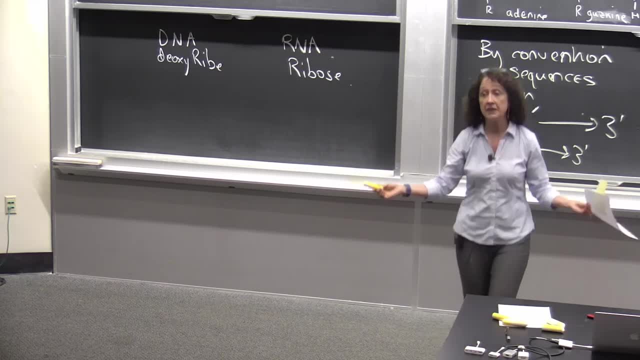 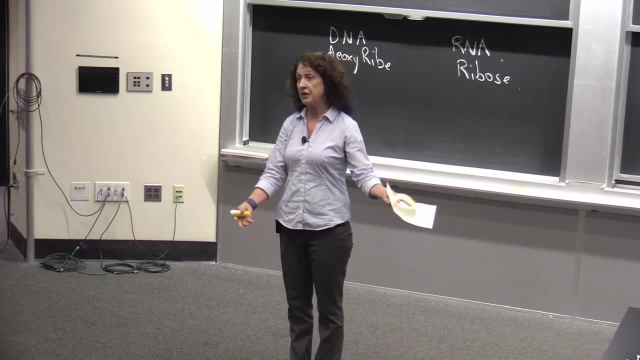 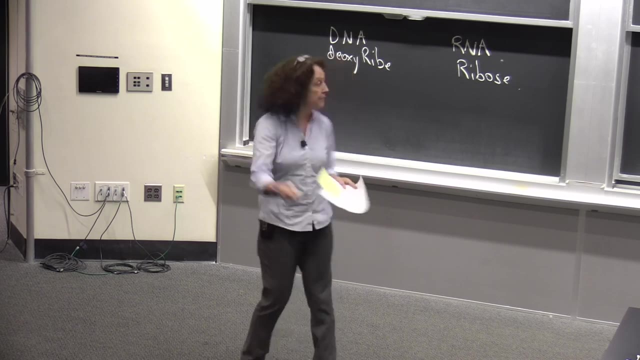 position versus not happening. not having it makes enormous differences to the stability of the polymer. RNAs break down very, very readily. DNAs are stable for the lifetime of a cell chondria. they stay intact. So there's a stability difference. 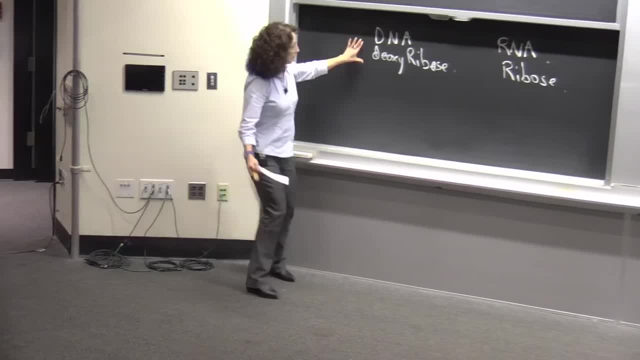 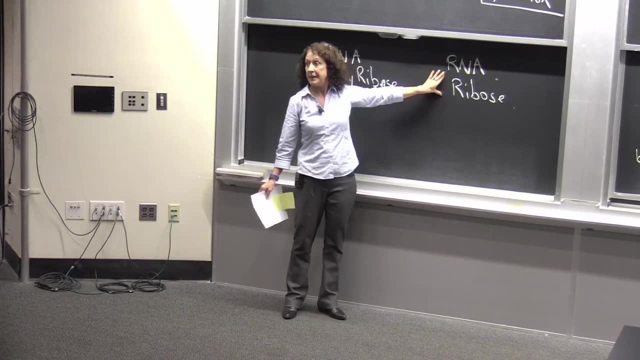 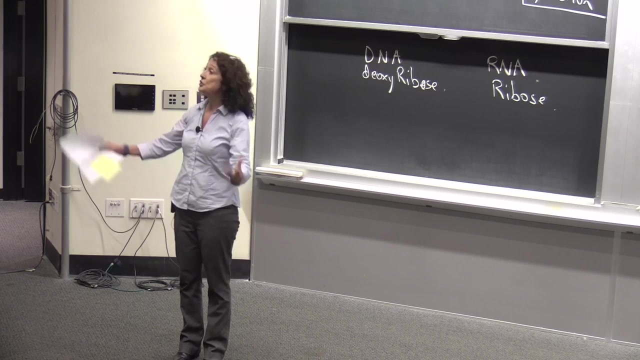 between the two sugars, because DNA has to be the place where you store your genetic material. It's got to stay good, Whereas RNA is the message that you make transiently to program a protein being made and then you want to get rid of it. 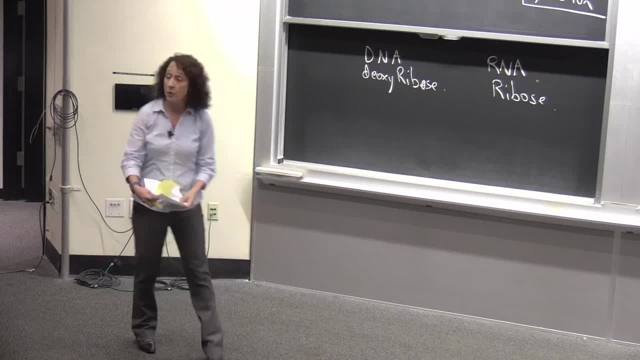 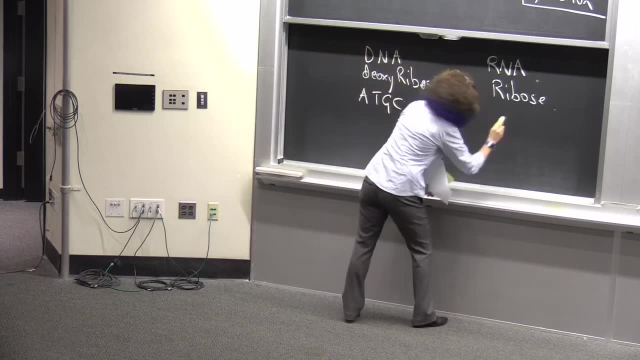 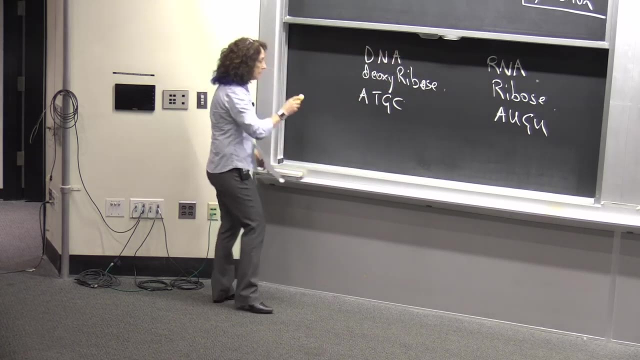 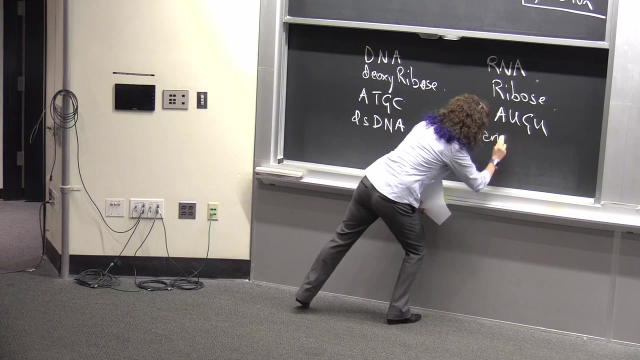 So we need the differences in stability that originate from that small feature. A T G C. there's the difference A U G C in the bases. The most common DNA is double-stranded DNA, whereas RNA forms various structures. 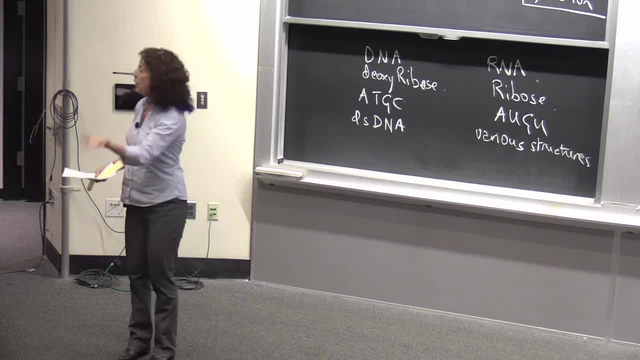 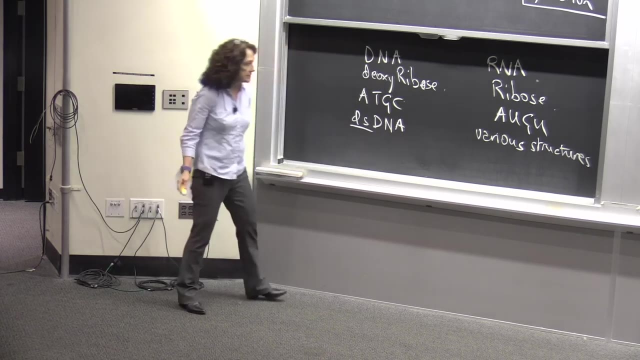 So it's much more irregular. It's more irregular structures than the DNA, probably in part because the ribose is substituted differently, So that continuous strand of double-stranded material is not quite so stable. in RNA We find DNA principally as double-stranded DNA. 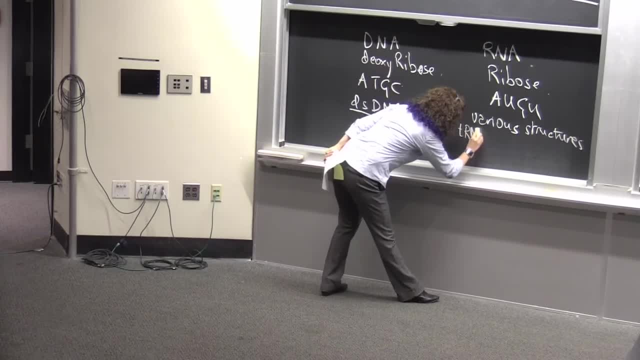 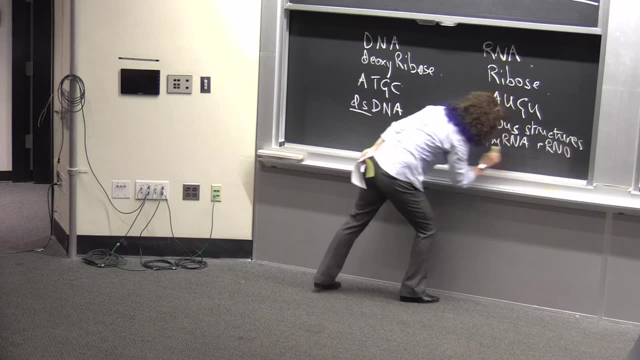 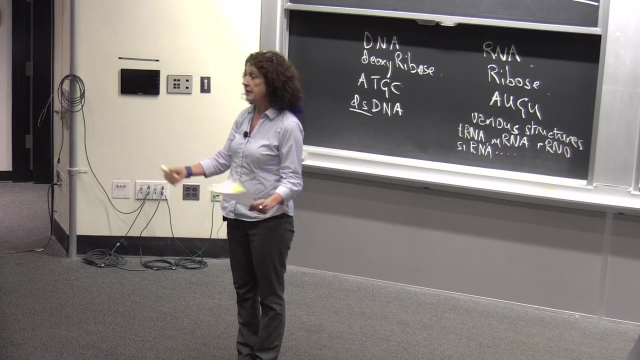 but RNA we find as transfer RNA, messenger RNA, ribosomal RNA. It does go on forever. It's short-interfering RNA. So the various RNA is used for a lot of purposes, whereas DNA principally stays as the double-stranded DNA. 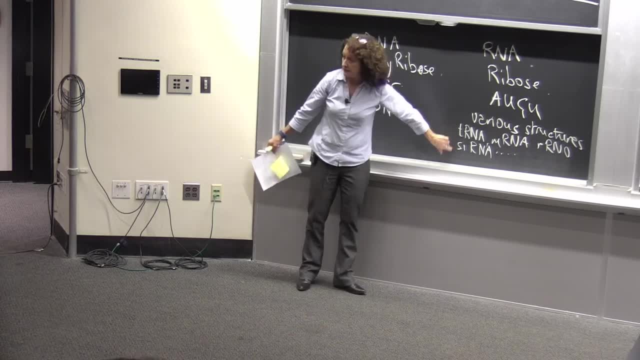 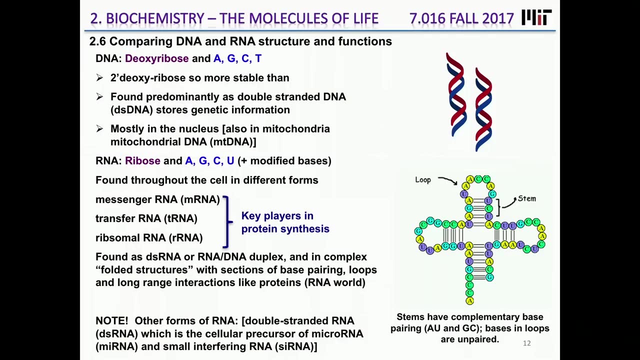 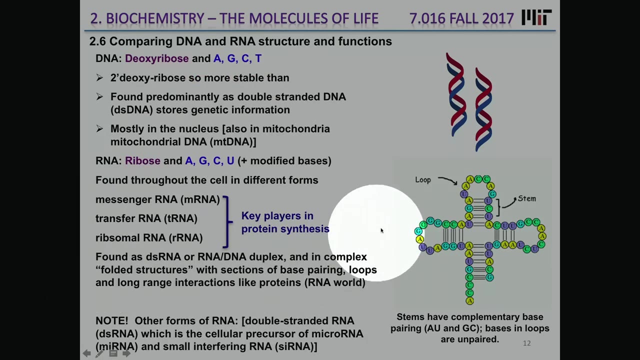 There's a little double-stranded RNA, but it is a precursor to some of these other forms of RNA. So this slide just summarizes some of that for you- the differences comparing DNA and RNA, And so what we'll see later It's how RNA lends itself to these interesting structures. 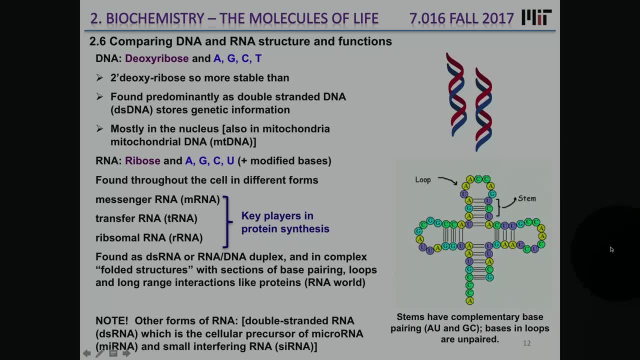 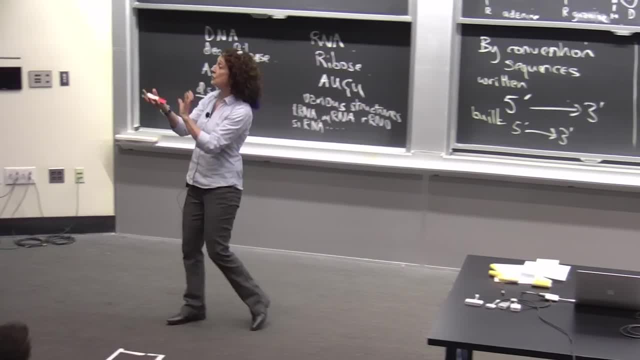 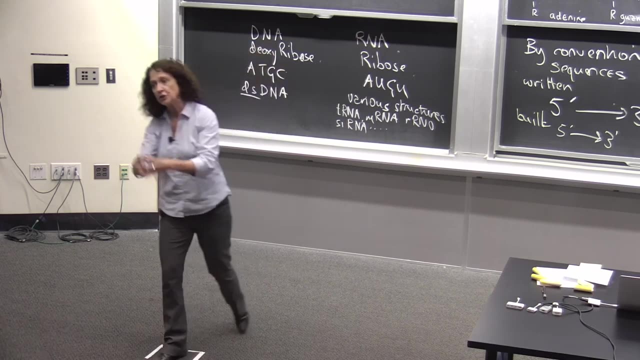 where you still have some base pairing but you have a lot of loops and turns and diversity of structure. And that's really kind of the origin of this RNA world, where RNA structures could have variety of form that might contribute to different functions beyond, just as a message, as a place to store a DNA message. 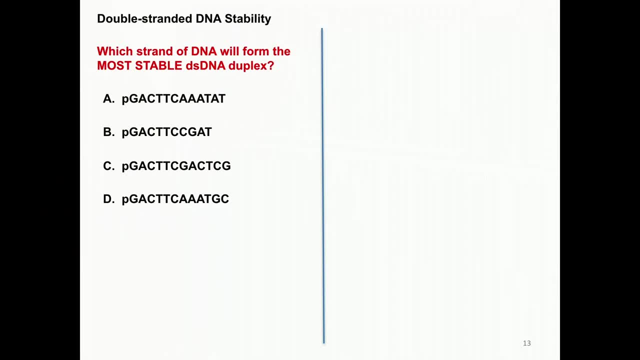 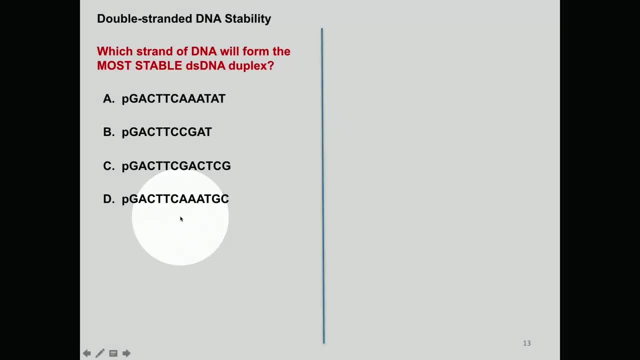 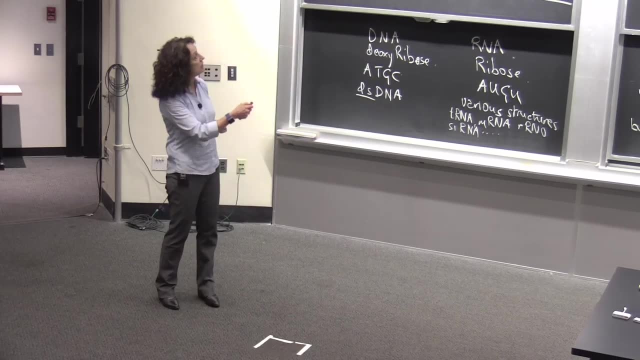 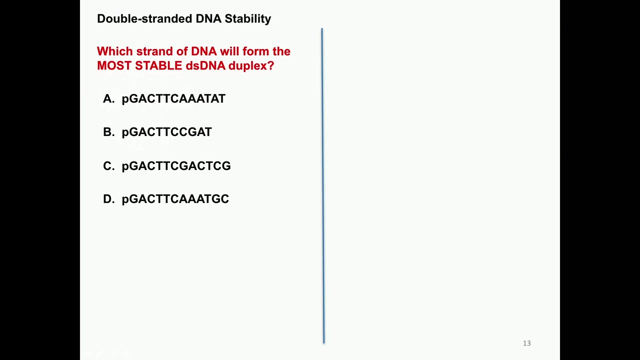 So can you guys guess which of these strands would have a complementary strand and be the most stable double-stranded DNA? So this would be one strand. You could draw for each of them its complementary strand. Can you guess the clues to figuring out which would have a most stable organization? 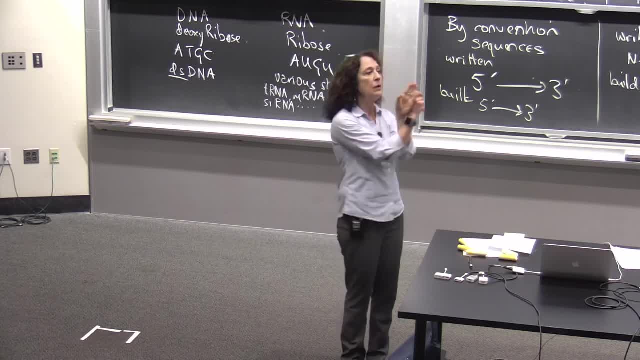 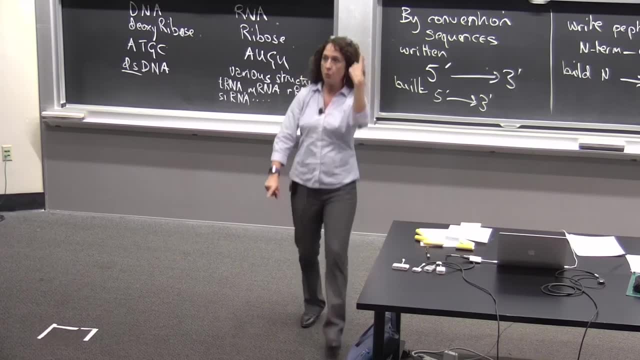 of the anti-parallel double-stranded DNA. What would I be looking for? Can you guess? the clues to figuring out which would have a most stable double-stranded DNA. Okay, so number one: higher GC content, because Gs and Cs form three hydrogen bonds. 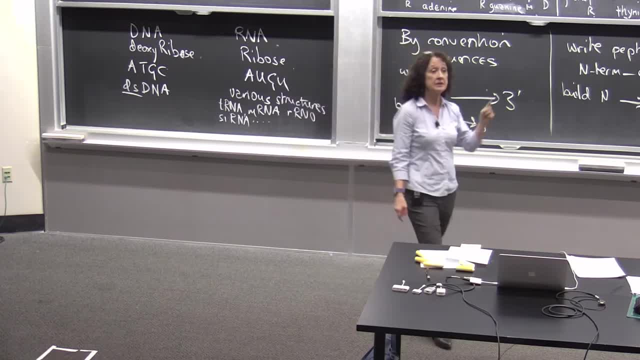 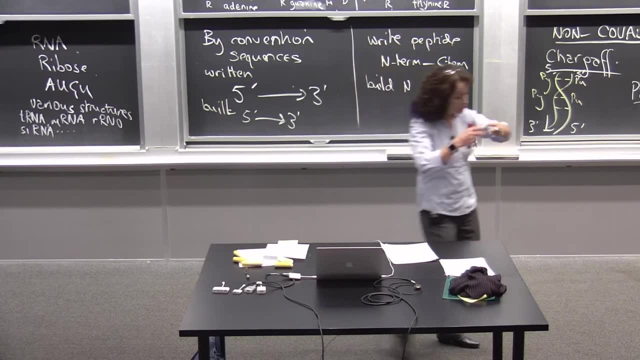 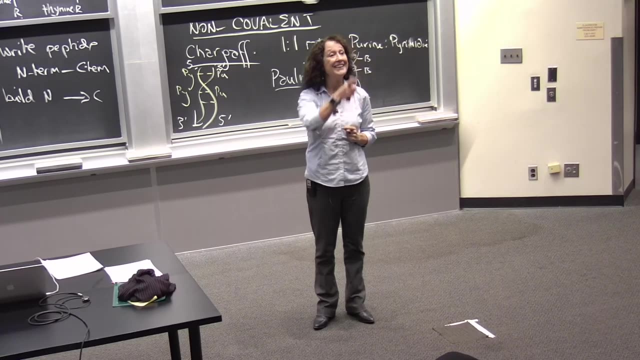 As and Ts only form two. And what's the other determinant? Just looking at those structures. Yeah, Yeah, you are doing. no, it's actually even more silly. It's more simple than that. Okay, length. so all you do is you go along. 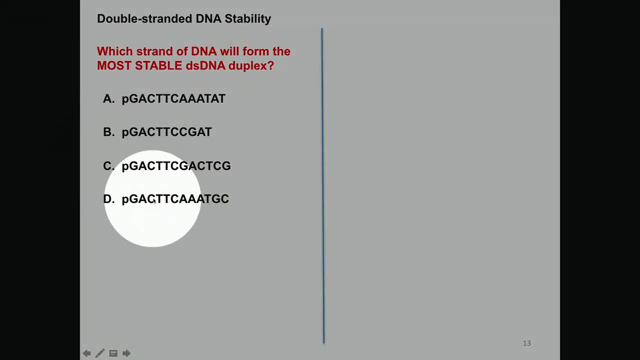 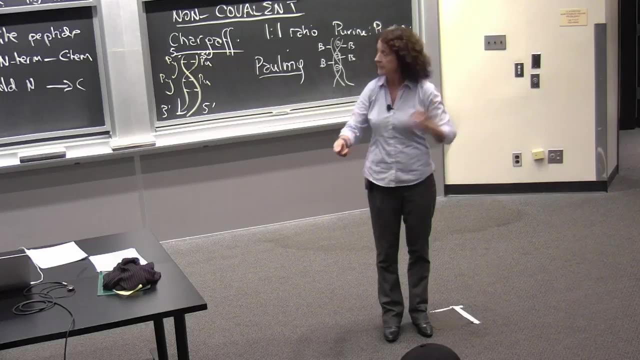 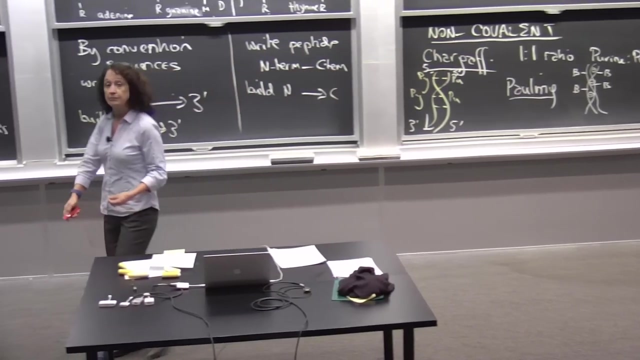 and say: I can make three hydrogen bonds: two, three, two, two, three, two, two, two. So you truly just count hydrogen bonds in its partner sequence and you can guess which is going to be the more stable, because it has the most hydrogen bonds. okay, 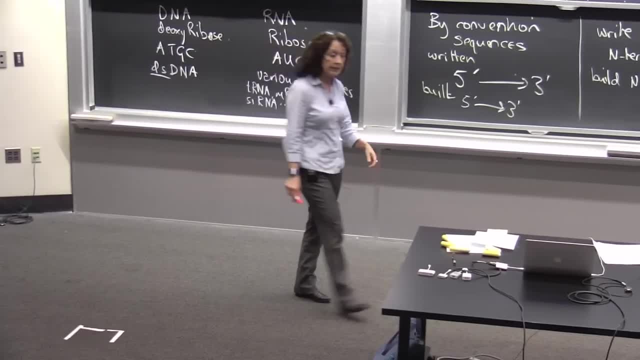 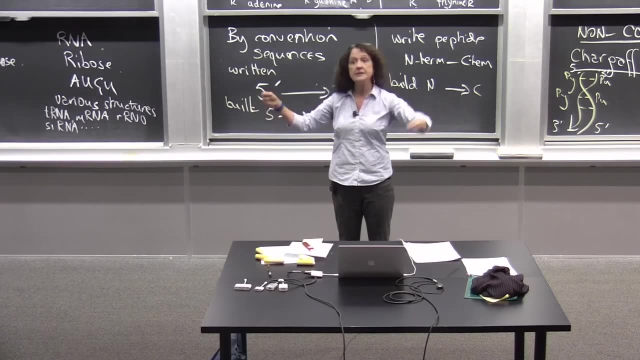 So we might ask you that which one will come apart? Now, the intriguing thing about DNA is: you can peel it, you can heat it and it'll come apart, But it doesn't denature the way proteins do. If you just cool it down, it comes back together. 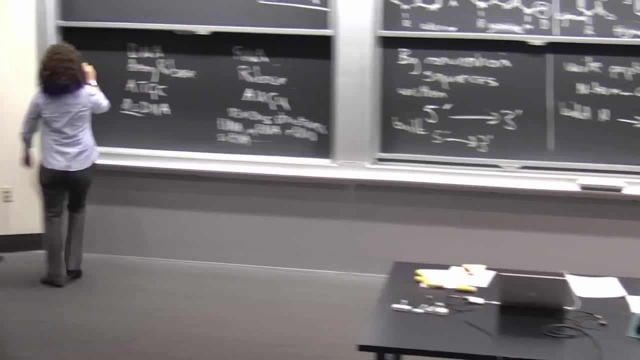 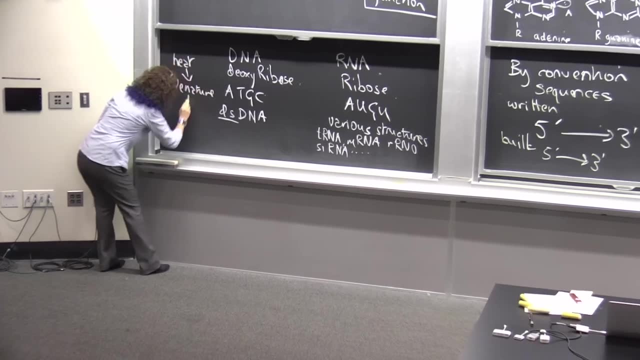 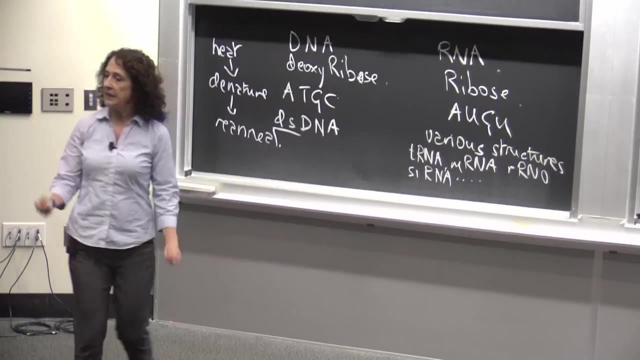 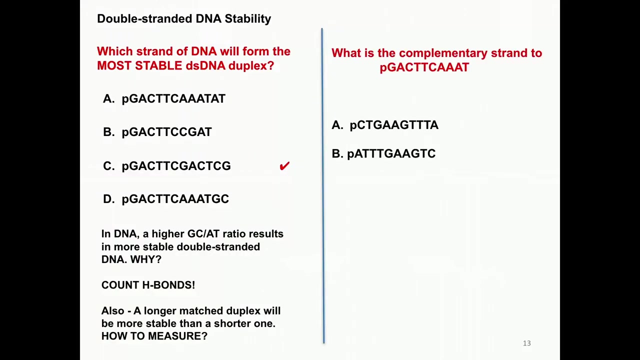 So another feature of DNA is that you can heat, denature and then reanneal Exactly how it was in the first place. It doesn't denature to something that's not very useful. And now the question: can you draw the complementary strand? 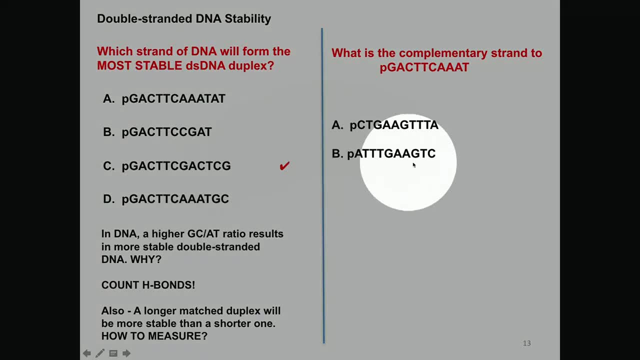 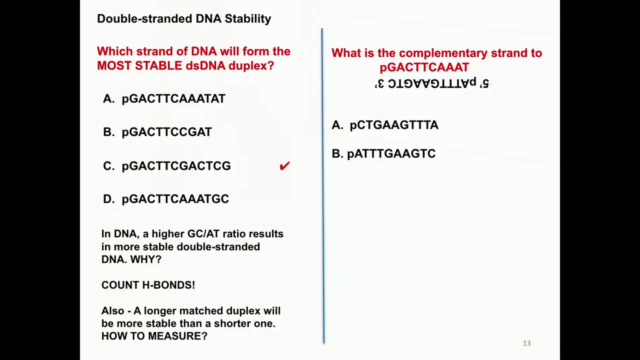 I always find if this top strand here, which of these is the complementary strand? Frankly, the best way to do it is to sketch out the complementary strand. You can see it kind of upside down, because it's really hard to draw things. five prime. 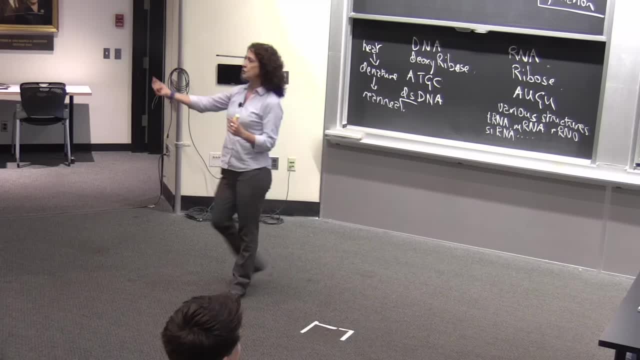 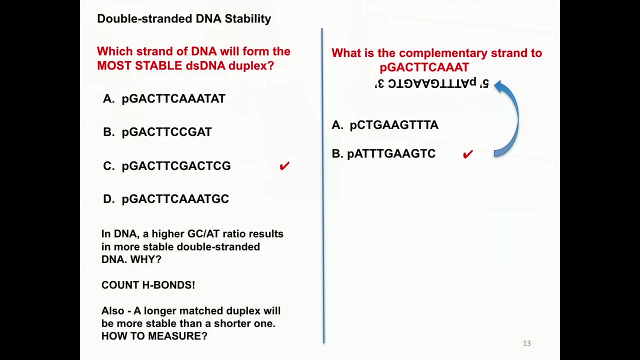 to three prime when you're also trying to figure out base pairing. So draw it upside down, Make sure you know the five prime and the three prime end, and then you can guess the right one. And that's the right answer for these types of questions. 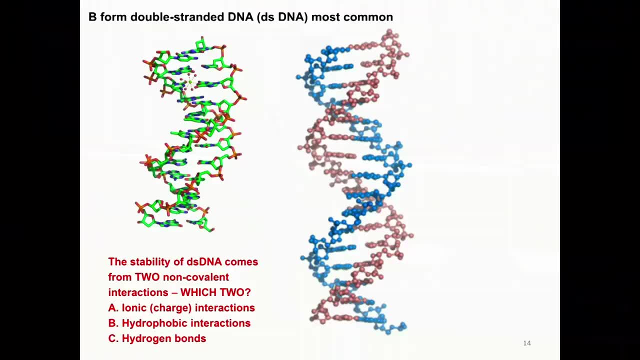 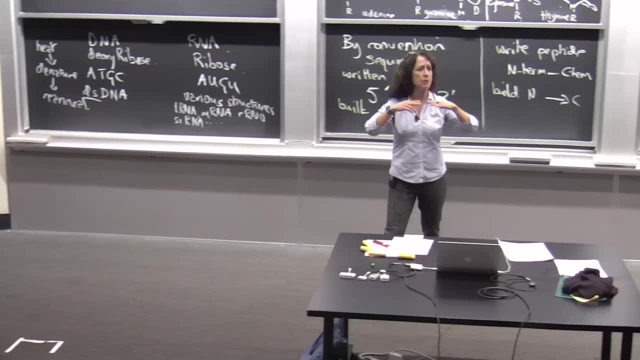 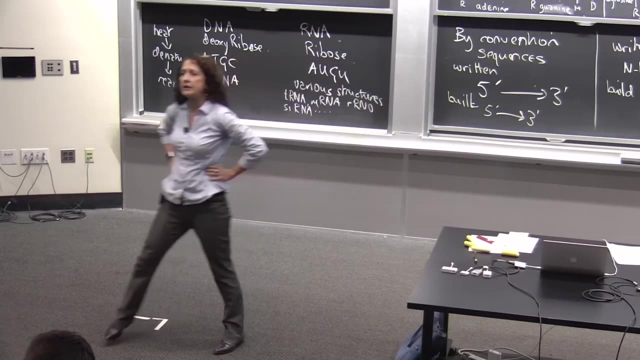 about complementary strands. Now one last question: The stability of double-stranded DNA. I've made a whole big deal about hydrogen bonding, right, That's what holds it together. What other forces could be at play in double-stranded DNA that might contribute to its stability? 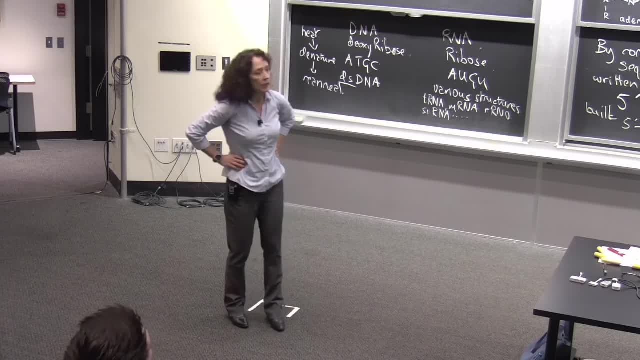 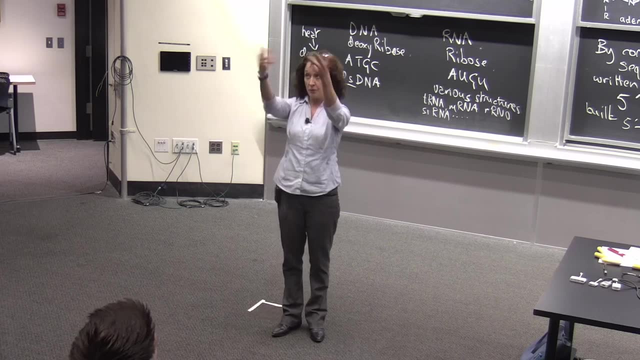 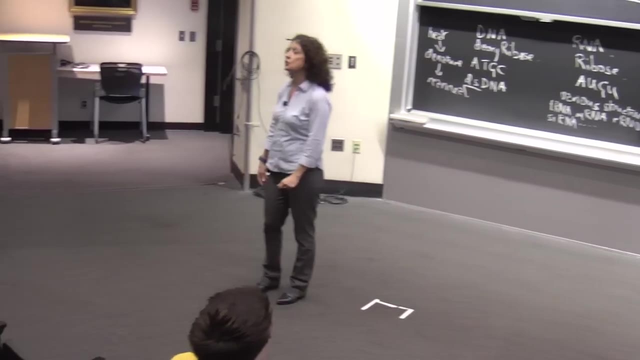 Any thoughts? What else? Well, it certainly doesn't look like it's charged because the predominant charge is negative. This is not an opportunity. You've probably got metal ions there, kind of neutralizing that charge. What would be the other force and how would I describe it? 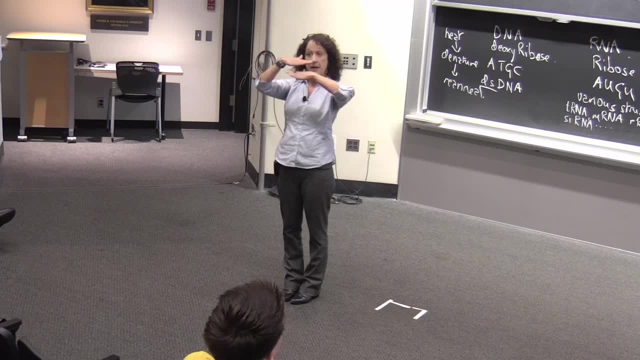 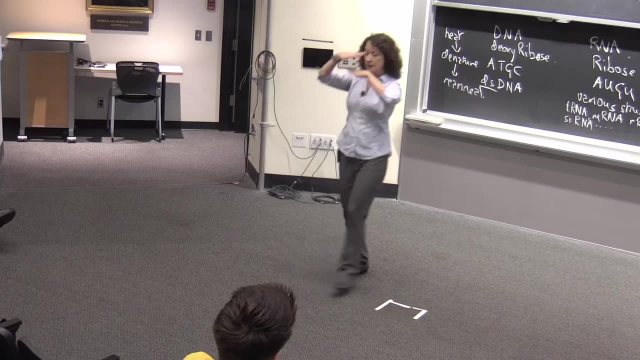 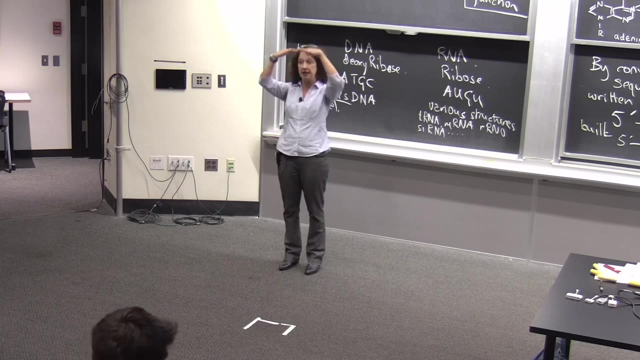 It's a tricky one. So we've got these bases and they're pretty hydrophobic, They're planes, They have electron density on both sides. So it turns out there is some stability gained between the packing of the steps of DNA, between each base pair with the next, with the next. So there are hydrophobic forces, And researchers at Scripps have actually proved this paradigm by making extra DNA bases that don't have hydrogen bonding partnerships but just provide the stuff, that's, the flat hydrophobic entity with the right size that can slip into DNA sequences and make stable adducts. 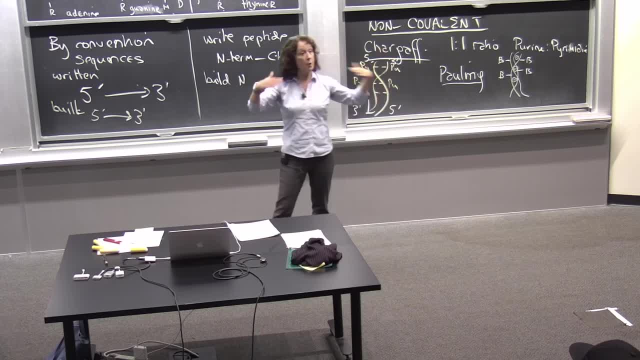 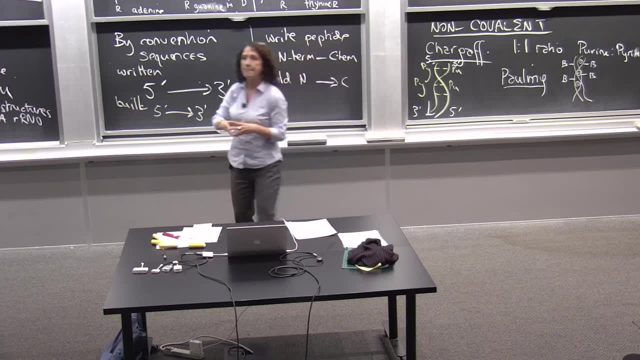 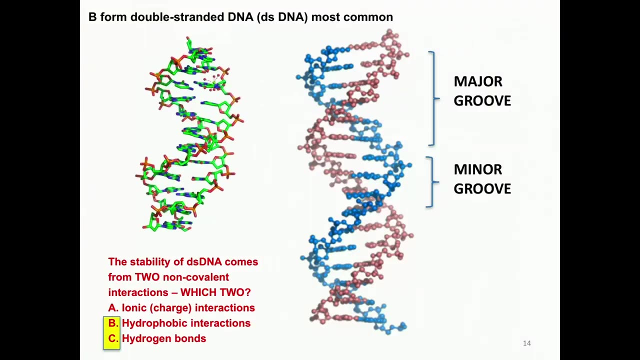 It makes stable, not really base pairs anymore, but just be stable in that polymeric structure. Are people understanding and following that? OK, So finally, when we look at the structure of DNA, there are some trenches where things can bind to. proteins can bind. 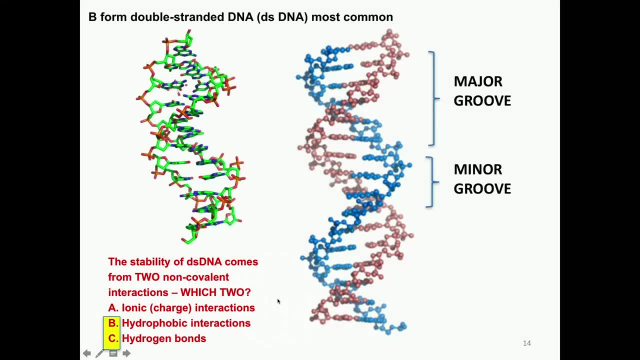 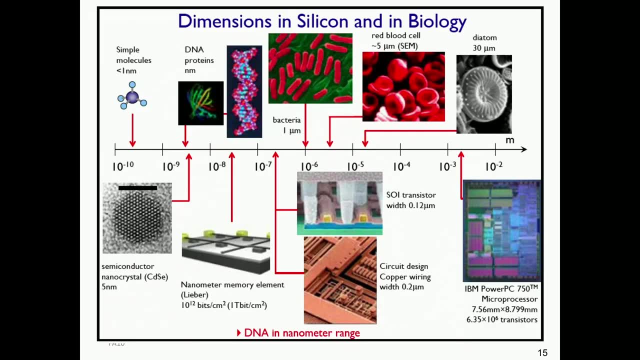 And we talk about the major groove and the minor groove, But I will talk about those later on, when we talk about transcription factors. Now I just want to, in really triple-passed time, and I'll put this on the website: there's tremendous interest in using the building blocks of DNA. 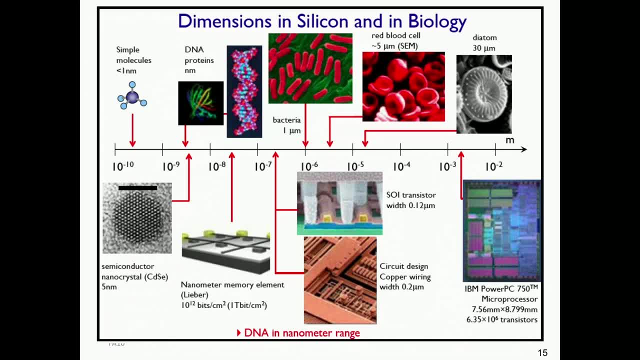 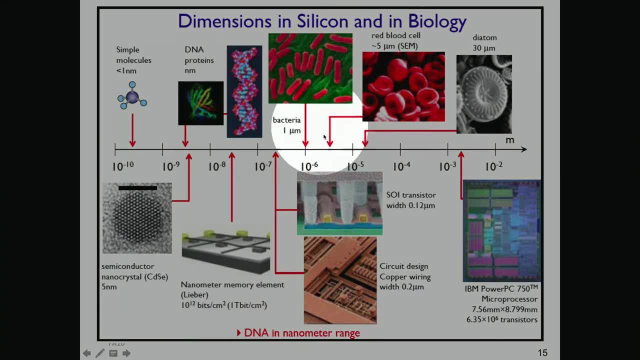 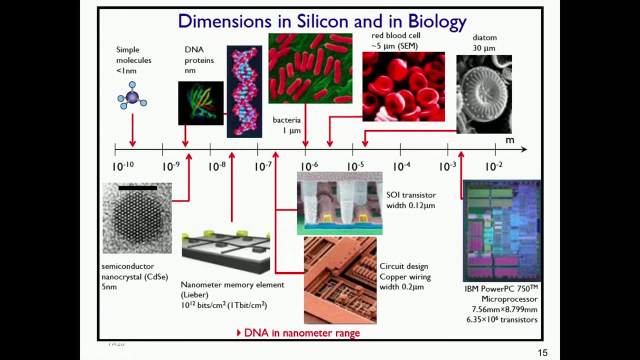 for information storage in computing. So if you look up DNA-based computing on Wikipedia, you'll learn a whole lot about it, Because what's so exciting about it is it's an organized nanoscale material that can be programmed to base, pair and form. 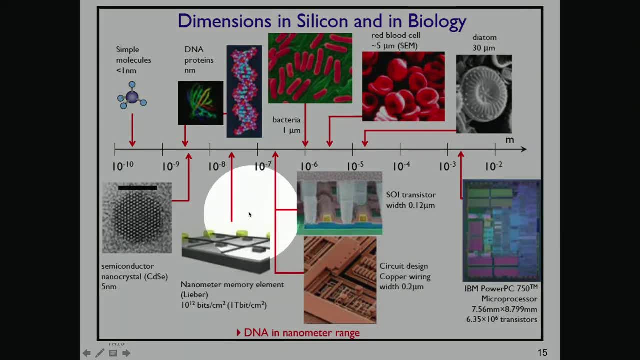 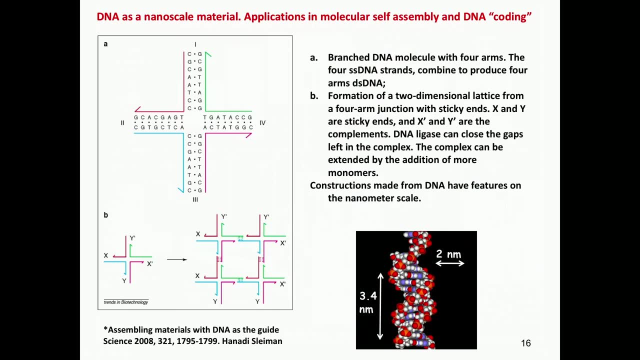 certain structures. So in the sort of range of different structures it's very interesting. It's very different sizes. There's been a lot of interest in DNA as a material for information storage, not for your genetic material, but for plain old information. 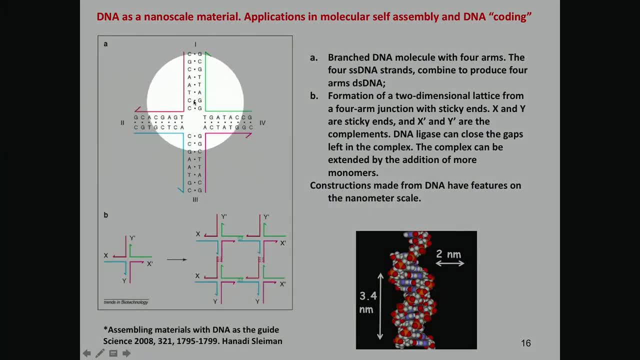 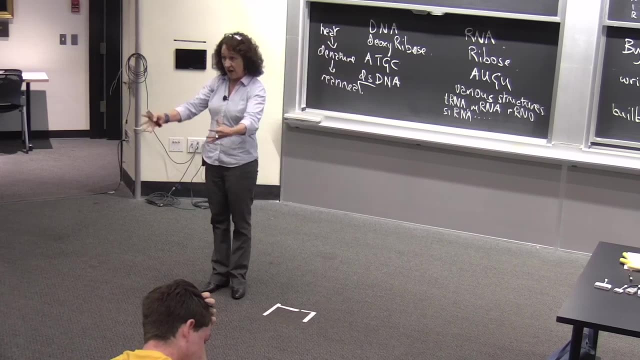 storage. So people have learned how to build structures of DNA where they can construct these sort of cruciform structures by base pairing. They can make the arms of these structures a little bit extended So you could start joining those things together to make very defined three-dimensional entities.